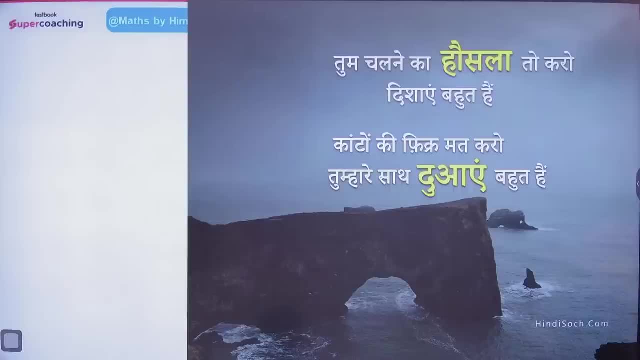 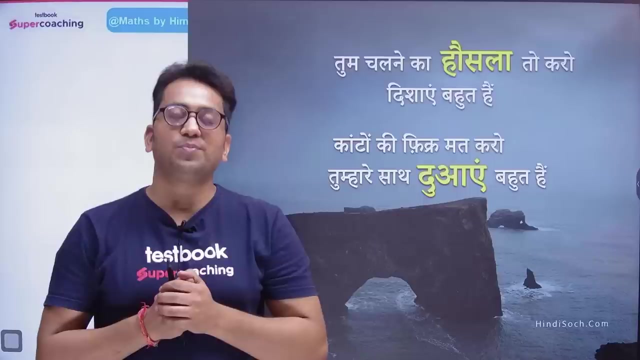 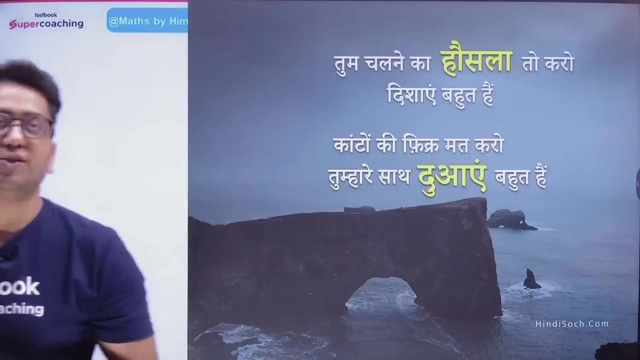 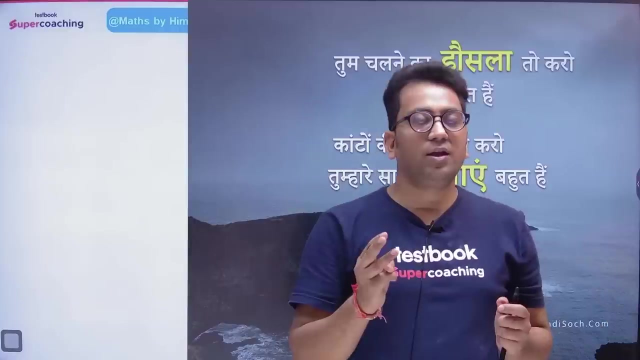 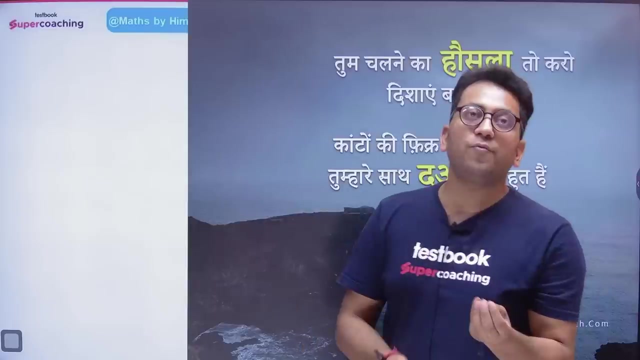 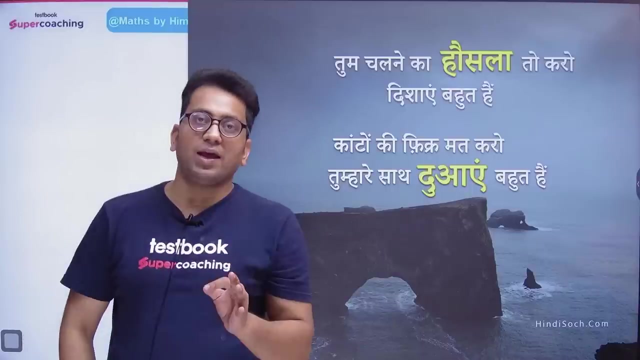 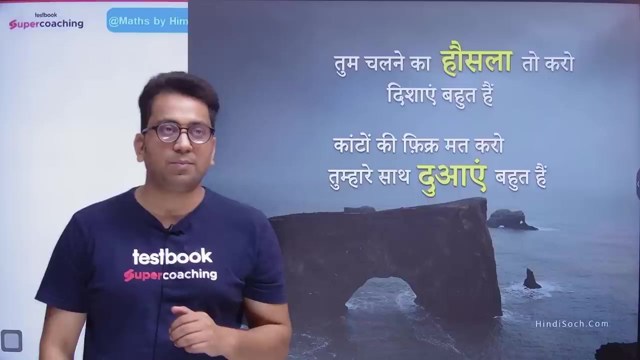 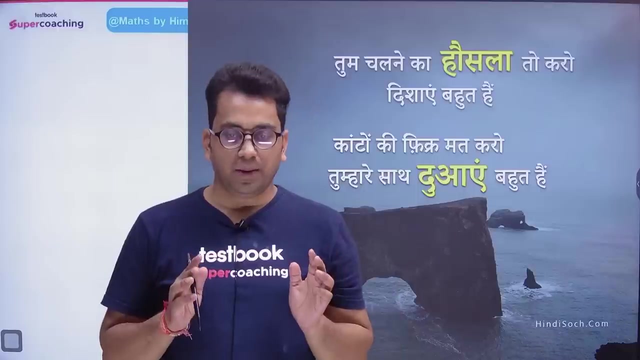 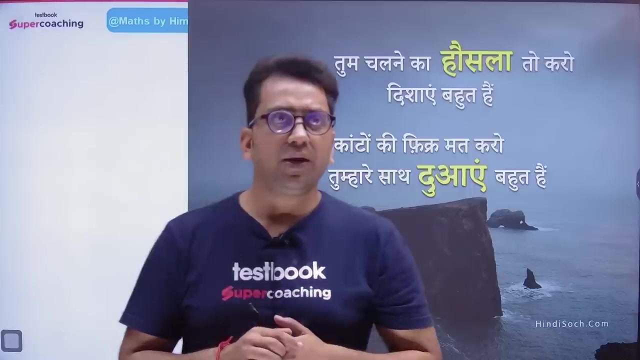 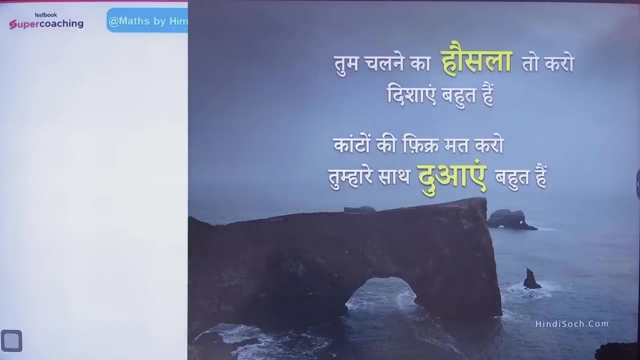 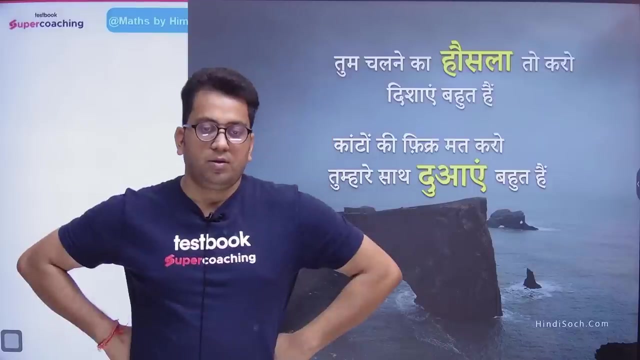 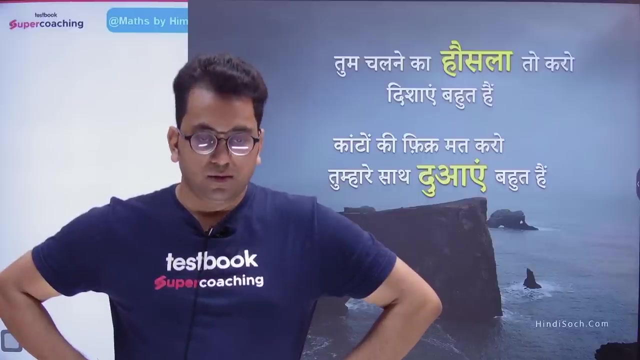 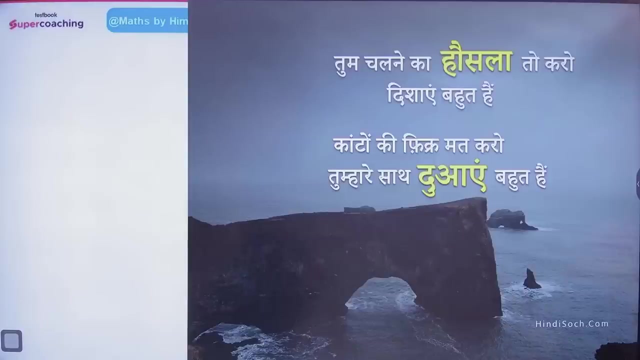 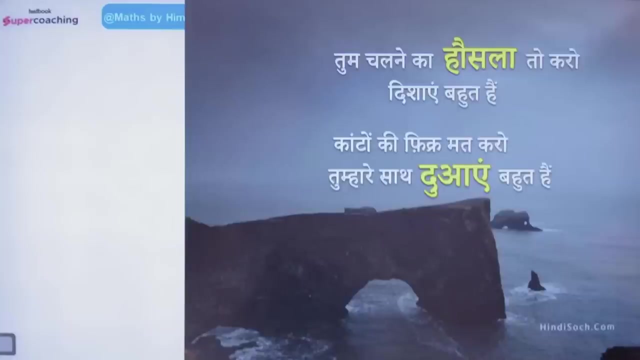 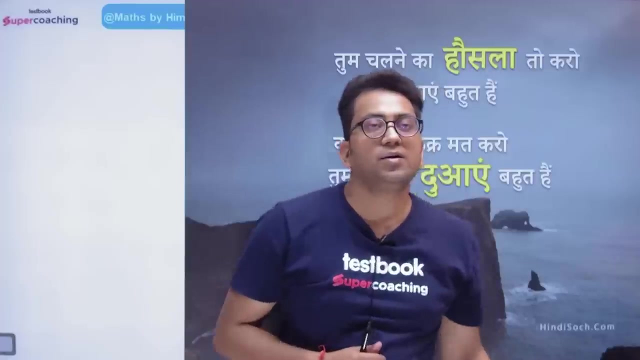 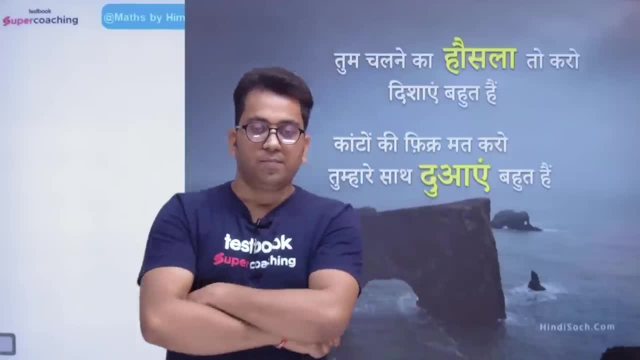 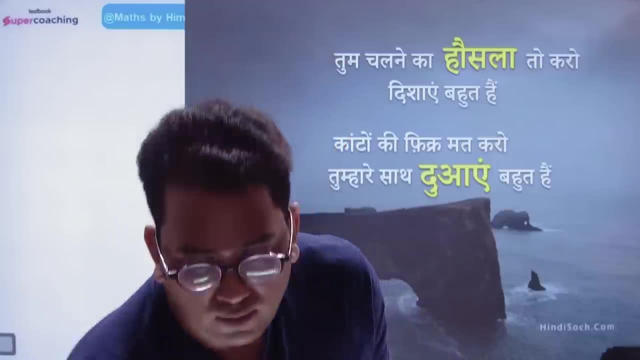 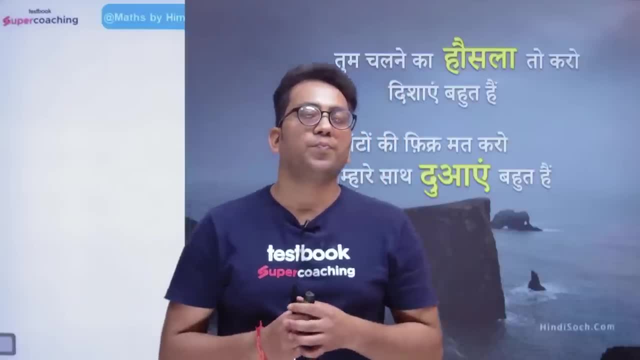 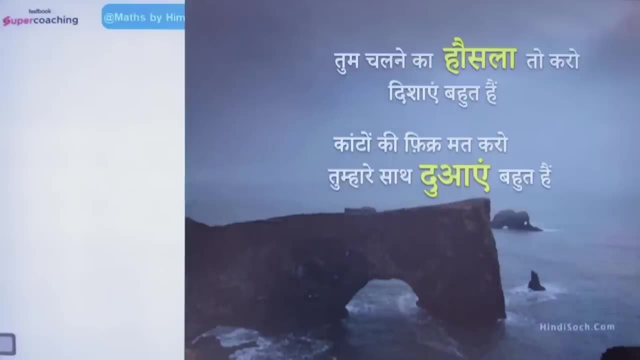 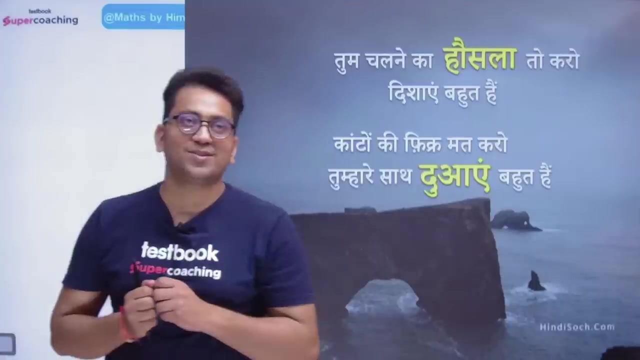 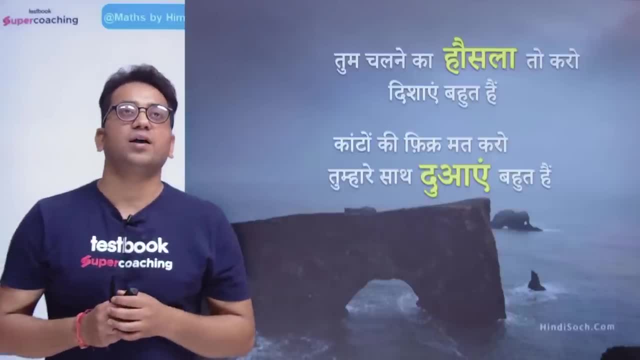 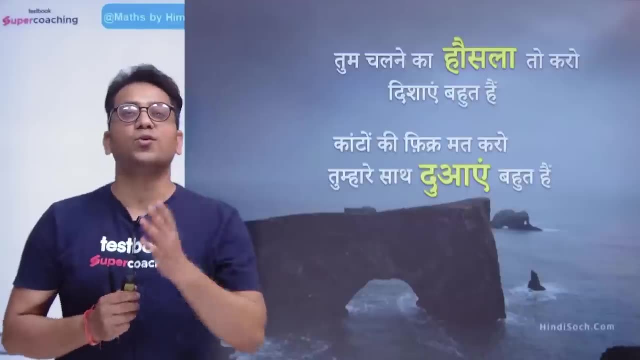 Everyone is ready, ready, So we will start with these excellent lines. You have to have the courage to walk. There are many directions. You have to have the courage to walk. There are many directions. Don't worry about thorns with you. 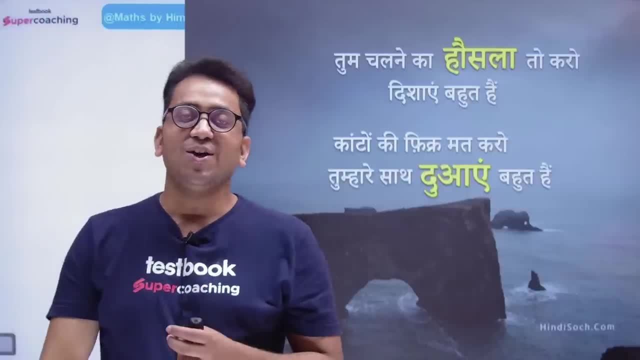 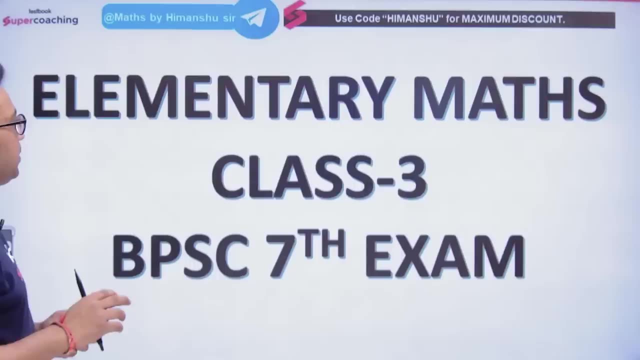 There are many blessings of your parents. Okay, so let's start our session today, Okay, Okay, In this session, what we are going to see, there are going to be a lot of great things. First of all, let me tell you that this is class number 3 of elementary maths. 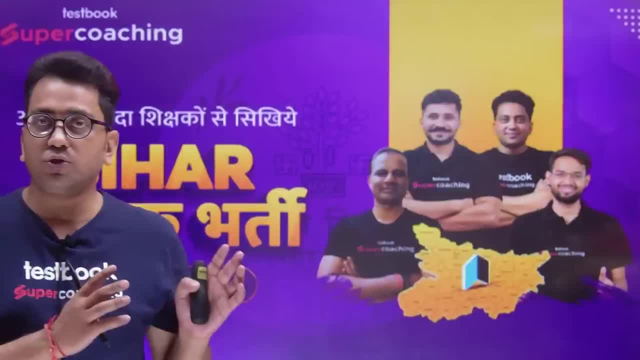 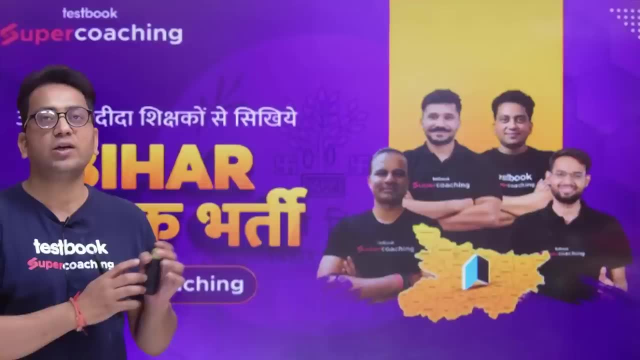 And the batch of Bihar Shikshak Bharti has come on super coaching. You can join this batch. Okay, as soon as you get a notification, a live batch will be started for you in this batch And this batch is going to be with you till exam date. 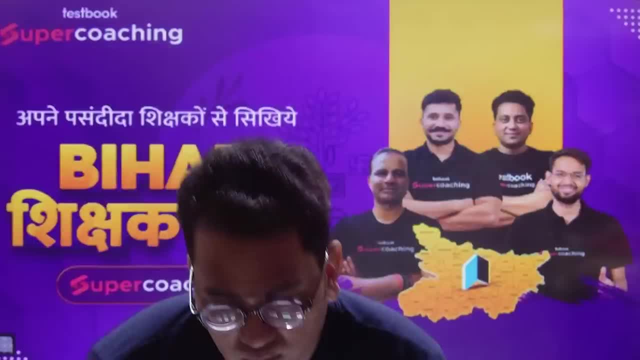 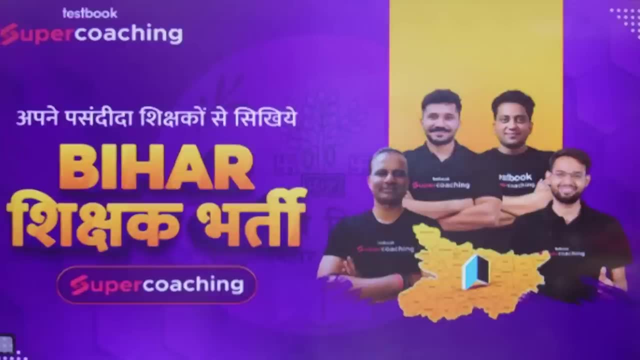 Is buffering still going on? Yes, Okay. Now do you want to know how many places this batch is? Yes, Okay, let's get started. So what we are going to do is: you are going to have to be very cognizant of this. 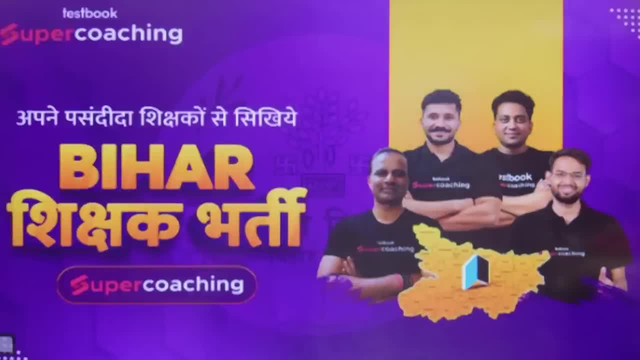 and you're going to be able to know what is going on in this batch, one by one, and you're going to be able to understand what your teacher is going to say and then what the moment that he is going to say. So here we go. 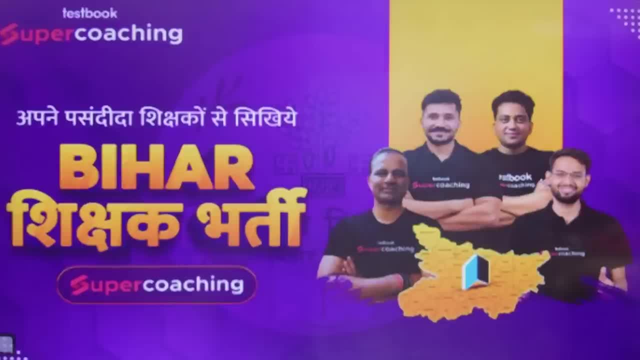 And you are going to be able to understand. okay, Here is the lesson, right, Okay, All right. So this is your first booze. Okay, let's go. Okay, good, Okay, good. Now we are going to have a little chat. 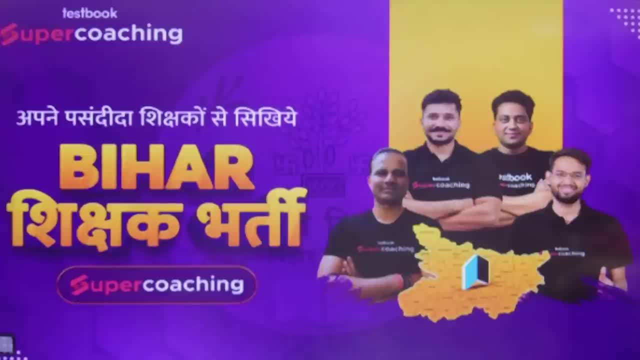 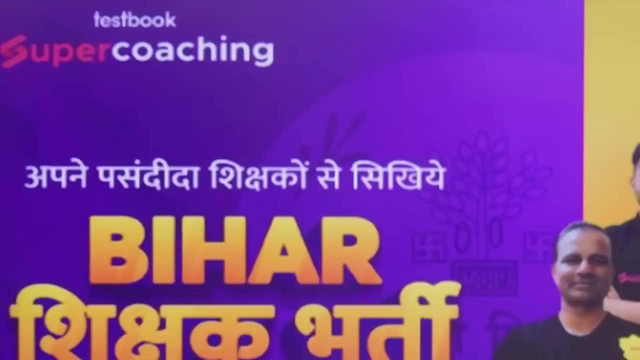 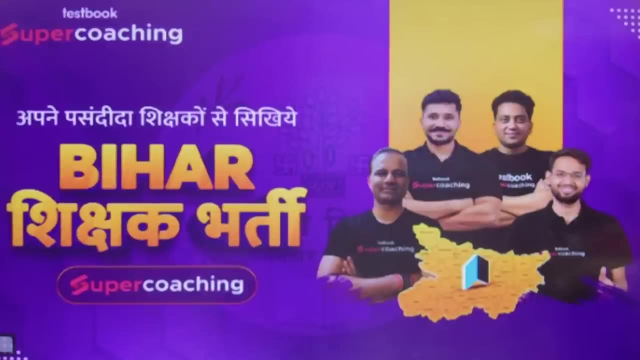 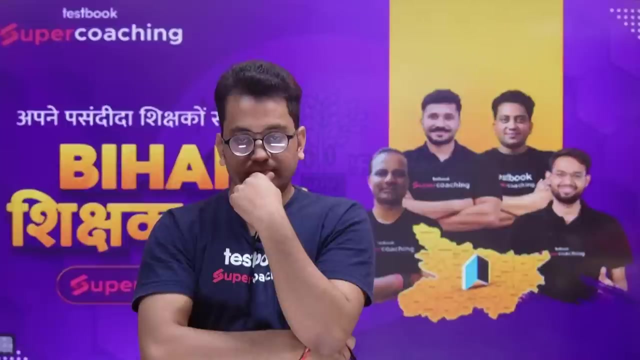 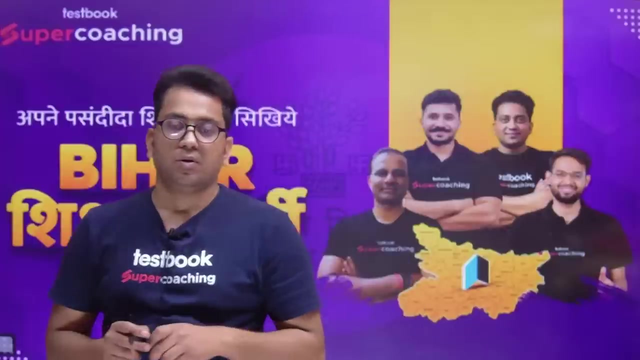 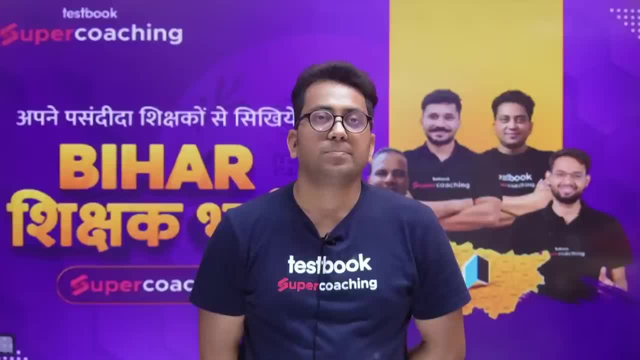 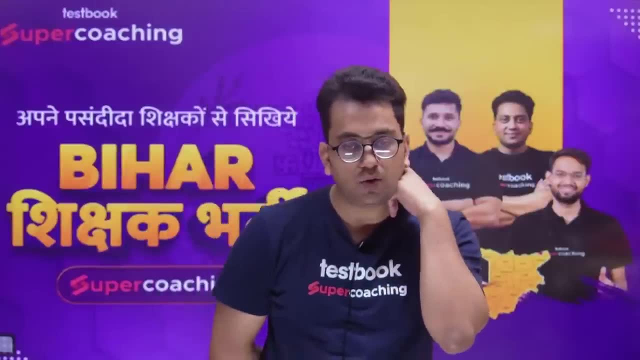 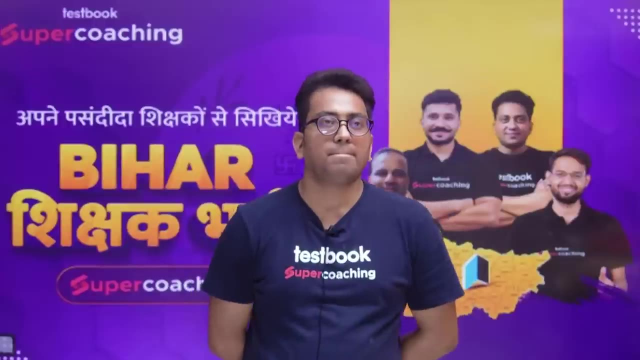 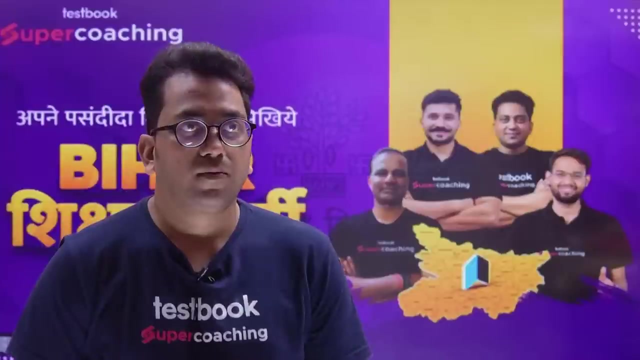 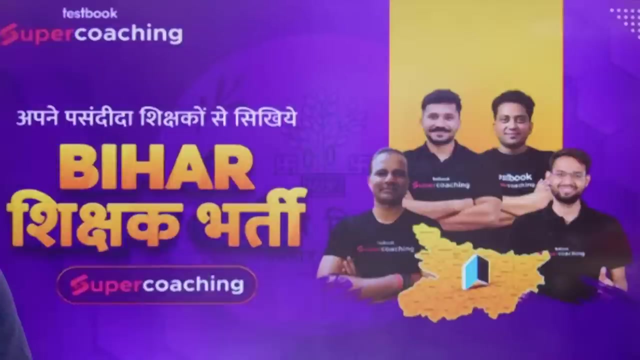 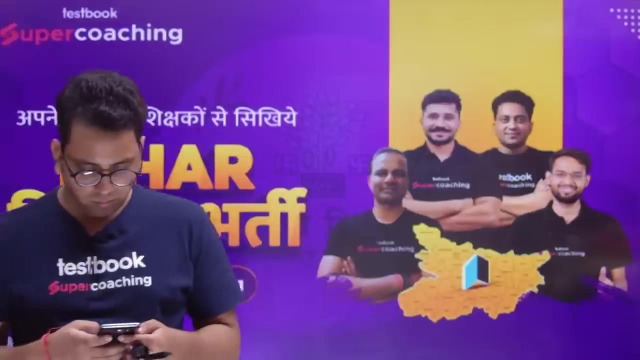 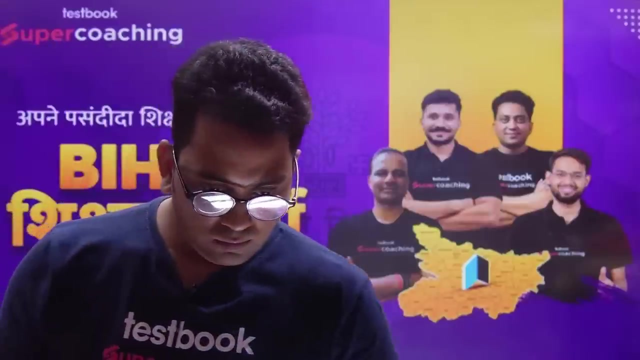 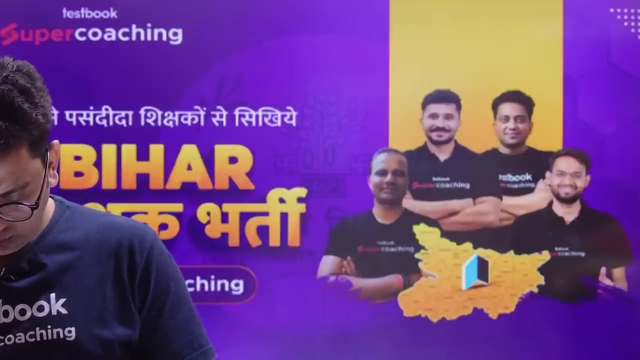 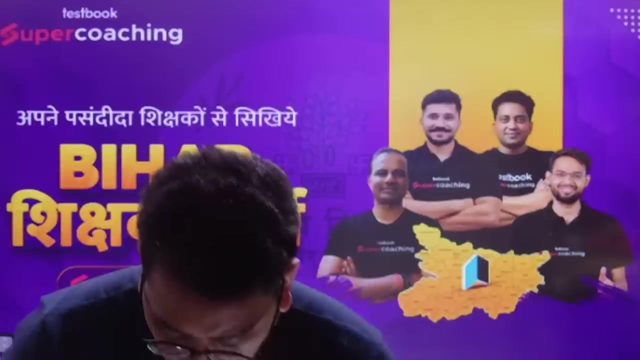 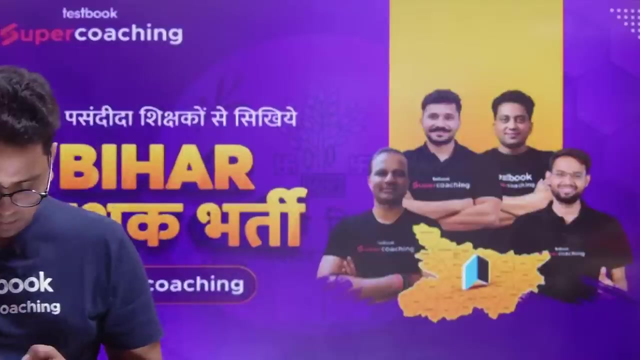 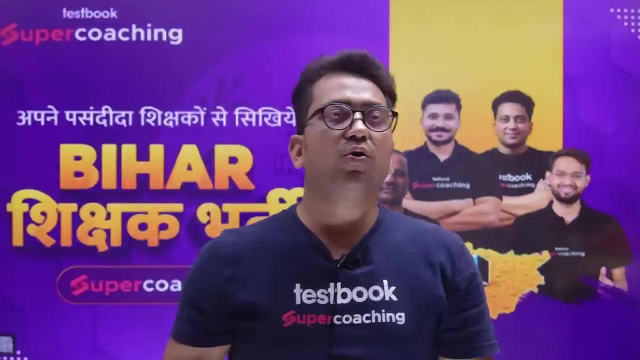 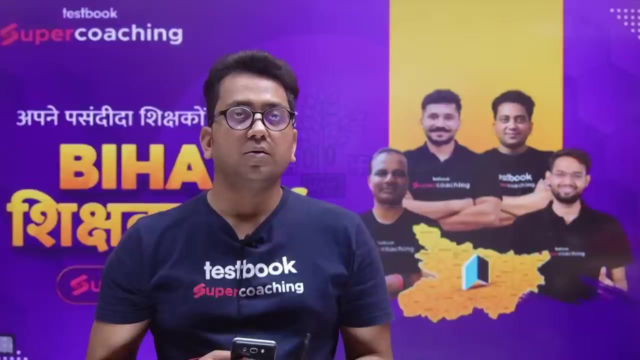 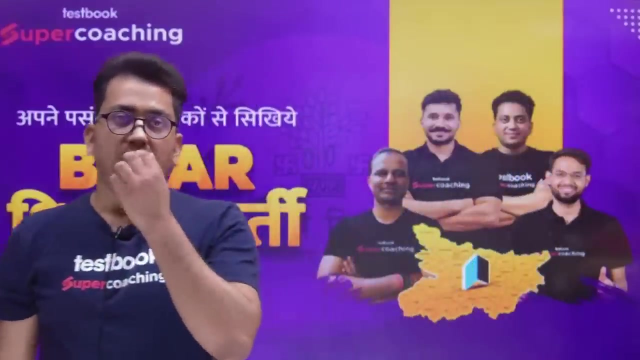 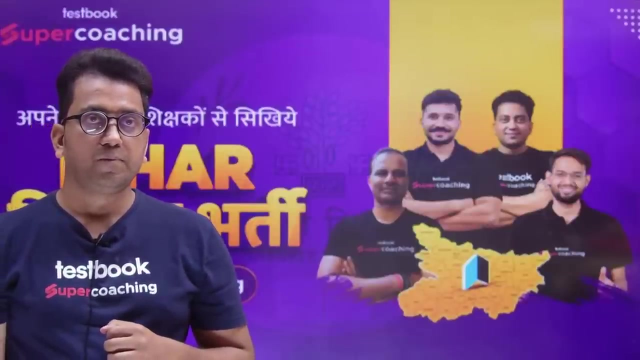 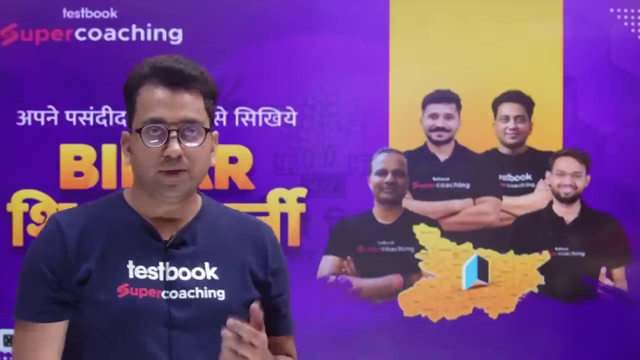 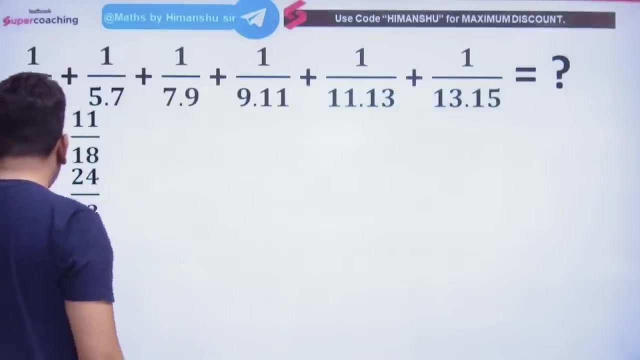 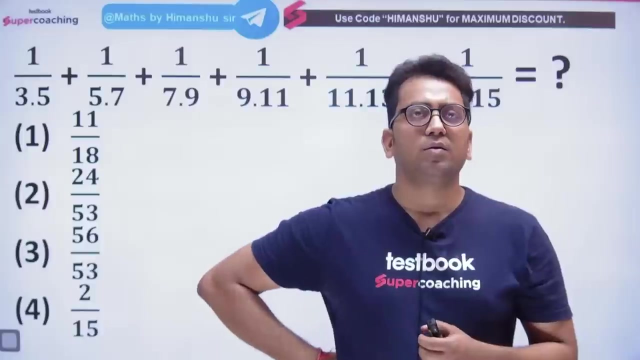 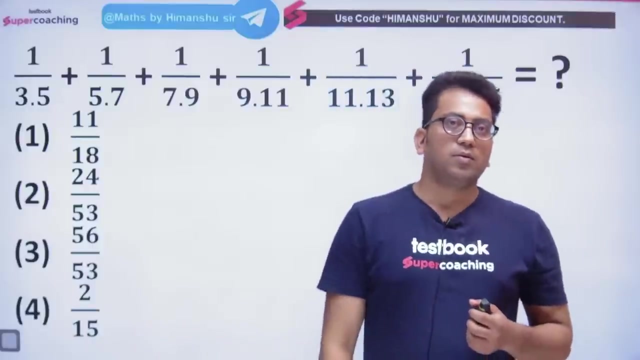 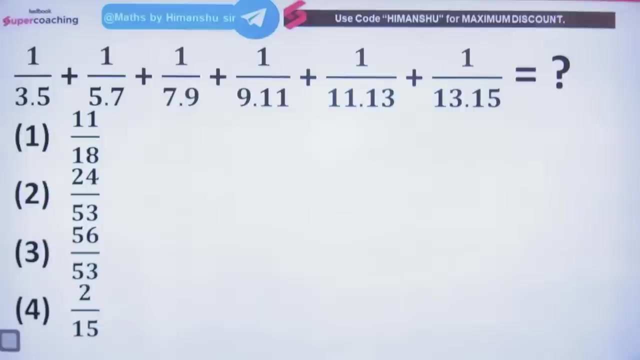 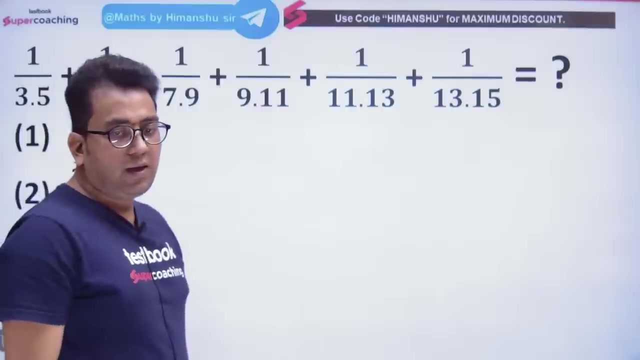 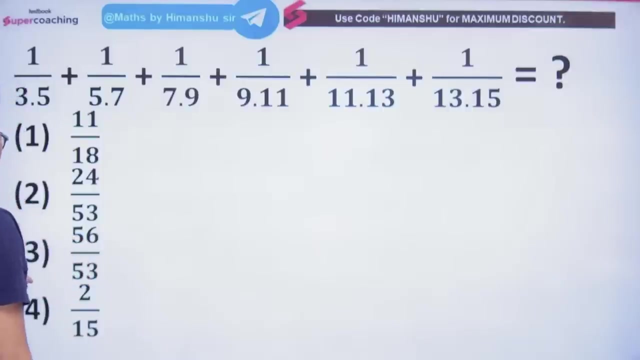 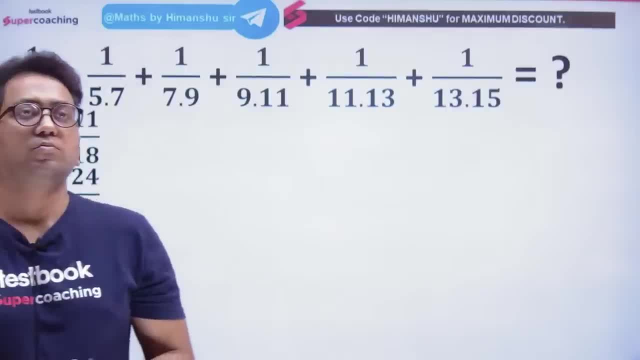 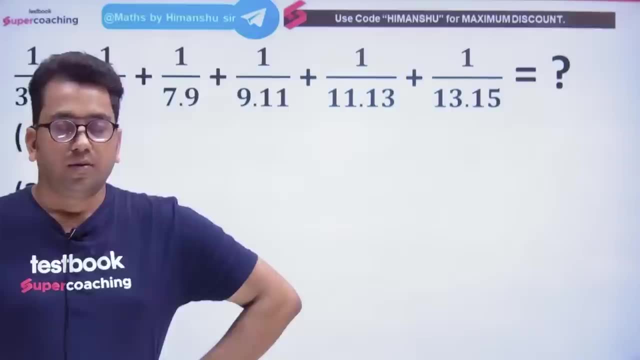 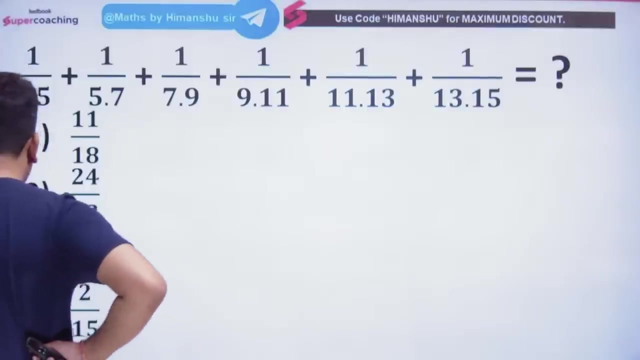 So the first question is in front of you. the first question is in front of you. see what it is saying: 1 divided by 3 times 5, the dot. you are seeing. what does this dot mean? times means multiply, okay. 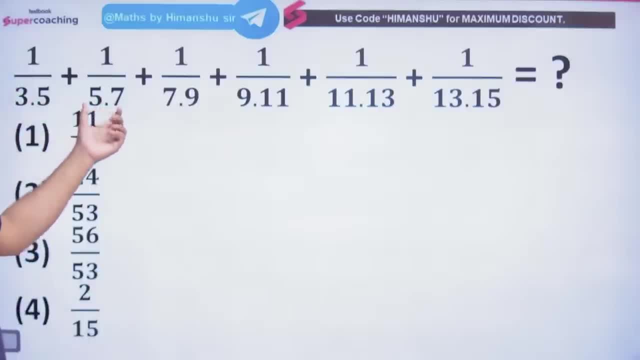 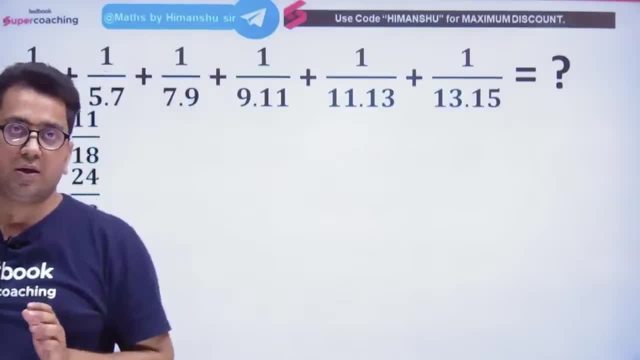 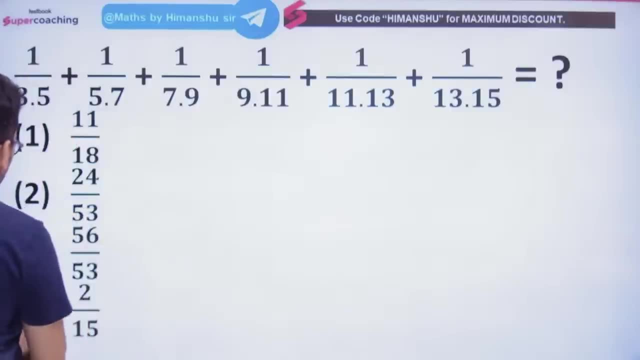 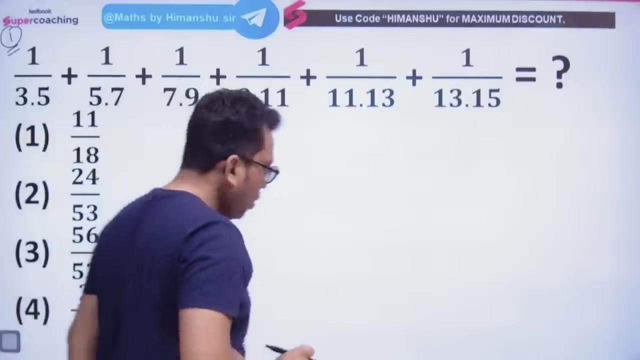 And this way it is going in front of you. okay, Yes, okay, now it is perfect. okay, okay, okay. So the first question of today's session is in front of us. the first question is now about this first question. first we will understand what its concept is and then we will see the way to shine it, okay. 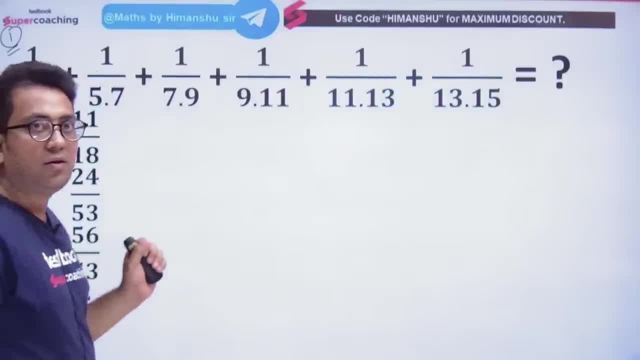 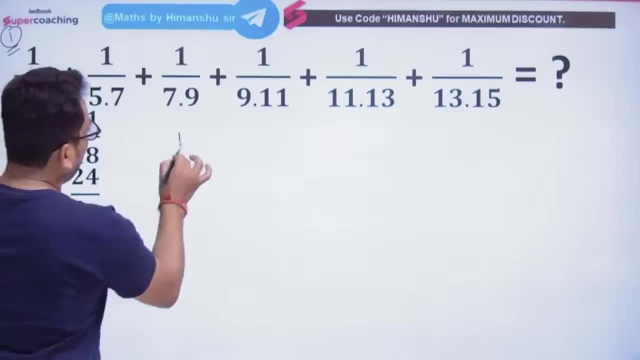 Now see, first of all. now it will be fine, it will be perfect, there is no problem, right? So look. first of all, we will see. See this: 1 divided by 3 times 5 is written. what does dot mean times 5.. 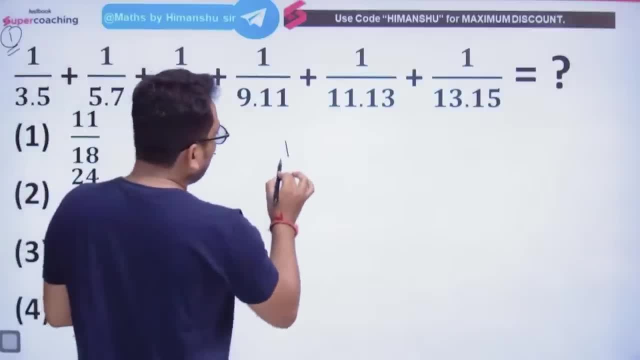 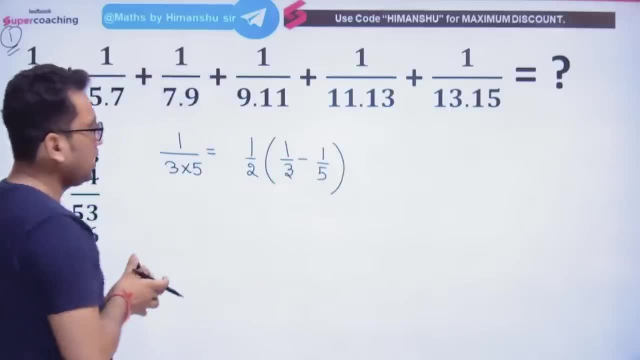 How can I write it in any other way? I can say it like this: that 1 divided by 3 minus 1 divided by 5, okay, And we multiply it by 1 divided by 2.. If I write it in this form, then these two are the same. they are equal. 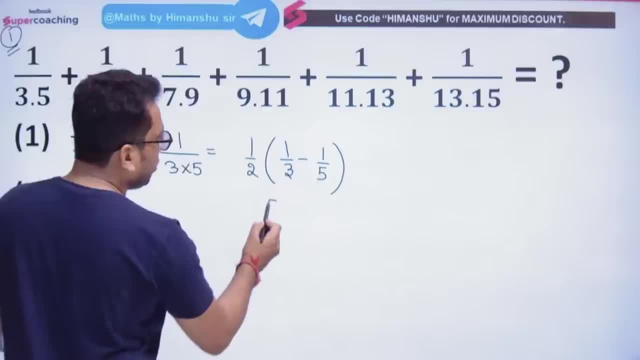 How See? we will show. you See, when I cross multiply, then it will be 5, minus 3 times 1,, then it will be 3, and in, divided by 3,, it will be 5 times 3,. okay, 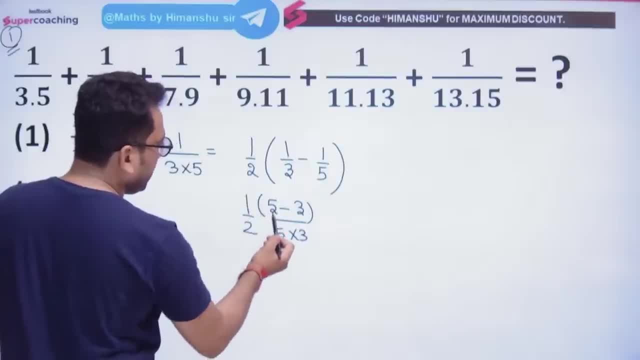 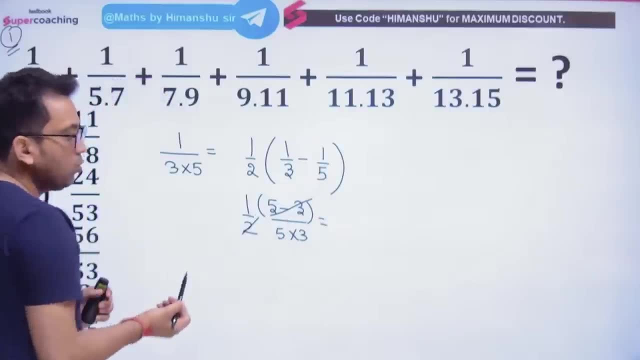 And in multiplied, it will be 5 times 3.. So in this case, what do you have here? you have 1 divided by 2, so 5 minus 3 is 2, and if I cut 2 from 2, then what will come? you will have the same see: 1 divided by 5 times 3,, ie 1 times 3 times 5, so that's the same thing. 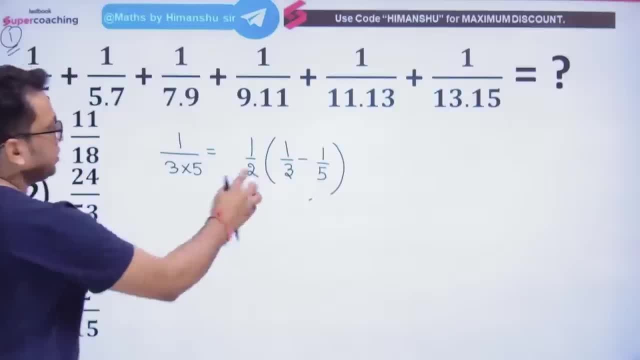 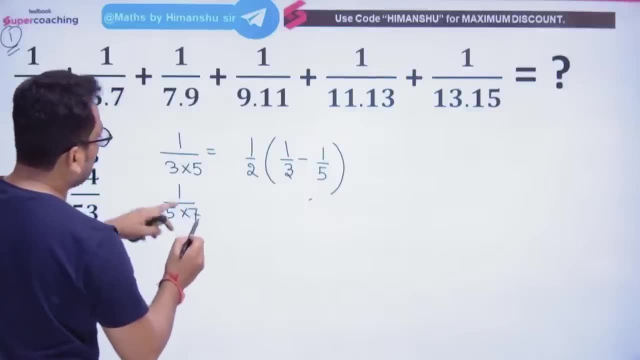 So you must have understood what it means to say that I can write 1 divided by 3 times 5 in this way. In the same way, 1 divided by 5 times 7, which is 5 dot 7,. dot means multiply. how can I write this? 1 divided by 2 times 1, divided by 5 minus 1 divided by 7.. 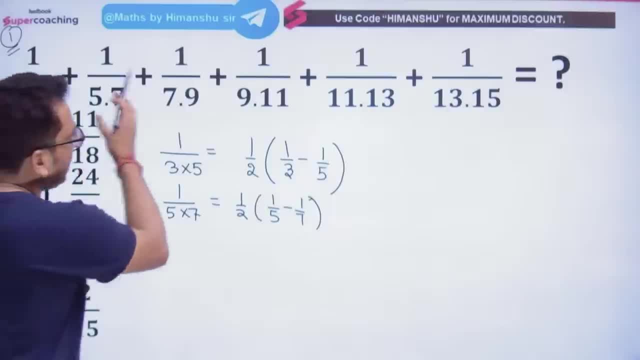 Do you understand what I am saying? In the same way, we can write each one in this form, in this pattern. let's write it. If we write it in this form, then you have this. okay, Perfect. Now, how will this come, son? 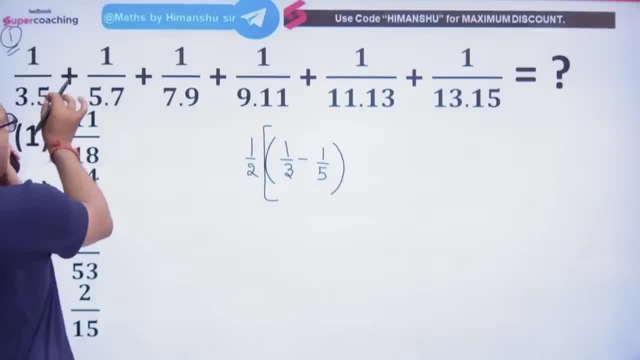 So what I did? I saw 1 divided by 2, it will come here too. 1 divided by 2 will come here too. 1 divided by 2 will come here too. 1 divided by 2 will come here too. so I took 1 divided by 2 as a comma. 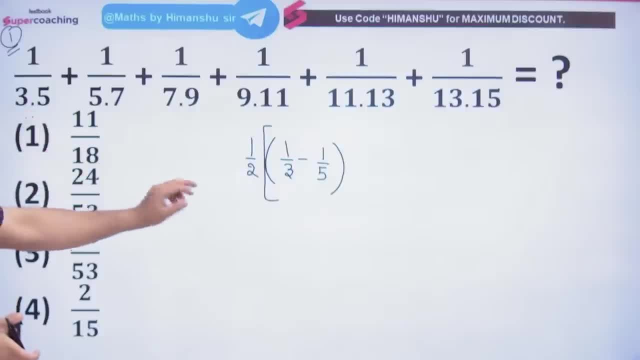 When I took 1 divided by 2 as a comma, then here will be 1 divided by 3, minus 1 divided by 5, here will be son plus 1 divided by 5.. Minus 1 divided by 7, do you say that you agree? 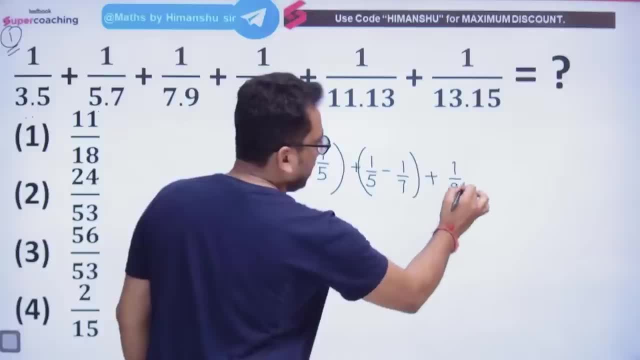 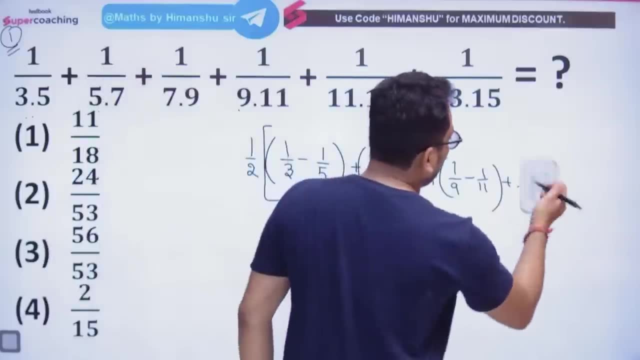 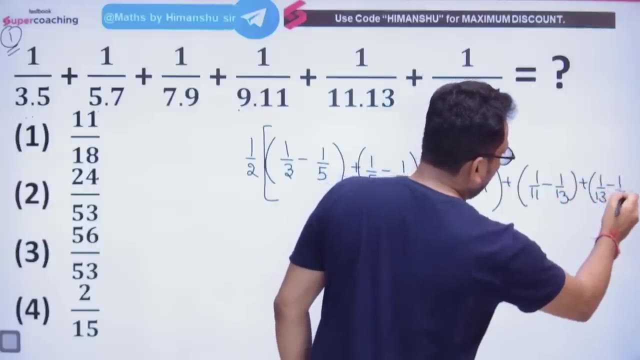 Here. 1 divided by 9 minus 1 divided by 11 will remain inside, right. In this way, these things will continue to move forward, right? So now let's write the whole thing Here. you will have 1 divided by 11 minus 1 divided by 13,, and you will have 1 divided by 15, sorry, 1 divided by 13 minus 1 divided by 15, okay. 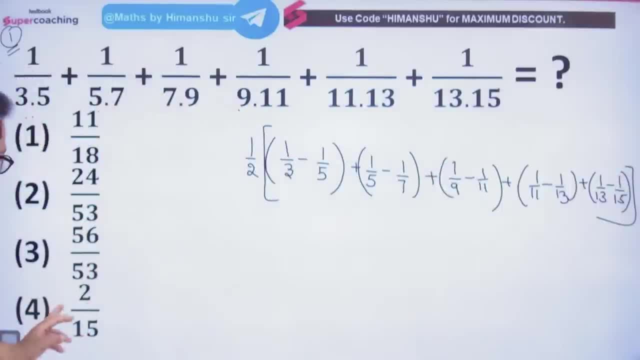 And this bracket is closed and I have kept 1 divided by 2 out. okay, Now let's understand carefully. If I look at it this way, then you can see that okay, Okay, Okay. So this is minus, son, this is plus. it will be cut. 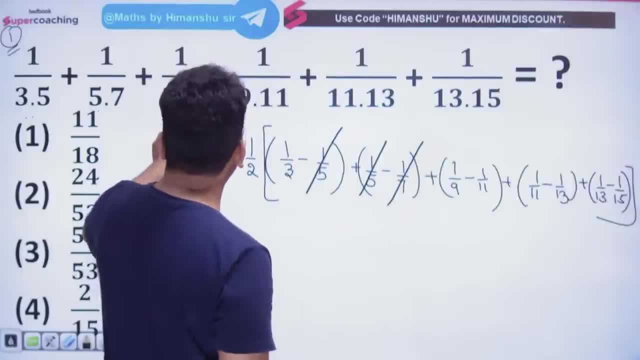 This is minus, okay Here. 7, 9 was also there. 7, 9 will remain. 7, 9 term will come again. 1 by 7 minus 1 by 9, right, This will come again. 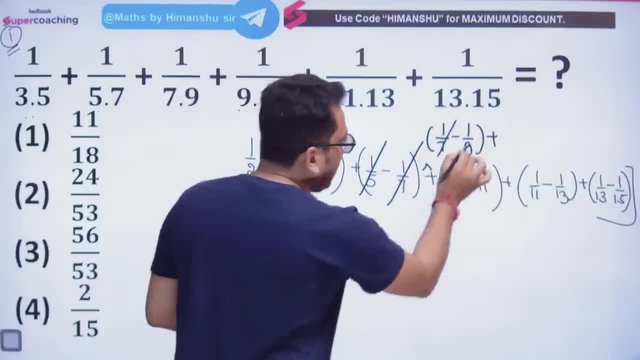 So 1 is minus, then this will be cancelled out by plus. 1 is minus is cancelled out by plus. 1 is minus is cancelled out by plus. 1 is minus is cancelled out by plus. Do you understand what I am saying? 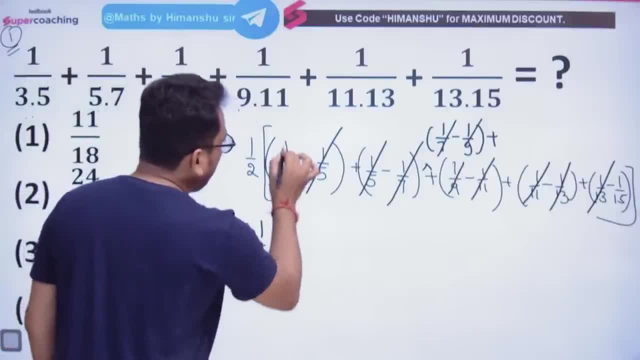 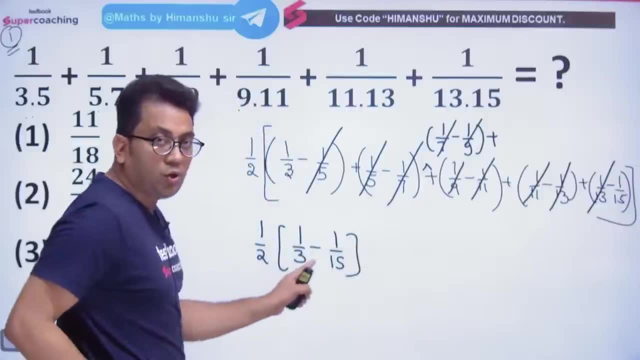 So what is left here? 1 divided by 2 is left out Here. 1 divided by 3 is inside minus this is left in the end. So you have 1 divided by 15.. When I solve this son, then its adhesion is 15.. 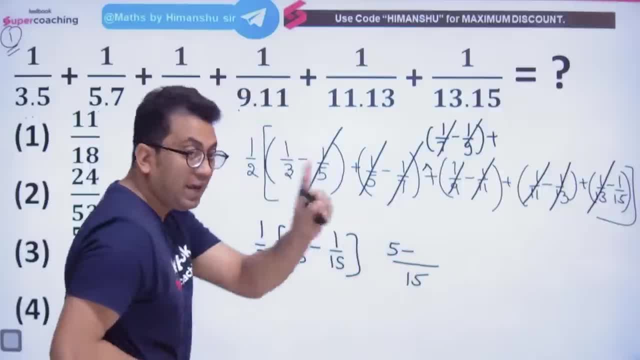 3 times 5 is 15,, that is, it will come up 5 minus 15,. 1 minus 15,, that is, it will come up 1, and we will multiply it by 1, divided by 2.. 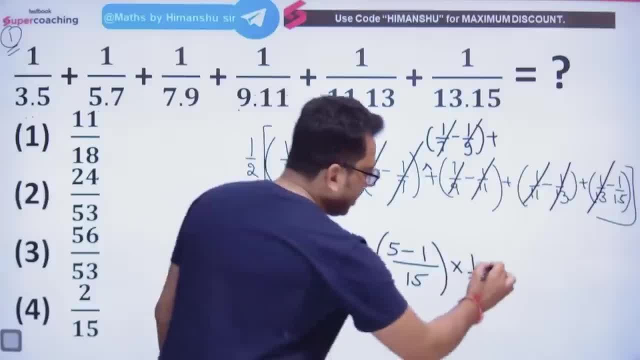 We will multiply it by 1 divided by 2.. 5 minus 1 is 4, that is, it will come 4 divided by 15, and in the multiplication 1 divided by 2, and we will cut 2 by 2,, not 4, so the answer will come 2 divided by 15.. 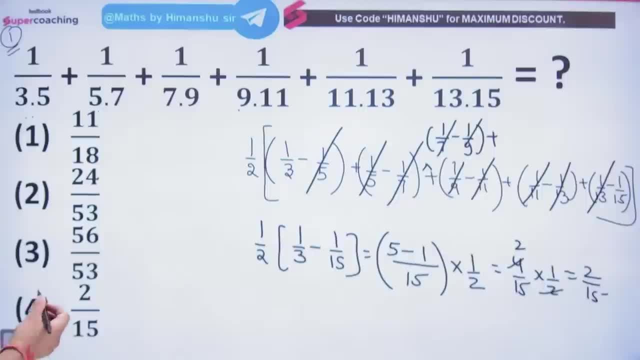 So this is the complete concept. This is the complete concept, son, from which we will get the answer. what will we get? We will get 2 divided by 15, that is option number 4,. our answer will be: 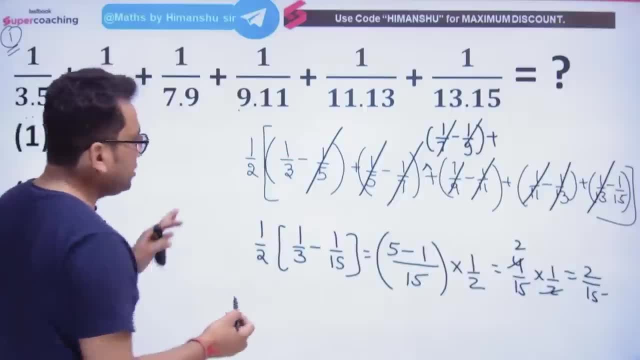 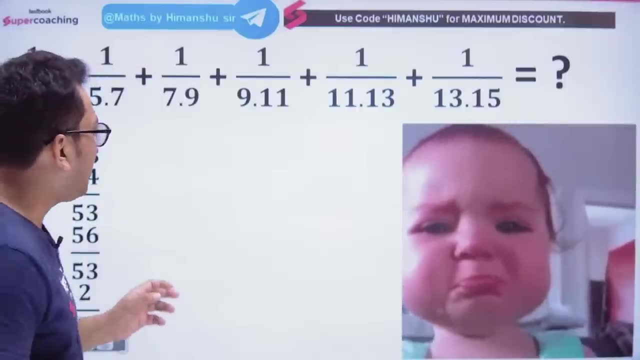 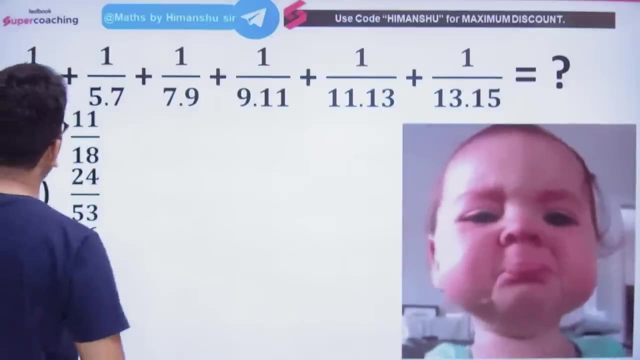 It is perfect. but, sir, when we tell this concept to the child, we tell the whole method. then the child does this. sir, Oh sir, I said, son, why are you crying? what is the matter? They say, sir, do not do this. tell us a way to shine, that we go to the exam, look at the question and tick the answer such a way. 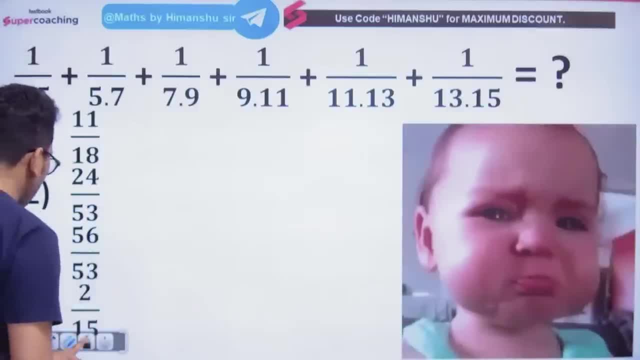 You understand the method. what is that method, sir? What will we do, sir, we will not solve it like this. we will shine. How will we shine? We will just see how many are added up here, that is, one, two, three, four, five, six. how many are there? 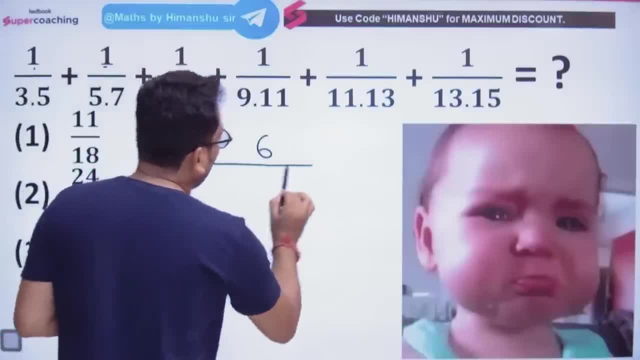 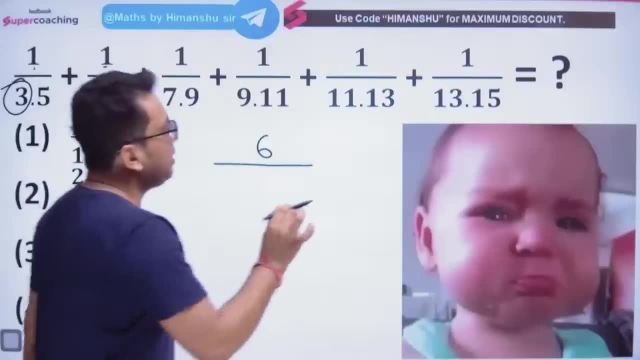 Six. so you write six above, write six. do you understand what I mean? You counted one, two, three, four, five, six, wrote six above. now see what is the first term, three. what is the last term, fifteen. 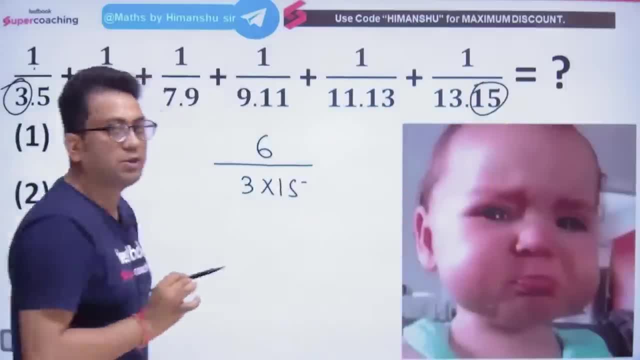 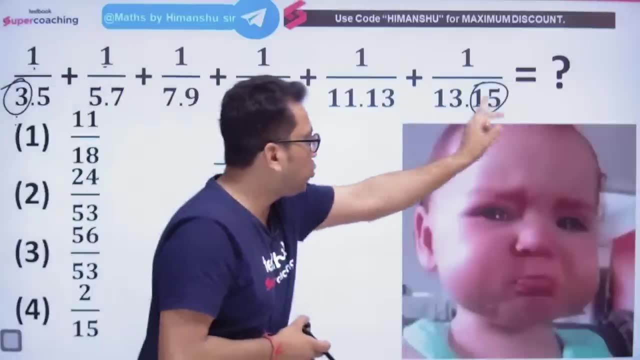 So just do the multiplication of them below. that is three times fifteen. do you understand what I mean In this way? that is, three came down, three came first, then fifteen came. you have to do the first and last step. 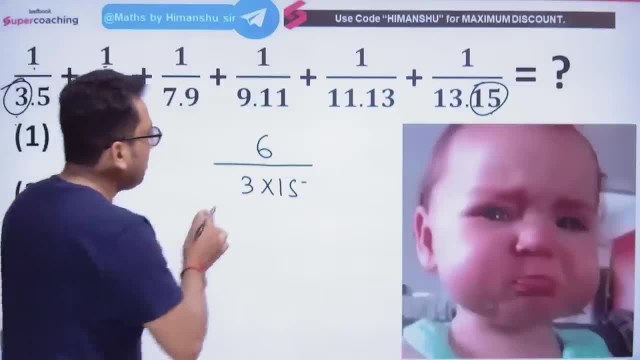 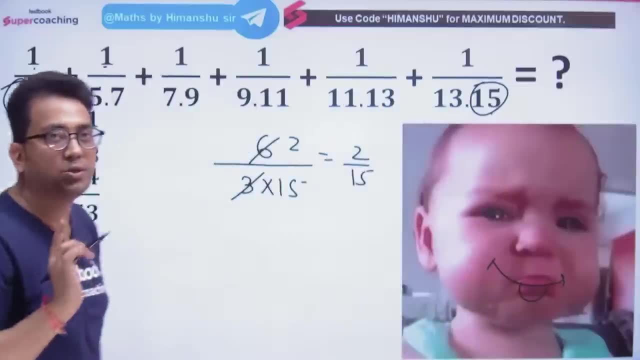 What to do? what to do? what is below? you have to put them down and do the multiplication. That is, if three is below, then the answer will be two times fifteen. So, son, don't cry like this. there should be a smile in it. in my opinion, the right children must have understood. so the answer will be two times fifteen. 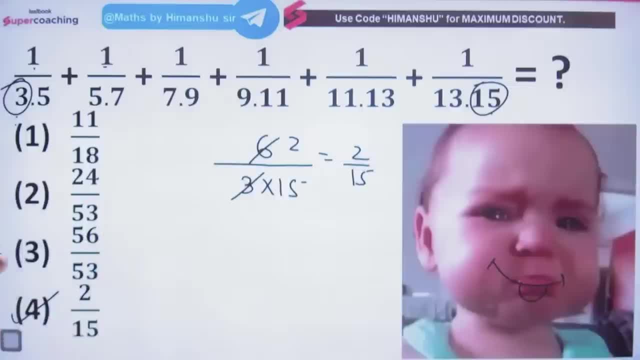 So we have to shine like this. do you understand what I mean? So I have explained the concept to you and also told you how to shine that when you go to the exam, how you have to do it. Okay, if you understand the matter, then the next question is coming in front of you. the next question is in front of you. 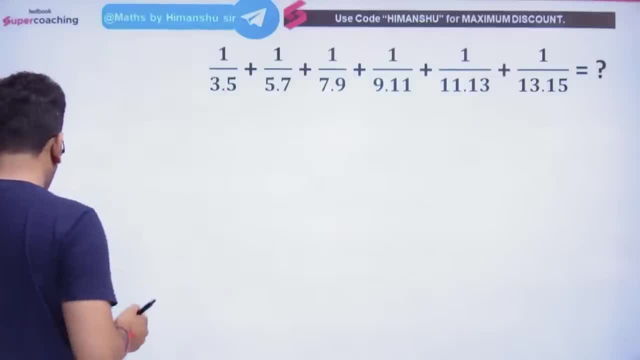 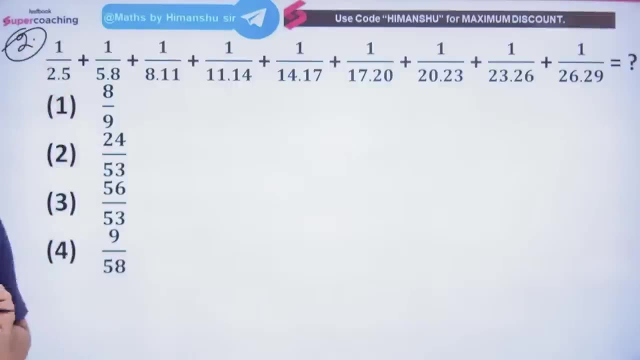 I want you to: Let's take this question. Let's take the next question Quickly. shine this question every time. Next question: Question number two is today's session. Quickly answer the second question with everyone. Come on. Afshan Naaz is saying: sir, first tell me the long method, then shine. 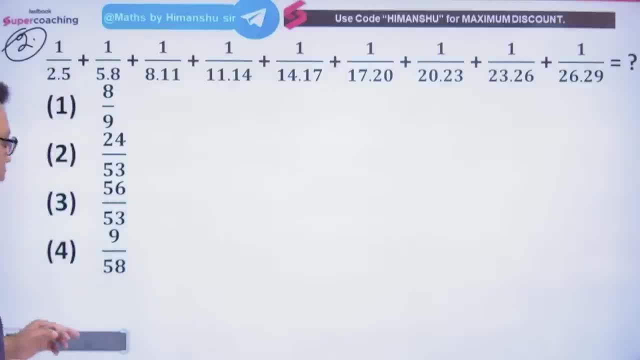 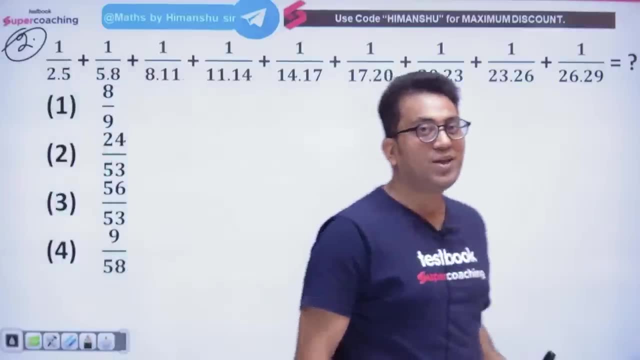 Okay, now come on, answer this question first. quickly tell me what the answer will be. It is not a long method, son, it is a concept. Okay, What do you think This is the way to shine? It is not like this. it does not fly out of the air. 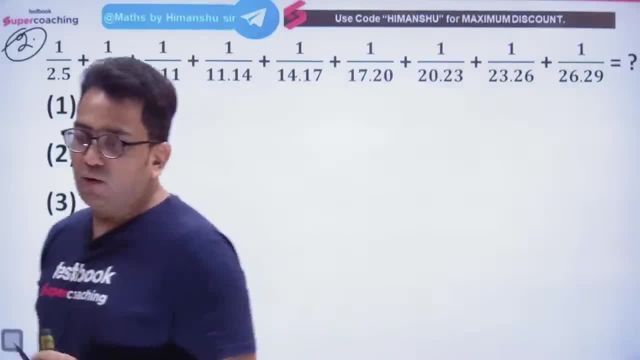 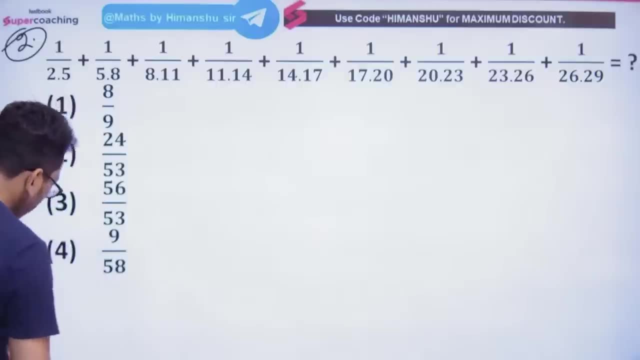 It comes out of the same concept, Isn't it? Come on, tell me quickly. I would like every child to answer. Let's see how many children are able to answer. Look what do you have? Consider a simple funda here, son. look carefully, a pattern is going on. look, a pattern is going on here. 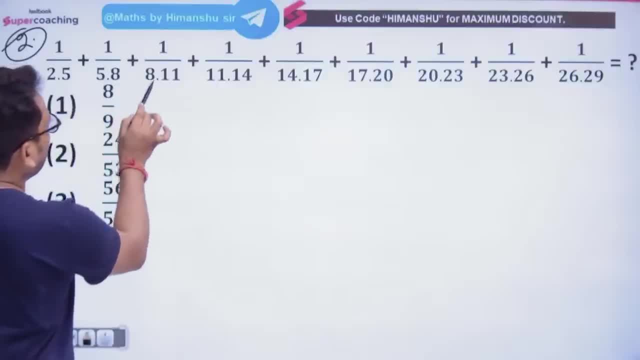 What is the pattern going on? Two, five is three, five, eight is three, eight, eleven is three, eleven, fourteen is three. there is a difference: of three, three, everywhere. This should be the difference. it should be two, it should be three, it should be four, it should be five, no matter how many. don't worry about yourself. 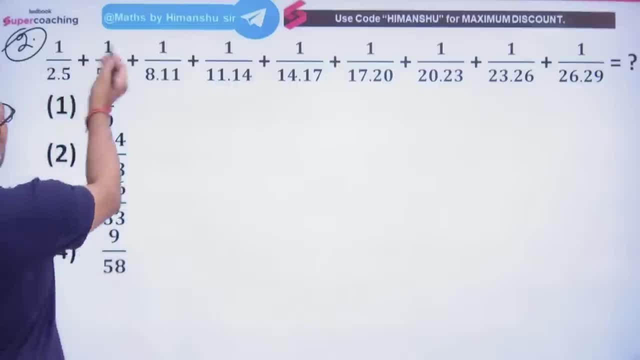 This should be the difference. So you have to see this pattern again. How many are there on top? So one, two, three, four, five, six, seven, eight, nine. So you put nine on top, son, like this: 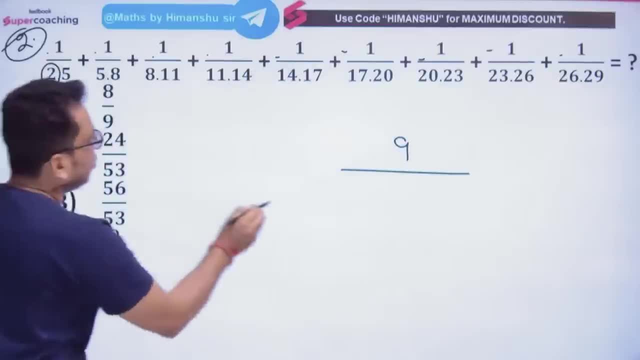 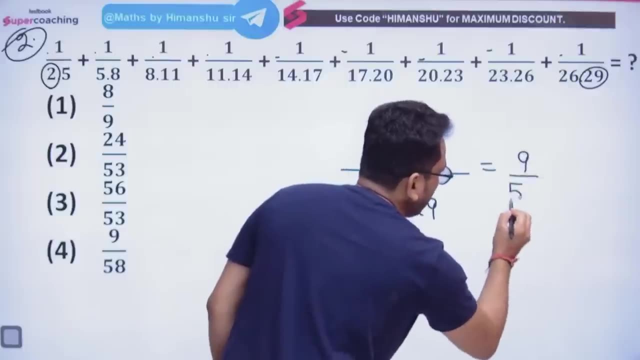 And what will come in the pattern? What is the first line here? There are two below. And what is the last line, Sir? the last line is twenty-nine, so here is twenty-nine, So the answer will be nine divided by twenty-nine, not fifty-eight. 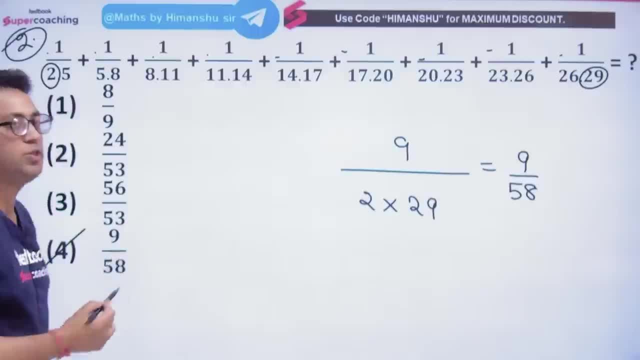 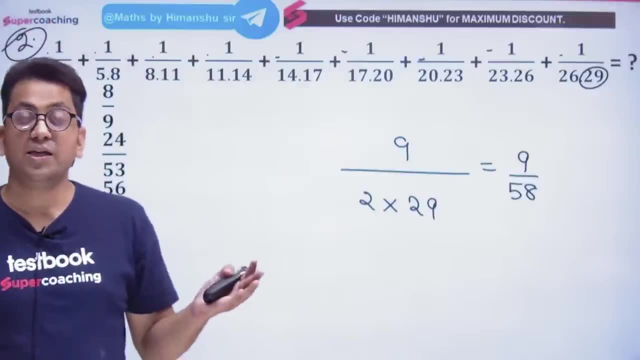 That is. our answer will be nine divided by fifty-eight, which we can see in the equation four. So the children who are answering D: their answer is absolutely correct. Okay, It's fun, Things are coming to understand How to shine in your exam. 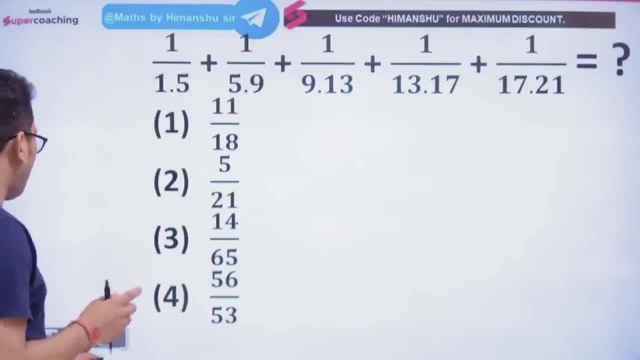 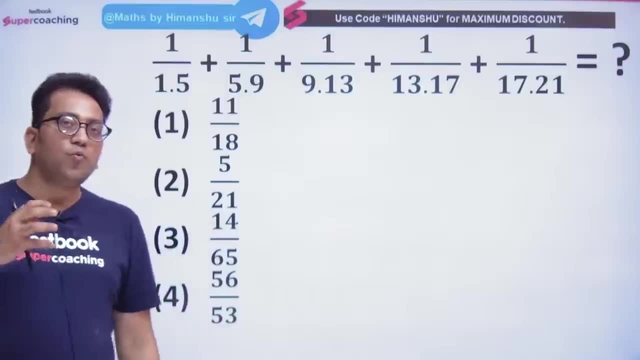 The next question is coming in front of you. I say that it is in your hands to make the question easy. Is the question that came in the exam easy or difficult? How is it? It is on you. If your solution is easy, then that question is easy for you. 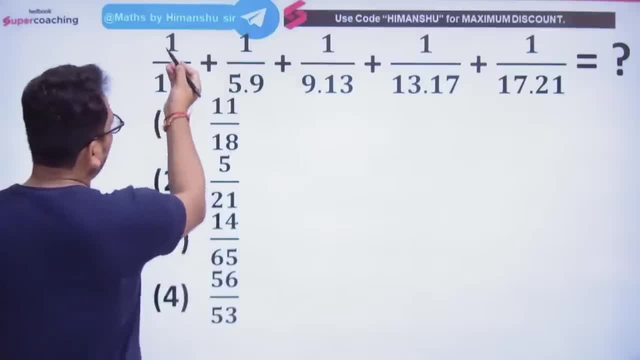 Tell me quickly. the next question is in front of you, Son. one in one. one to five things are going on like this. Tell me quickly what will be the answer. The question number three of today's session is in front of you. 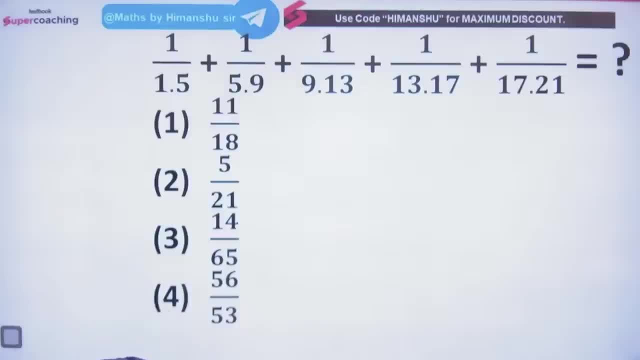 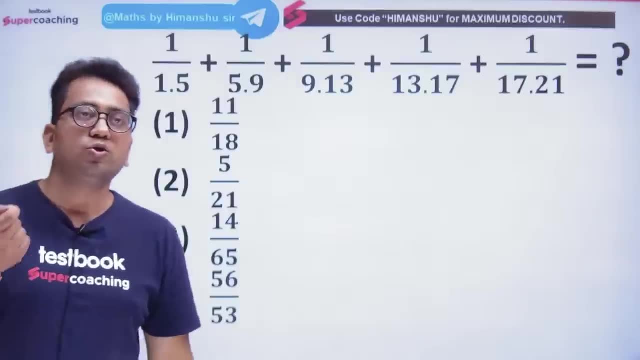 The third question: Answer all of them And like and share as much as possible. son, All of them, Isn't it? I would like every child to like and share the session once. Whatever was the problem in our session? Okay. 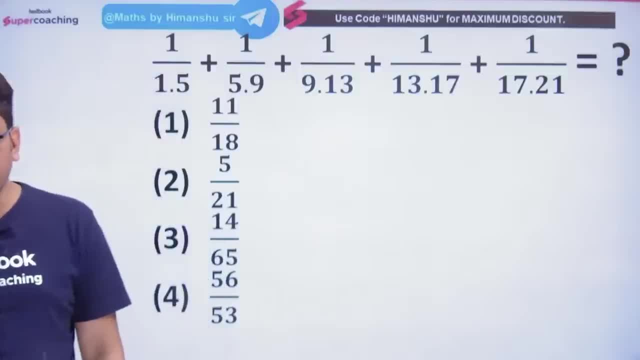 That is fine now. So you all tell the children once, Share it so that every child comes and joins the session. Okay, And look, this is your support that I am continuing these classes, Because, look, I am giving 100 percent in my way. 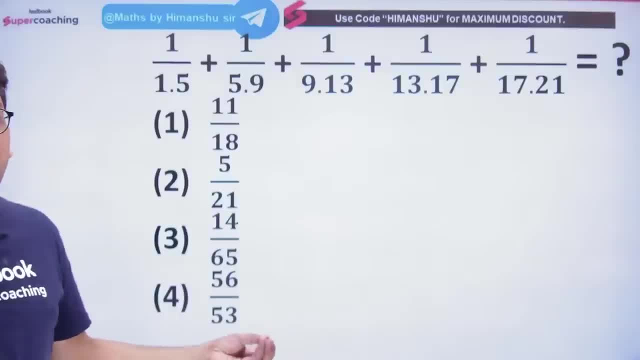 So I would like every child of mine to give 100 percent. Come here and join. Okay, I am making you do very important things. I am giving you such content that you will not get anywhere. So you all come and join at 12 o'clock. 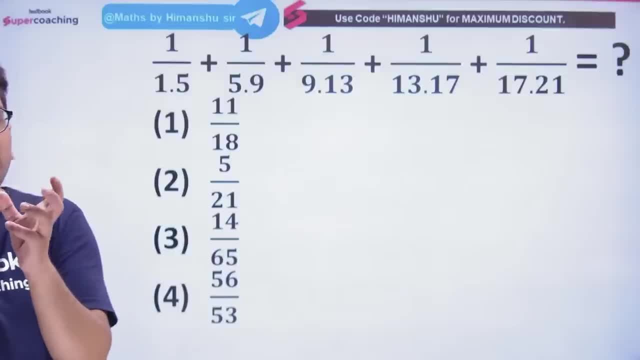 And you will find that difference inside you- Yes, sir, In math, which I did not know before, And how much better I have become, Or I have become Son. the next question is in front of you, It is given to you. 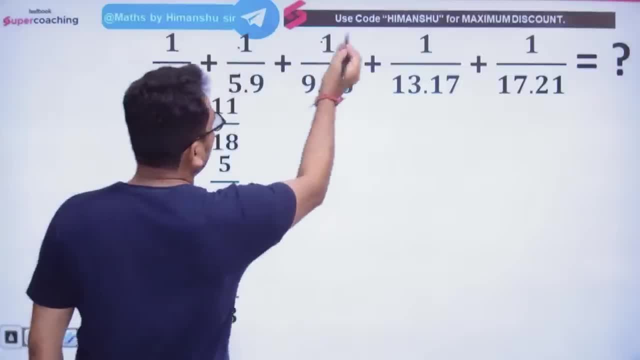 You tell me how many are here. So you said one, two, three, four, five. So you wrote five above. What is the first line here? What is the last line, Son? there is 21 here, So 1 times 21.. 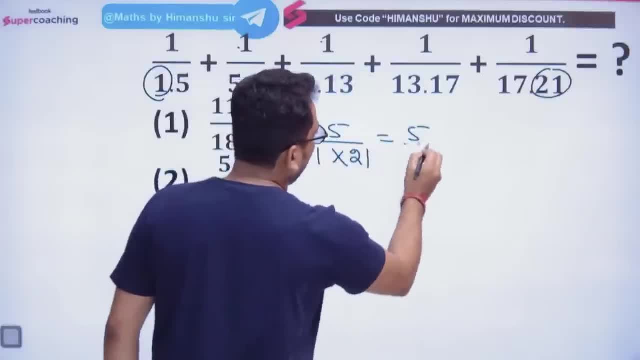 So what will be the answer? we will have 5 divided by 21.. That is option number 2 will be our answer. Our answer will be 5 divided by 21.. Can you understand? Can you do it? The next question is coming in front of you. 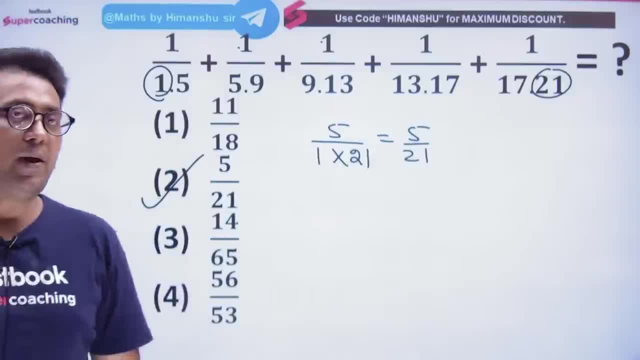 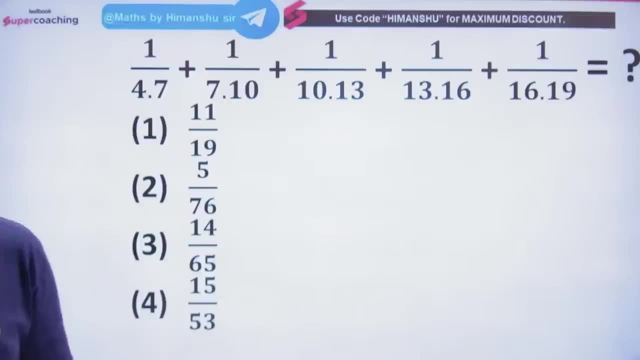 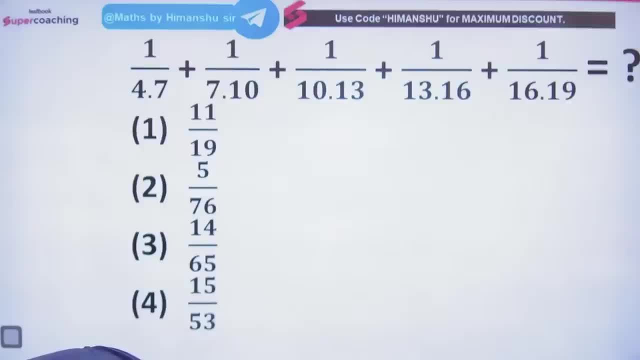 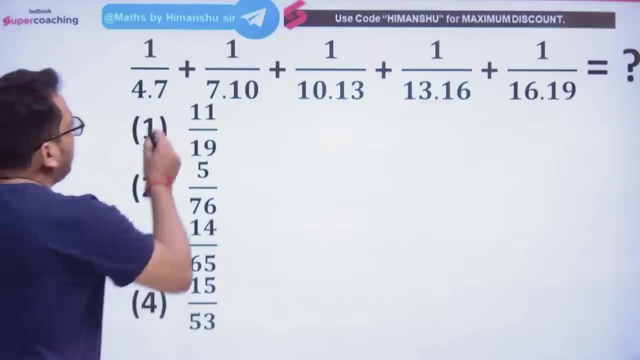 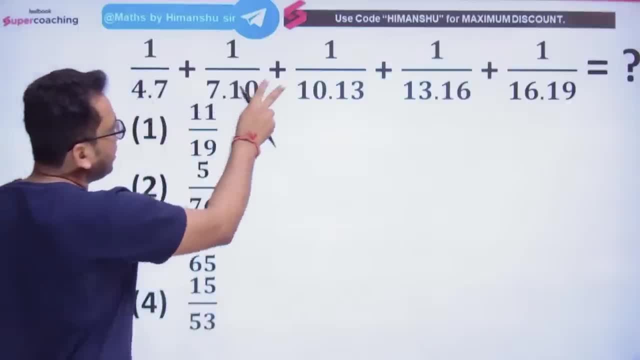 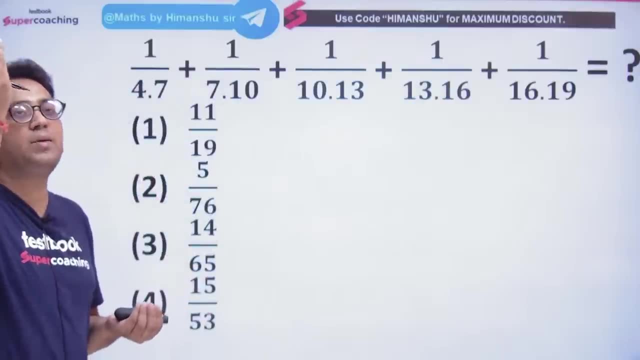 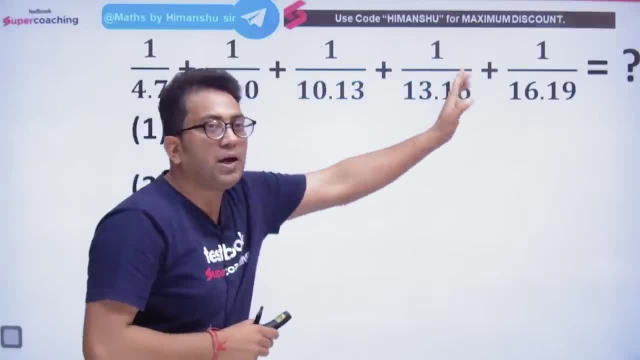 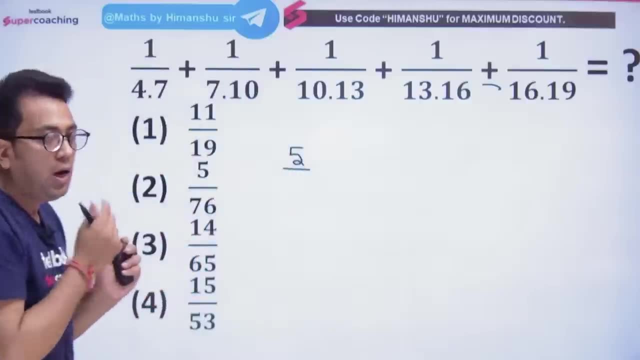 Then you will say One, Two, 5 times. So what will come up? 5 will come. You have to see the number 1, 2, 3, 4, 5.. 5 came up. Now what is the first line? Below 4 is written. So you have written 4.. What is the last line? 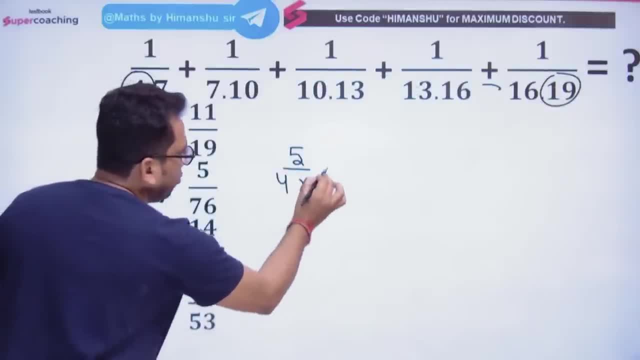 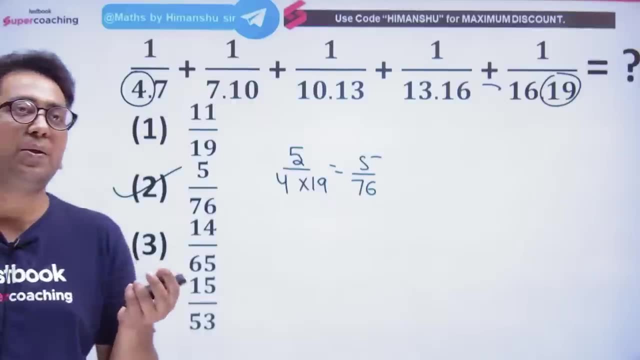 Here is 19.. So you have written 19 and done down the number. That is the answer will come 5 divided by 19.. So you will get the answer. option number B. The option B will also be our answer. Are you able to understand everyone? Is it clear? Go ahead. The next question is coming in front of you. 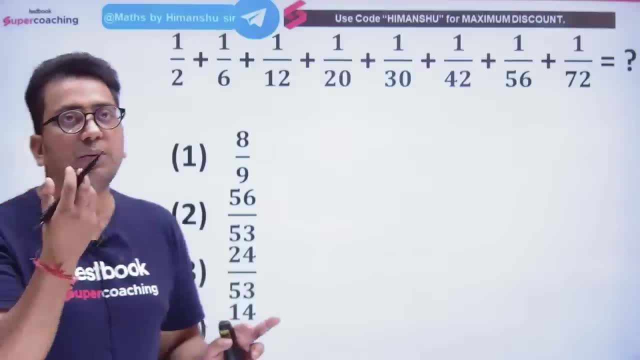 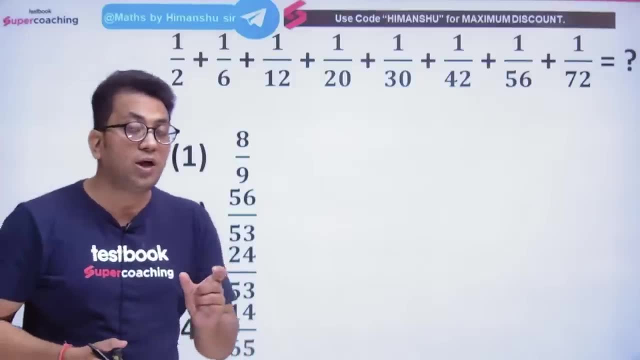 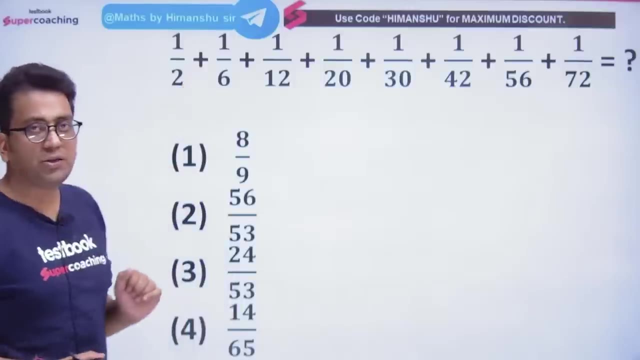 You are seeing how easily you are answering the question. Now some child will say, sir, will it be so difficult in elementary math? My dear, what did I say? Is the question difficult or easy? It depends on you. Now come to this question. I told you to join like this, So will you take their? 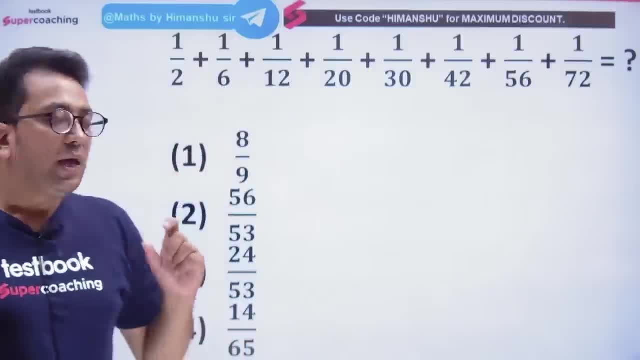 LCM by sitting in the exam. No, brother, you don't have to take LCM. You have to make this question as your own. You have to make this question as your own. You have to make this question as your own. 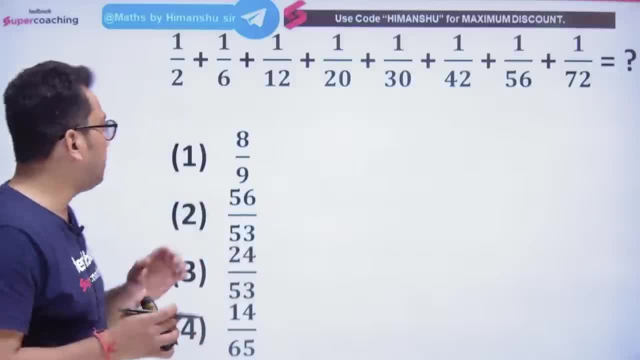 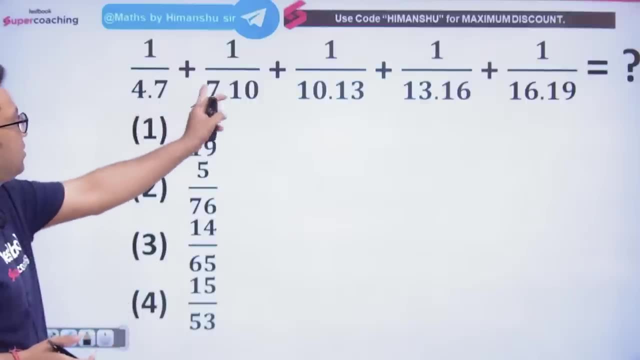 How will you make it, sir? What are you saying? Come on, Let's make this question as your own, As you people just understood that we were able to ask this question here right 4,, 7,, 7,, 10,. 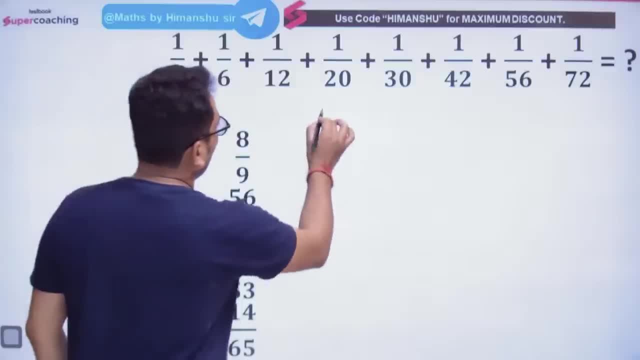 10, 13,. in this way, Sir, how can we do it here? So see, can I write 2 as 1 times 2, plus, Can I write 6 as 2 times 3?? Say yes or no. Can I say 12 as 3 times 4? Can I say no? Can I say 20 as 4 times 5?? 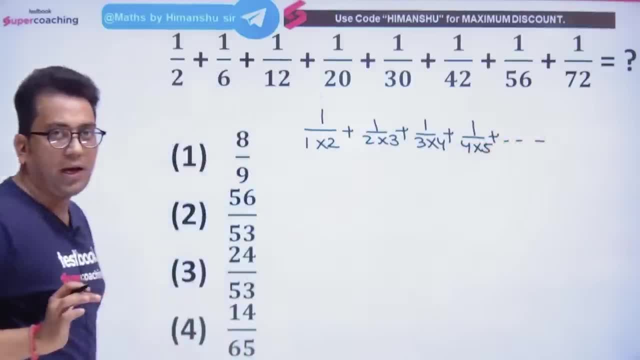 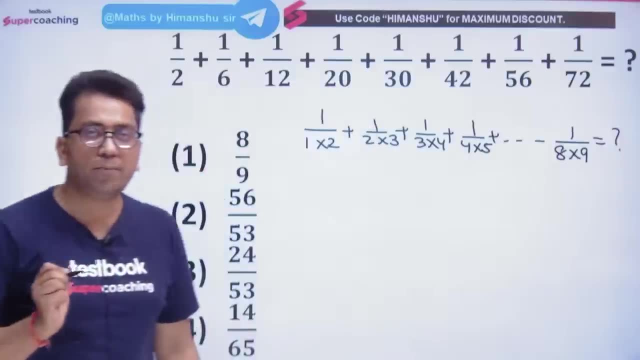 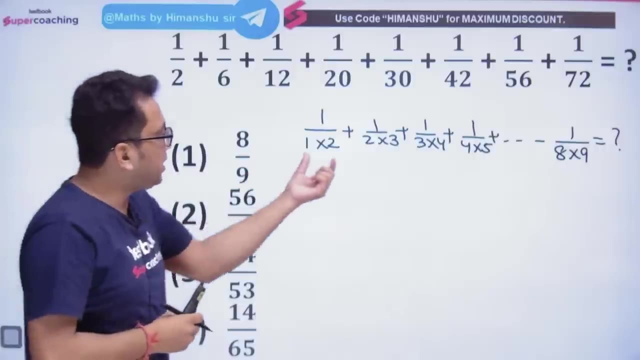 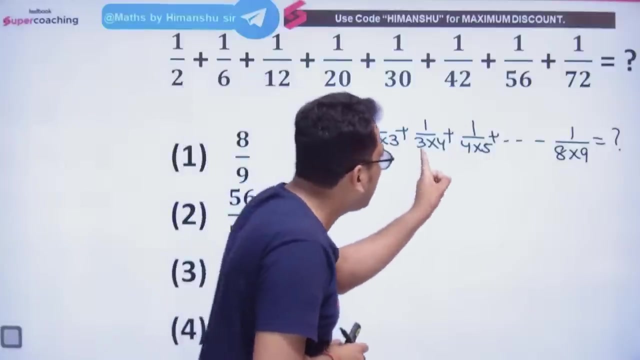 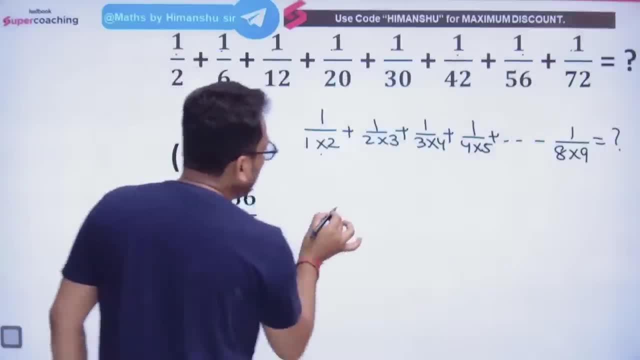 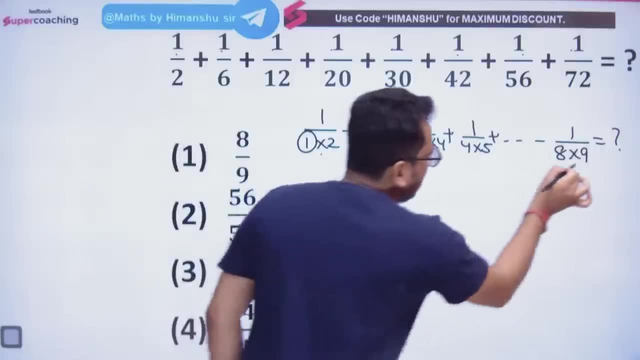 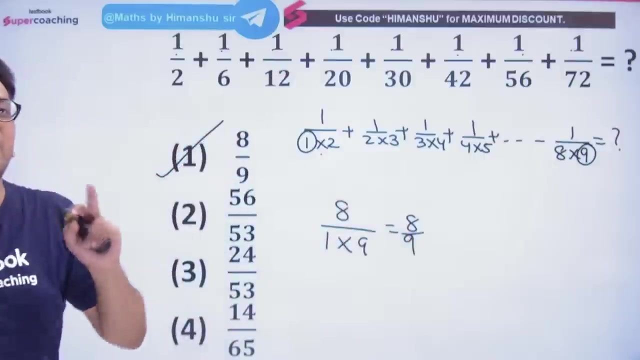 So 1,, 2,, 3,, 4,, 5,, 6,, 7,, 8, so, sir, 8 came up. they are clear. what is the first step? the first step is 1,. what is the last step, sir? the last step is 9, so the answer will come to you: 8 by 9,, that is, 8 by 9, our answer will come, which is one option you can see. so 8 by 9 will be the right answer. ok, it is perfect. it is fun. things are coming to understand. it is fun, things are coming to understand. son press, like and share. 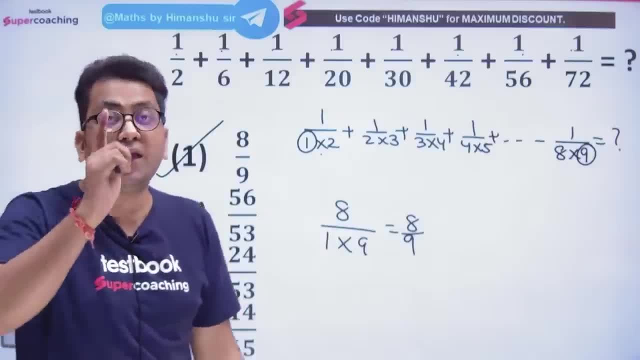 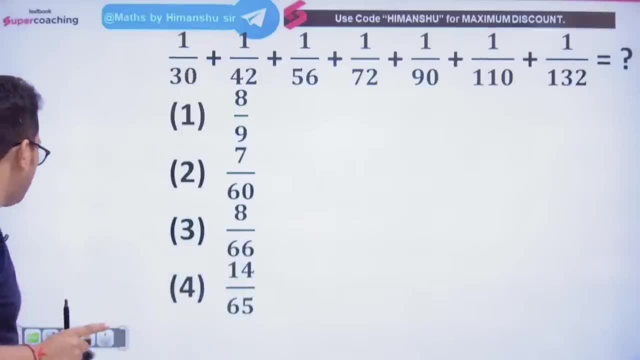 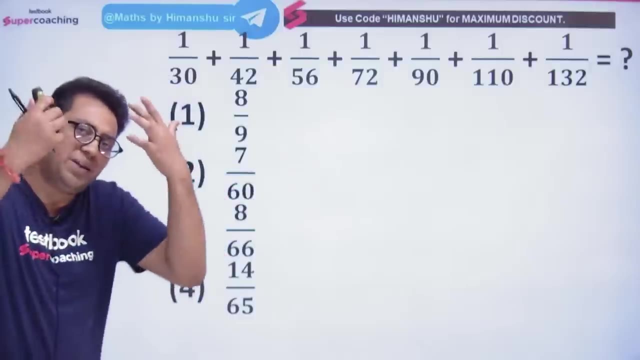 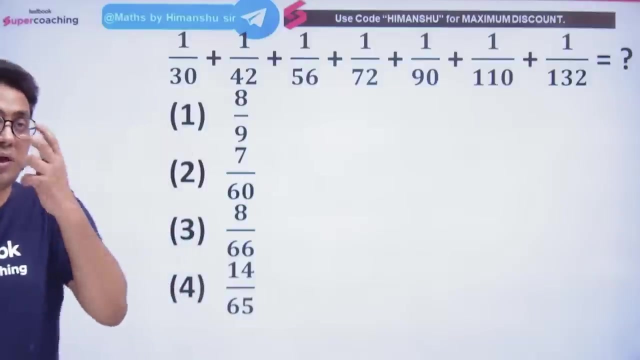 Ok, All these things that you will find here in Himanshu sir's session at exactly 12,. it is fun, let's go ahead. next question. the next question is coming in front of you. shine quickly what you have to see. you do not have to solve this. you have to make this question as yours because you have understood those things. now try a little bit, put some effort. how can I make it as my own? how can I make it? try it. try it, son, and tell me what. the answer will come soon. 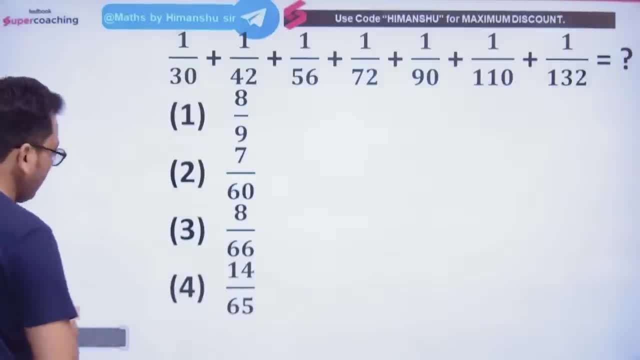 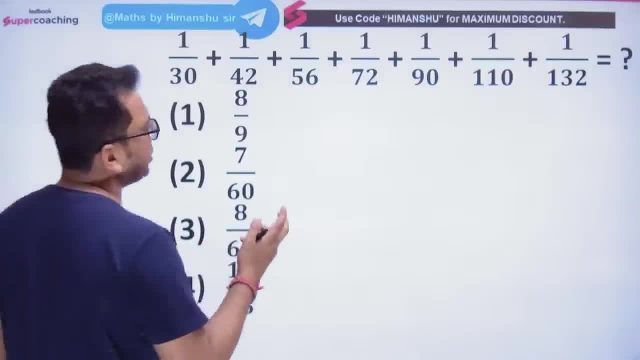 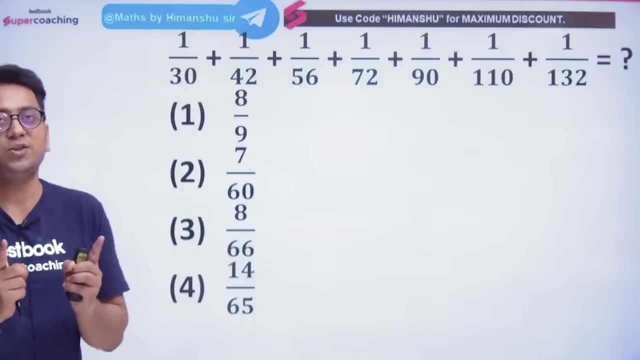 Come on quickly with speed. maximum Like and share should be maximum. Put fire in the session today. Hurry up and share all of them. I want my every share and share in today's session, Because today the things I am giving you are very good things. 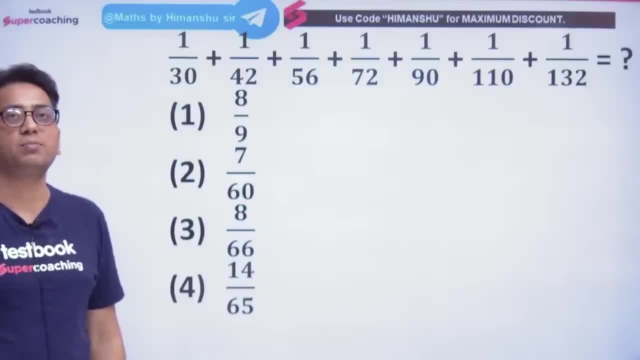 I want these things to reach every child, So share maximum. See what he is saying to you: 1 by 30,, 1 by 42,, 1 by 56, it is going like this: 1 by 132.. 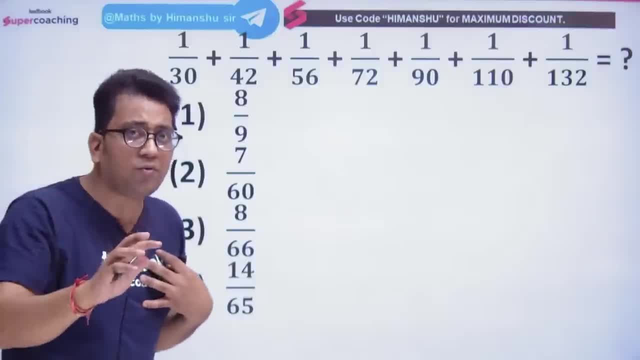 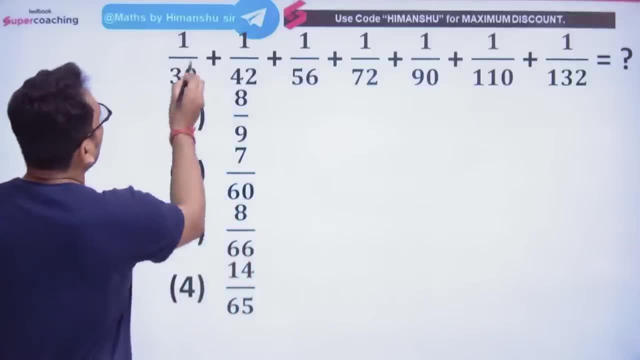 Now see, I understand and believe many children. I am very weak, sir. They don't understand how to write 132 directly. No problem, You see here, Run the pattern. Hey, you will be able to catch 30. that 5 by 6 is 30.. 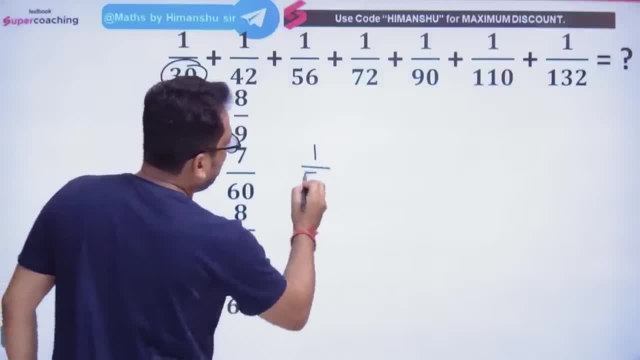 5 by 6 is 30. Say yes or no, 5 by 6. You will be able to say, like this: right, If you see 42 as 5 by 6, then the next should be 6 by 7.. 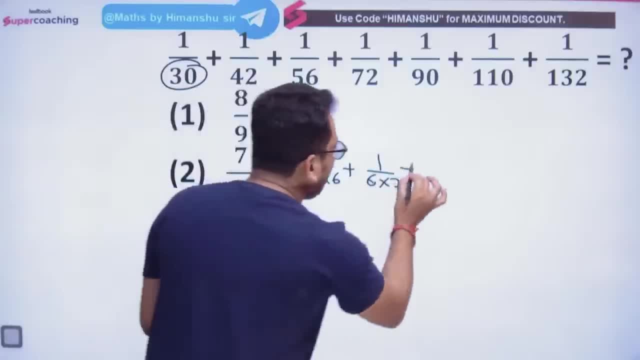 See: 6 by 7 is becoming 42.. So you just have to see, you don't have to write. I am telling you by writing this. Now look ahead. If this is 6 by 7, then the next is 7 by 8, is 56.. 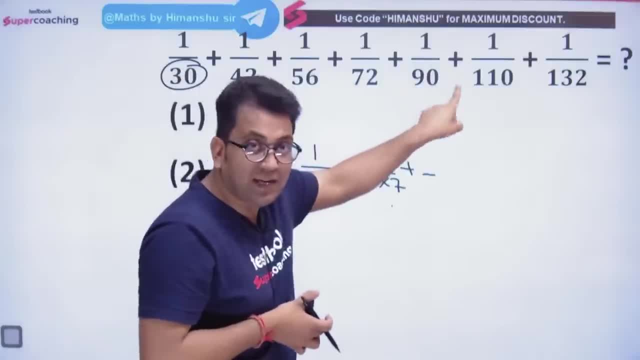 Yes, sir, 8 by 9 is 72.. 9 by 9 is 92.. Right, If you multiply 10 by 11,, then it is 110.. And if you multiply 11 by 12,, then it is 132.. 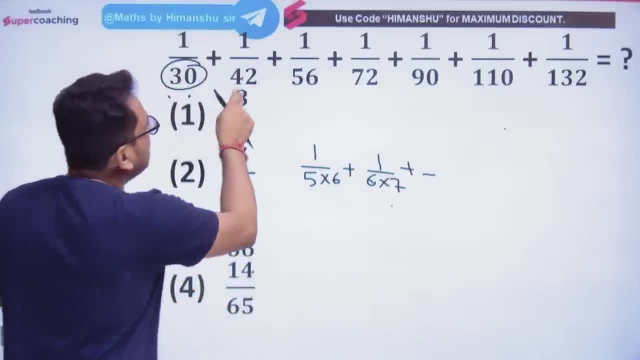 So you will understand it yourself. That first is 5 by 6.. 6 by 7 is 7. Right, 7 by 8.. 8 by 9.. 9 by 10.. 10 by 11.. 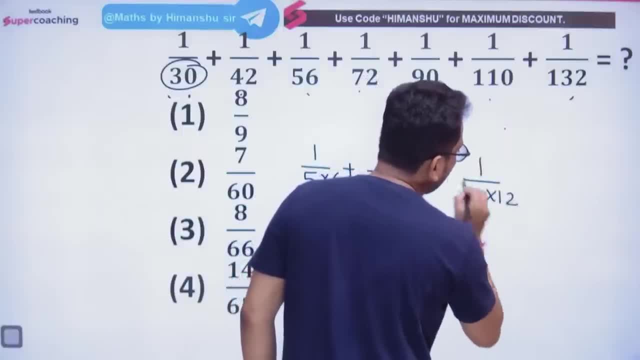 And 11 by 12.. That means you will get 11 by 12 at the end. Are you understanding what I am saying? Like this, And you just have to see how many times: 1,, 2,, 3,, 4,, 5,, 6,, 7.. 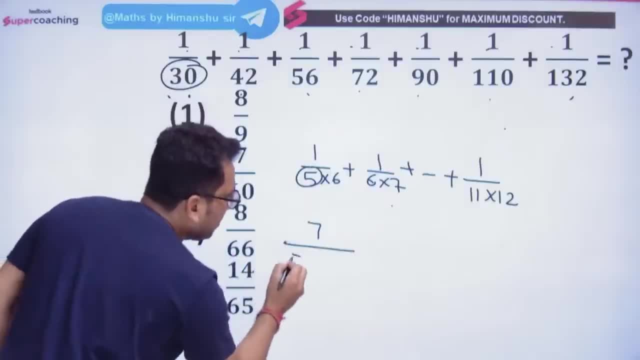 Seven times, then seven comes up. What is the first step, My child? there is 5.. What is the last step? There is 12.. So you will get the answer: 7 by 60. That means 7 by 60.. 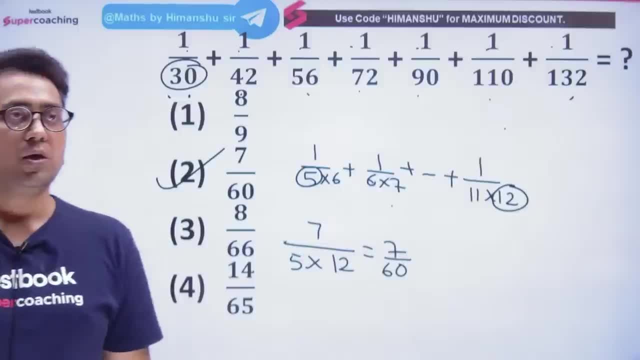 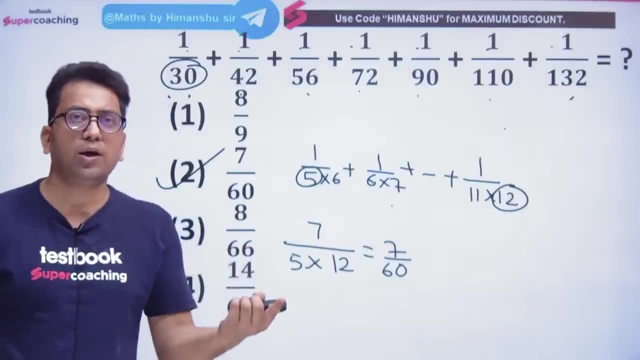 That means option number two is our answer. Right Two will be our answer. Even our answer will be: Are you able to understand now? Is it clear? Can we move ahead? Next question: The next question is coming. The next question is coming. 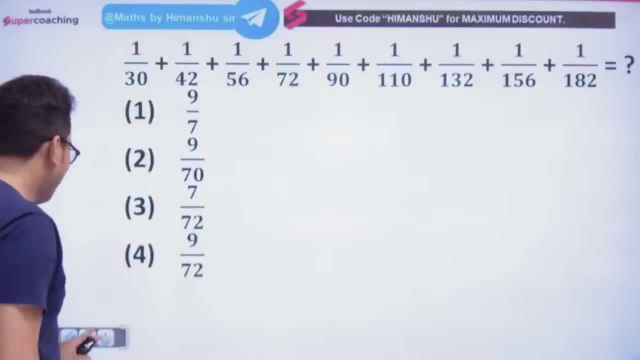 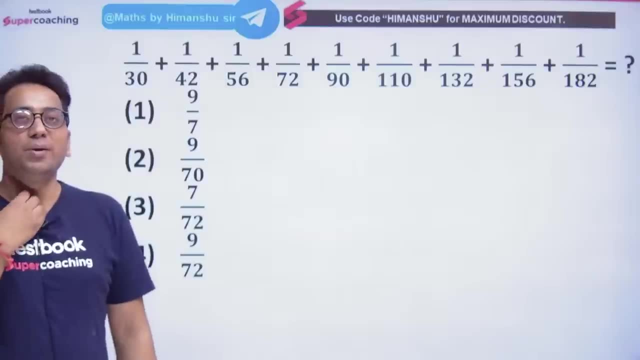 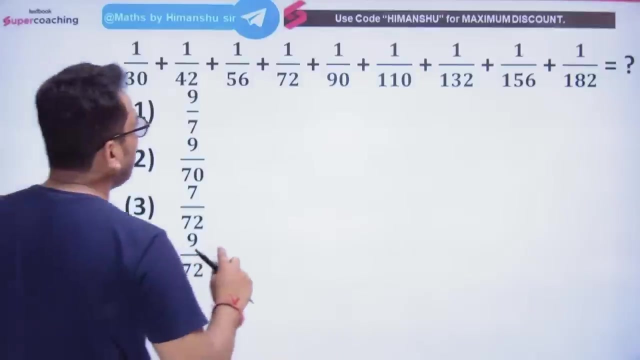 Okay, Come on, brother. This fire is only to put fire in the comment section. It will take a lot of time, but share the maximum. I would like every child to come here and join And the things that are being given. I don't tell you to go and practice separately. 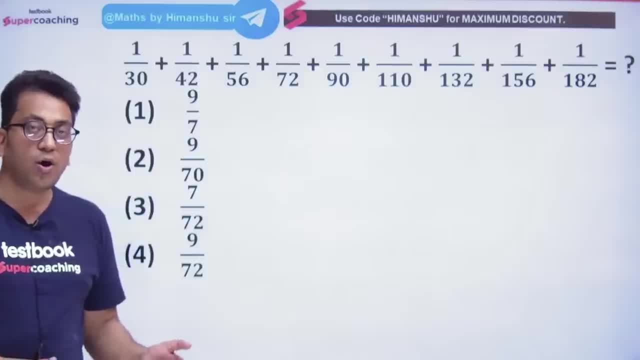 No, I am saying that you come at 12 o'clock and join And I will develop that interest in you to do math. This is my guarantee. The next question is in front of you: 1 divided by 30 is equal to 1. divided by 42 is equal to 1 divided by 56 is going this way: 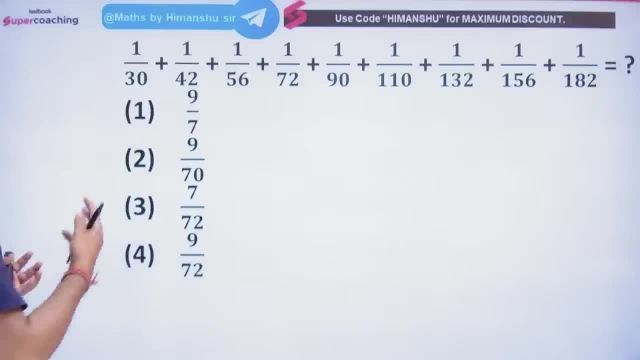 1 divided by 100 is going up to 82.. Sir, the child does not understand what to write to 82.. There is no problem, You follow from here and you will reach there. They say: right What Sir? we will reach the destination. 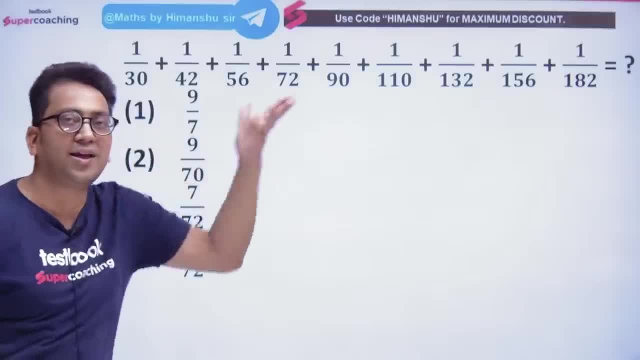 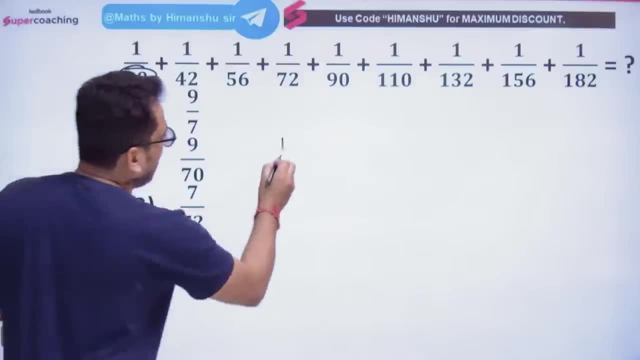 It's just the time to leave. If you don't leave, how will you reach the destination? So leave, You see for yourself. Brother, what will I call 30?, 5 and 6.. That is the first one who came. he came. 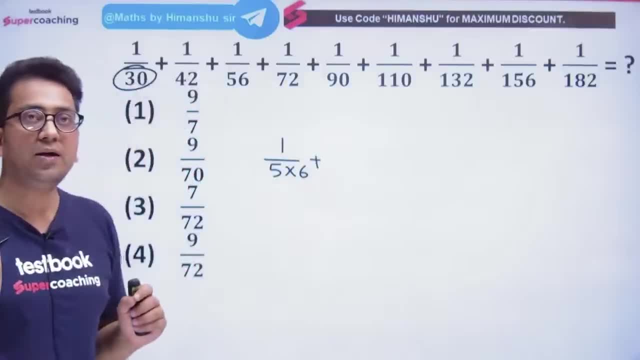 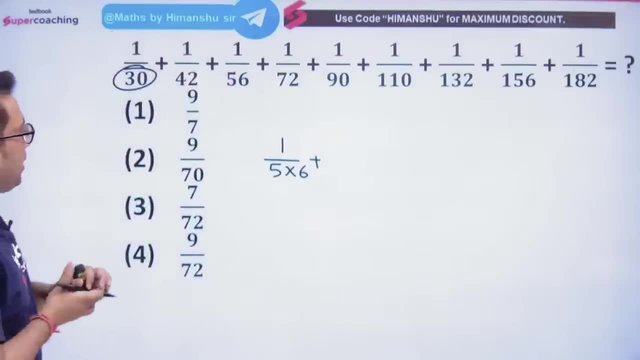 5 divided by 6.. Are you understanding now, Isn't it Sir? please, Please, get a session of profit and loss done. Nahid is saying: Son, we will do it, absolutely Okay. 1 divided by 5 is equal to 6.. 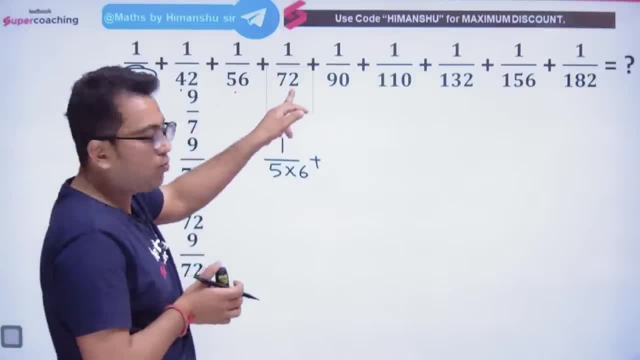 After that, 6,, 7,, 7,, 8,, 8, 9 is 72.. Absolutely, 9 is 92.. 10 times 11.. 11 times 12.. 12 times 13.. 13 times 14.. 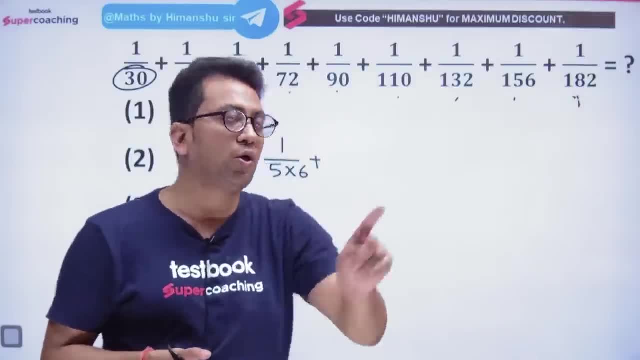 13 times 14.. See, whatever you don't understand, you will do that too: 13 times 14.. That is, you will get 13 times 14 at the end. So look at the math, son. How many are there above? 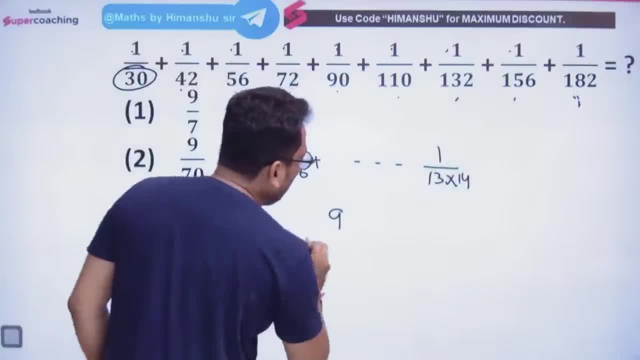 1,, 2,, 3,, 4,, 5,, 6,, 7,, 8,, 9.. So 9 came up, 9.. What is the first step? What do you have? 5. What is the last step? 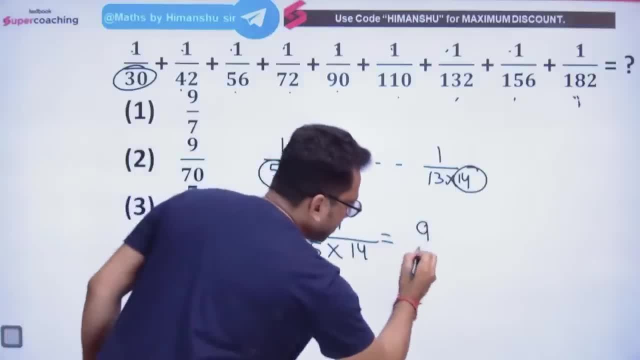 You have 14.. So it came 9 divided by 14 times 5.. That is, 14 times 5 is 70. Son. so 9 divided by 70 will be our answer. That is, we have only two options here. 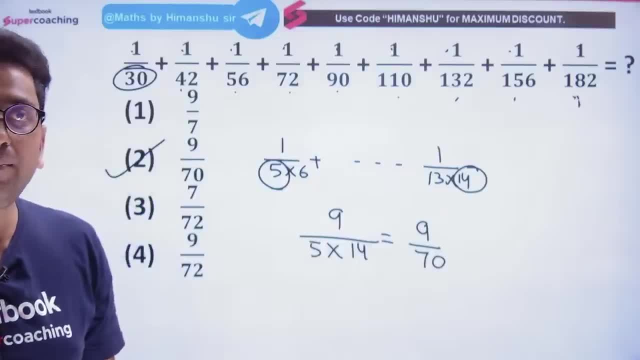 Okay, So 9 by 70 will be the right answer. Is it clear? Are you all understanding? It is perfect, We can move forward. Come on, the next question is coming, son. The next question is coming Here, it is in front of you. 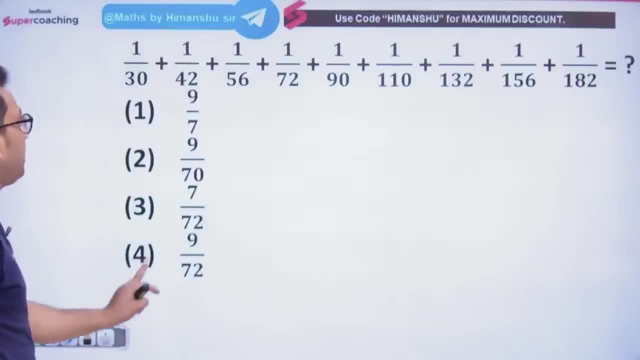 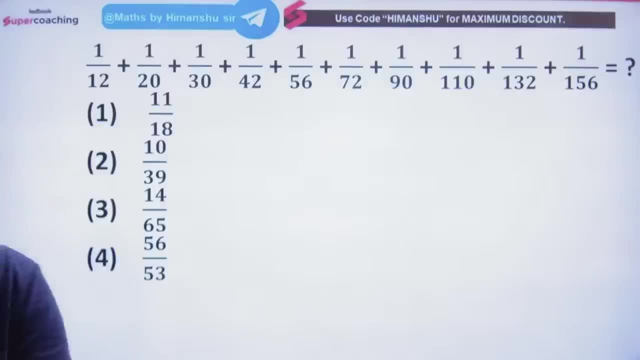 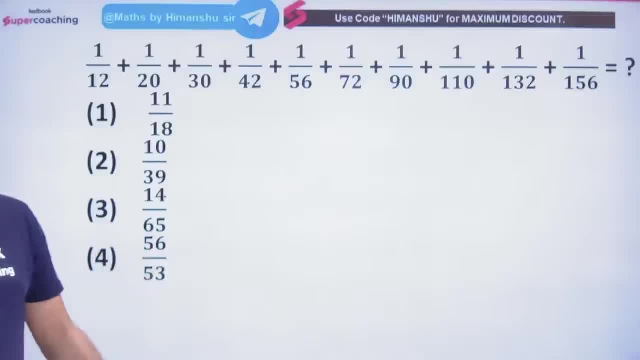 Don't fight son, Answer it, Come on. all right, I can see Babita, Ashutosh Kunal, Snigdha Pooja, Hare Krishna, Mayur Prem. All the children are answering. 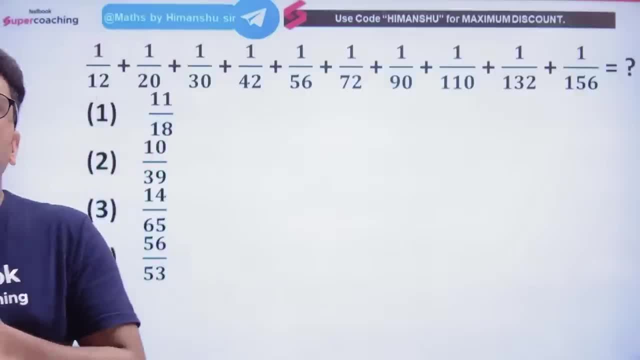 Answer this question. Tell me what the answer will be. All right, All right, Along with the beat. See, one kid is listening, the other one is reading. All right, All right, Okay, Okay, Okay, All right. 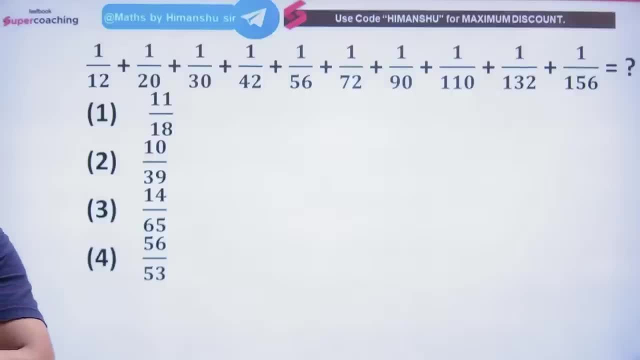 All right, All right, Okay, The one who is listening. Look the one who is reading. You are listening to the earphone. Listen to the earphone. That is what is there in the ear. 1 divided by 12 is 12.. What can you say about 12? 3 times 4.. What will you say about 12? 3 times 4.? Say yes or no. 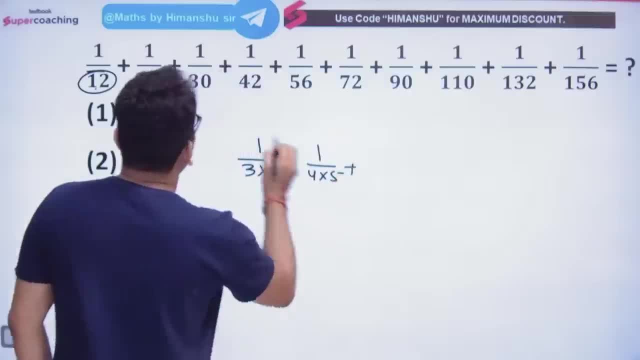 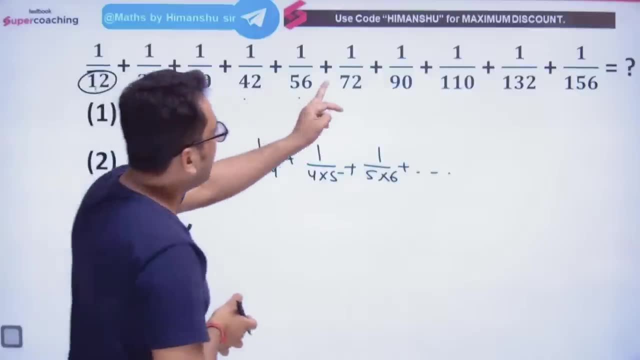 Okay, sir, What will we say about 20? 4 times 5.. Okay, sir, What will we say about 30? 5 times 6.. Means, we have caught the pattern. We have caught the pattern, So 6, 7,, 7,, 8,, 8,, 9,, 9,, 10,, 10,, 11,, 11,, 12,, 12,, 12, 13.. 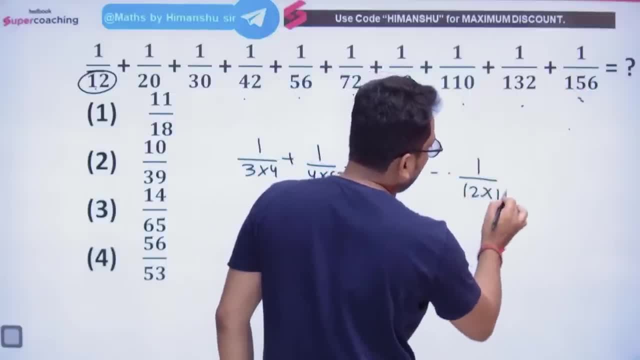 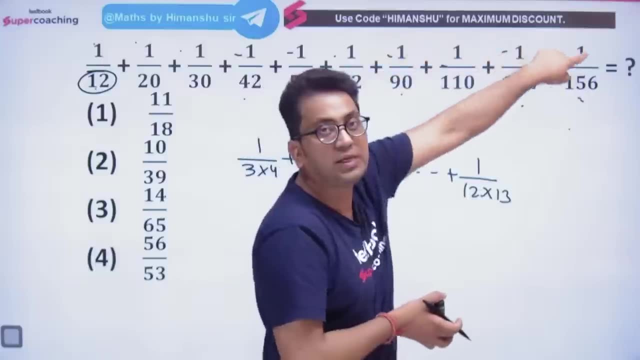 What is this, sir? This is 12, 13.. So 1 divided by 12 times 13.. Do you understand what I am saying? Now see how many are above 1? So 1,, 2,, 3,, 4,, 5,, 6,, 7,, 8,, 9,, 10.. So this time, 10 will come above What will come above 10.. 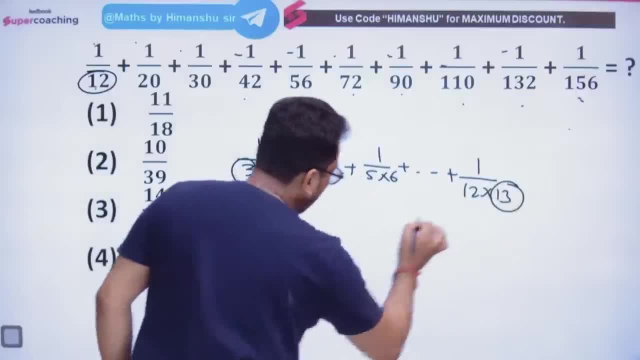 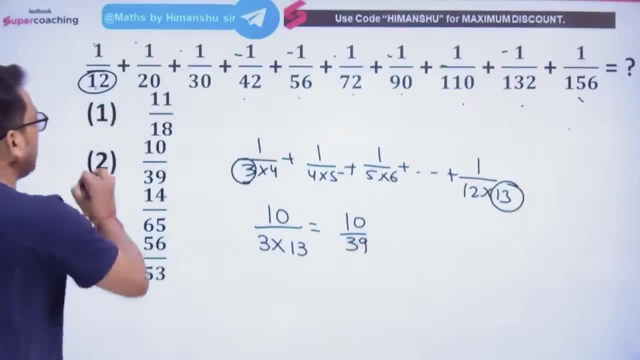 What is the first line below 3.. What is the last line below 13.. So do this son? Do you understand what I am saying? The answer will come: 10 divided by 49. Means, 10 by 39. Means. we have 2 options. 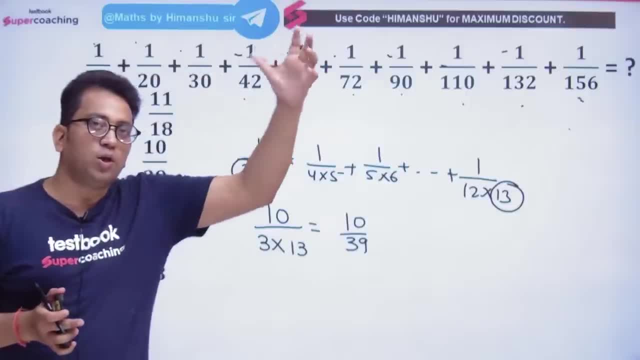 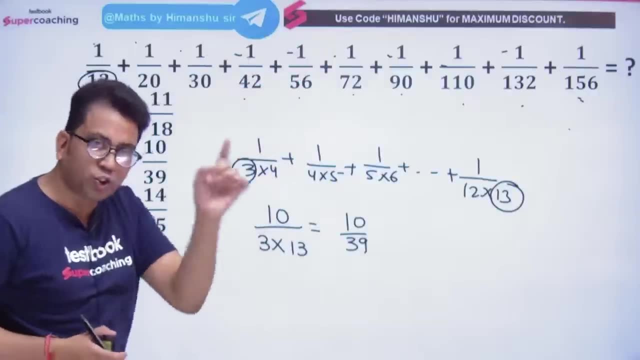 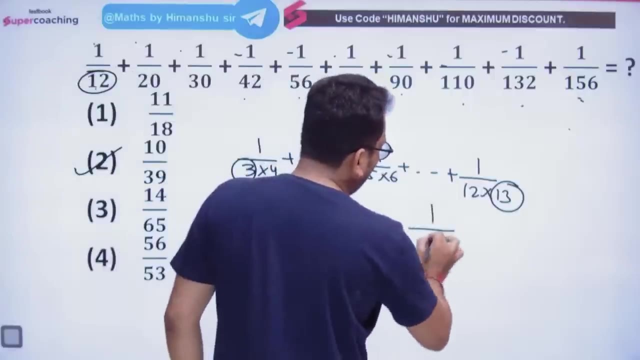 Do you know that the big books like RS Agarwal and other big publications, I will not give names? The shortcut given to you is also given in such a way that the child can make a mistake. The shortcut is such that here comes 1 by difference and in the bracket 1 by first line. 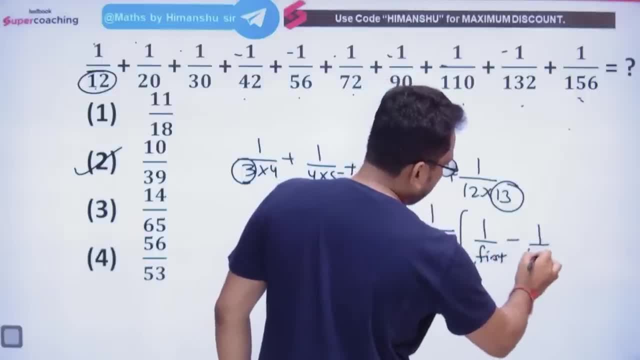 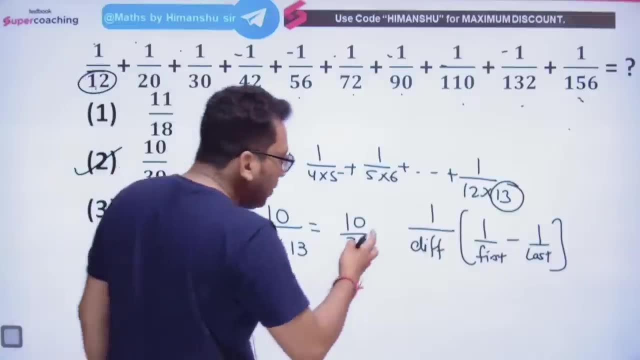 Means. here comes the first term and then in minus 1 by last term. So in this way they have given this formula Okay. But sometimes the child makes a mistake here too. But he will never make a mistake here Because he doesn't have to do anything. He doesn't have to do anything here. 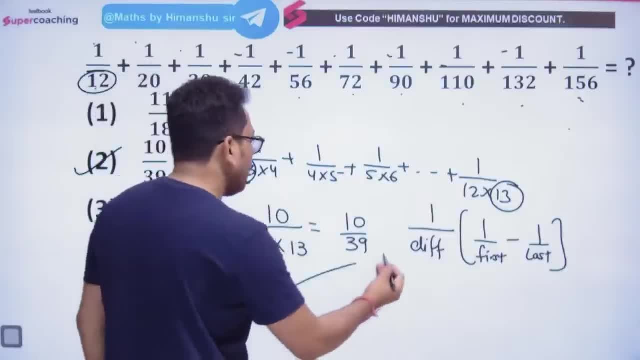 So he made a mistake. The mistake becomes absolutely zero. So you do like this. Do you understand what I am saying? So the things that I am telling you will not be found in any book, son, Because I bring these things for you, except from these concepts. 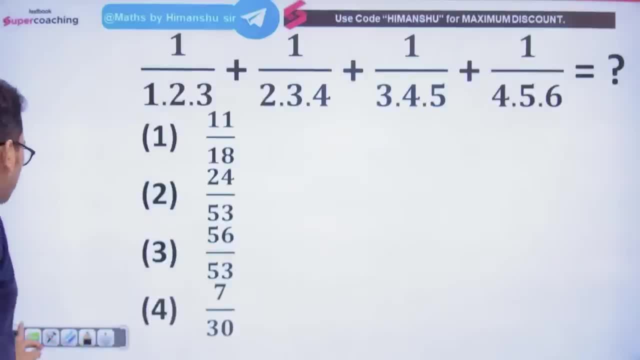 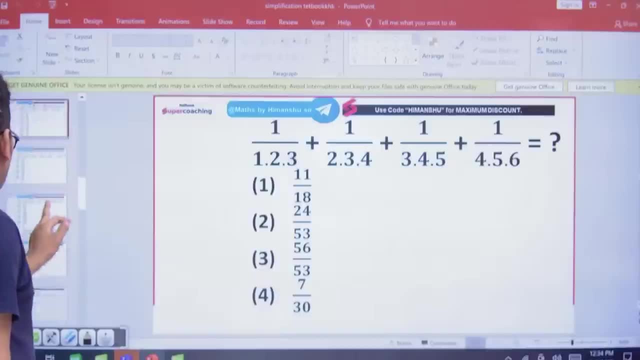 Okay, So the next question is coming in front of you Quickly Now on this question. So now I am skipping this question Because for this first I will tell you the concept. Okay, You come to this question. Come to this question, Do it carefully. 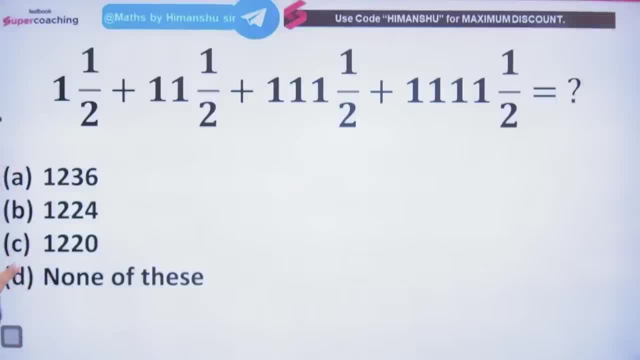 Do it carefully. The first question is in front of you. It is a very easy question to do carefully, And the same questions will be made in your elementary Maths. son, Quickly tell me what will be the answer. All of you Answer it. 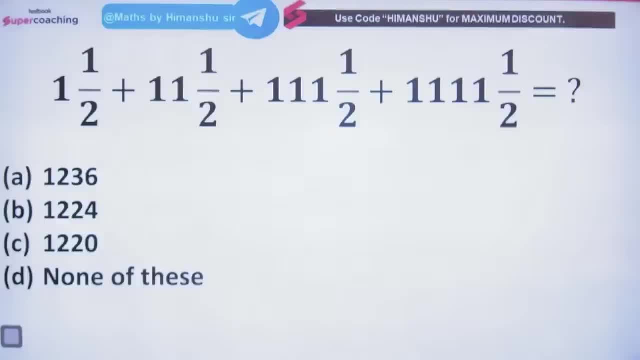 Come on Nikhat, Come on Aarti. Pratima, Manisha, Lakshmi, Right children son Answer it: Ahaan, Rajput, Subhadra Pratima, Richa With Peetha. 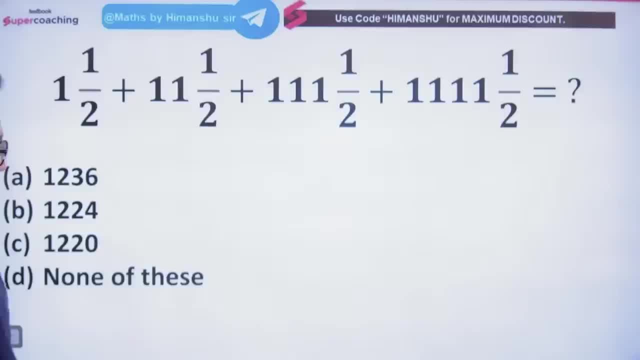 Okay, Okay. One child is saying: Just take the name of the publication, We will take it. Oh, son, What I meant to say was that the things that I am telling you will not be found in any book. Okay, Okay. 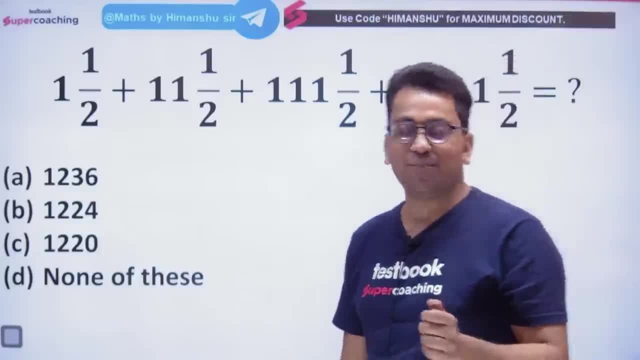 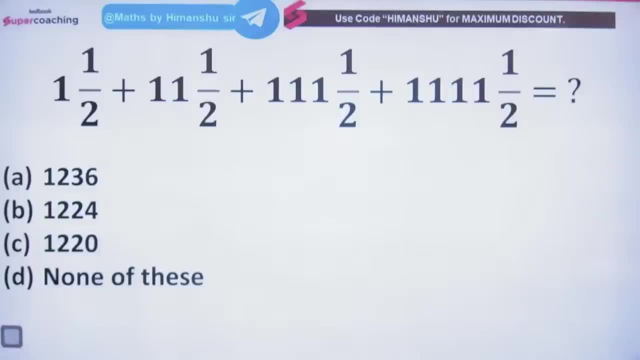 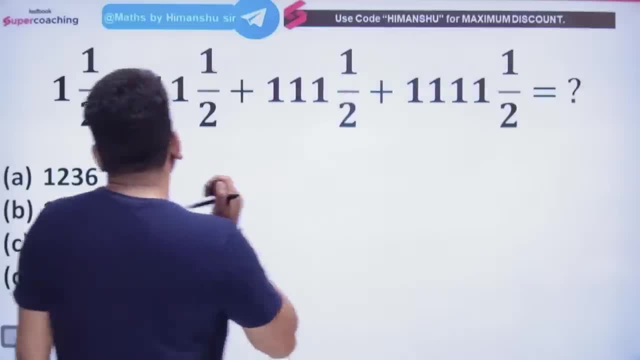 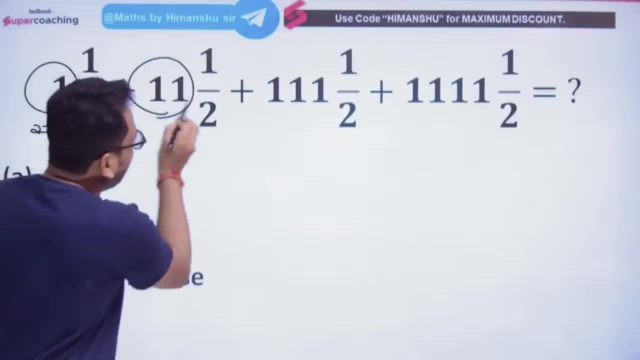 See, We have to connect this Now. how will we connect? Understand This next number, which is next to the number. Connect these next number together. Do you know what he says? We are together. Let's connect together, Brother. 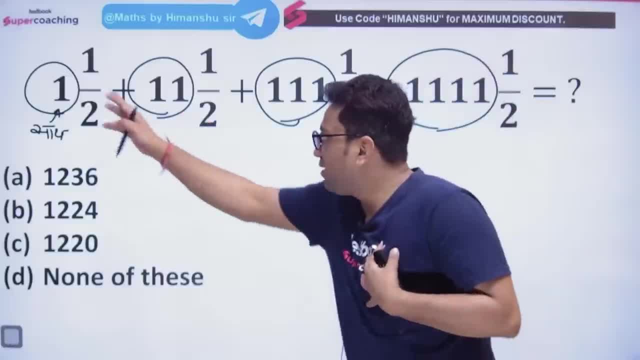 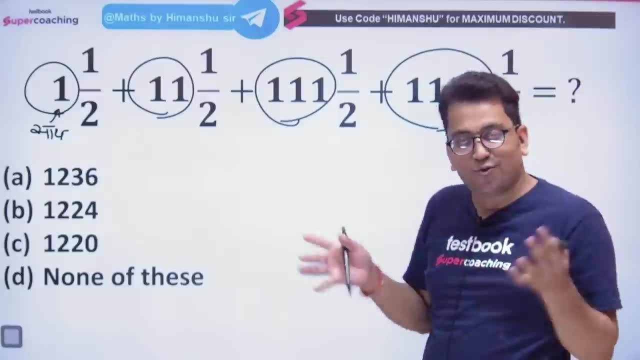 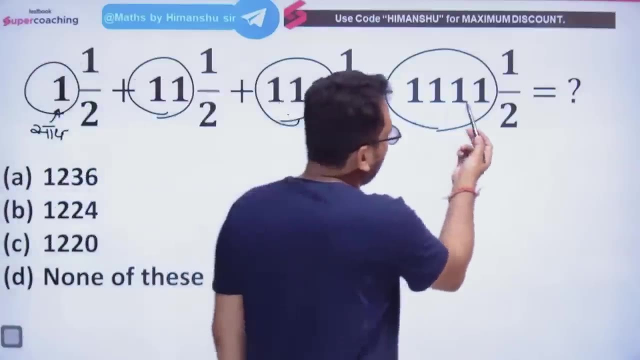 We are connected together. We are looking different, but we are together because we are attached to each other. All these people are doing the stick movement, so stick them, Stick them all. What do you say? You stick, That is, stick them all. 1, 11,, 111,, 1111,, stick them all. 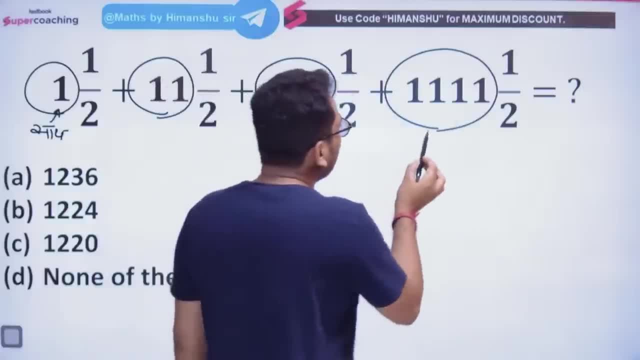 How to join. Learn to join directly. You just see how many times it is written in the end: 4 times. How many times, 4 times? So you take it from 1 to 4.. 1,, 2,, 3,, 4.. 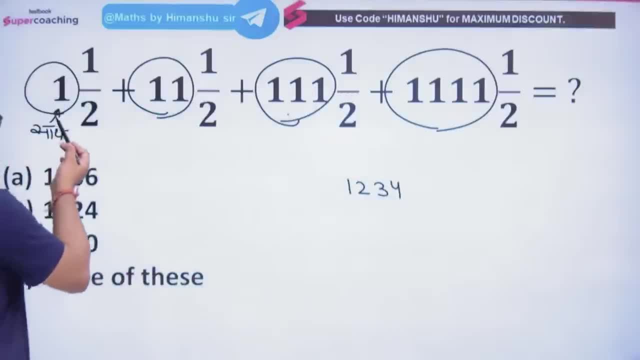 It is joined. It is joined. There was nothing. 1 time, 2 times, 3 times, 4 times was the maximum. So you wrote that 1, 2,, 3, 4 is joined. Now you just have to join them. 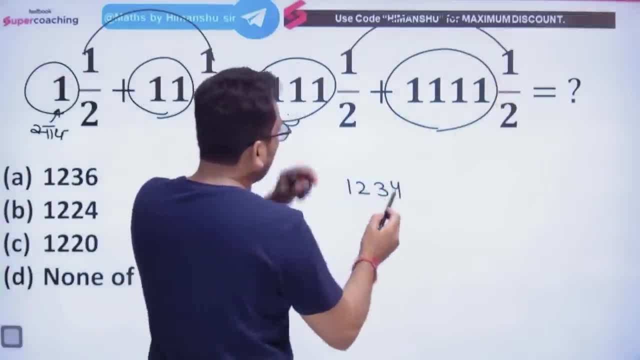 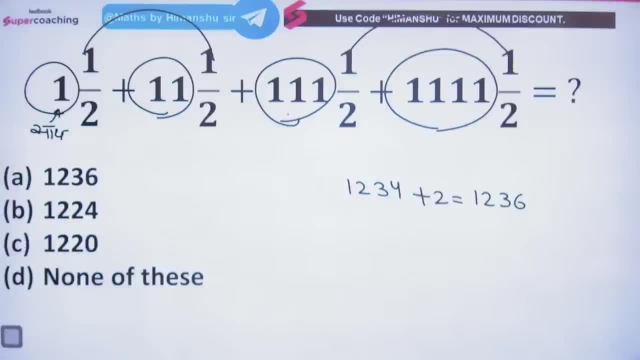 Half half 1, half half 1, 1 and 1, 2.. So join them separately And when you join them, our answer will be 1236.. I think every child will be able to answer. 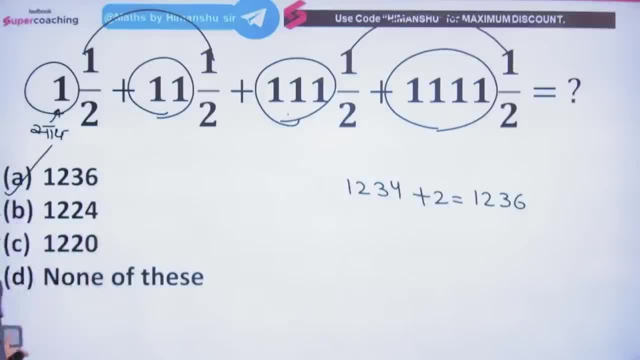 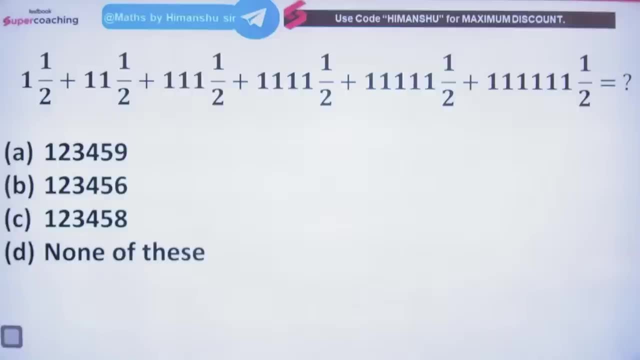 1236, that is, our answer will be 1236.. Next question: The next question is coming. Tell me quickly what will be the answer. The next question is in front of you. Let's see how many children are able to answer. 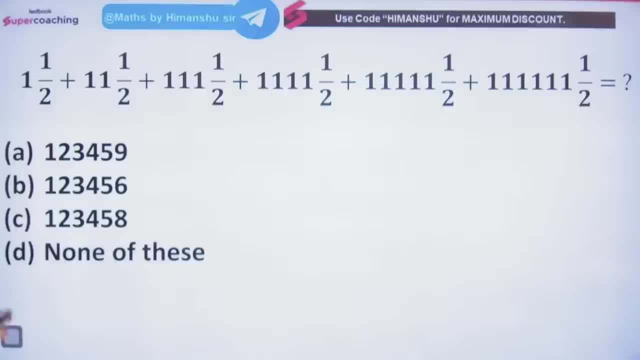 Answer. All of you Answer: Son, tell me what will be the answer. All of you answer: Come on, Come on, tell me quickly what will be the answer. The question is in front of you. Answer with speed. I will want the answer from every child. 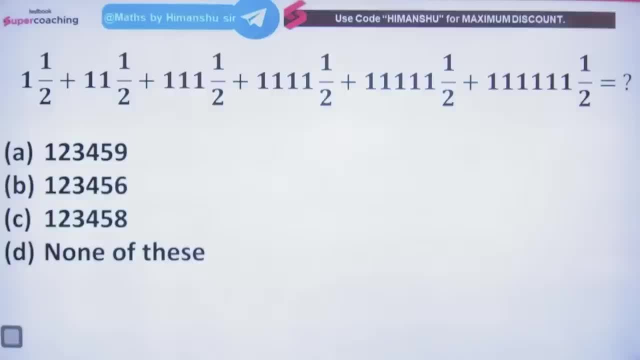 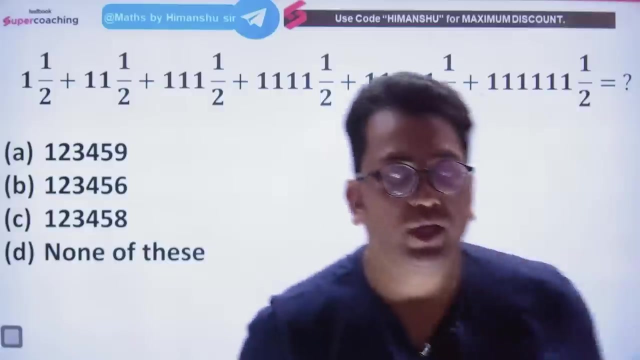 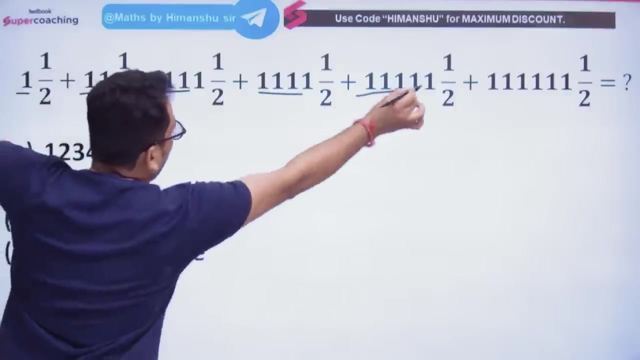 Tell me what will be the answer. All of you are able to answer. All of you are able to answer. Okay, very good, Son. if we come to the question now, what would you say? that these seven together? we have to join them separately, right? 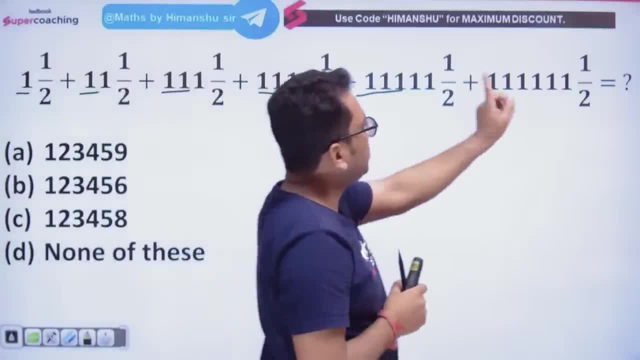 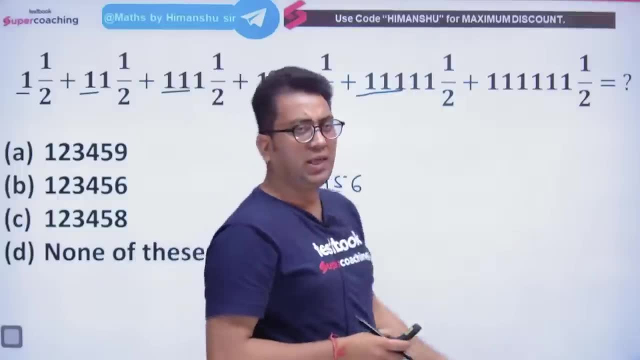 So look once twice, three times, four times, five times, six times. So write 6 times like this: 1,2,3,4,5,6. Not like this. We will join like children. No, no, no. 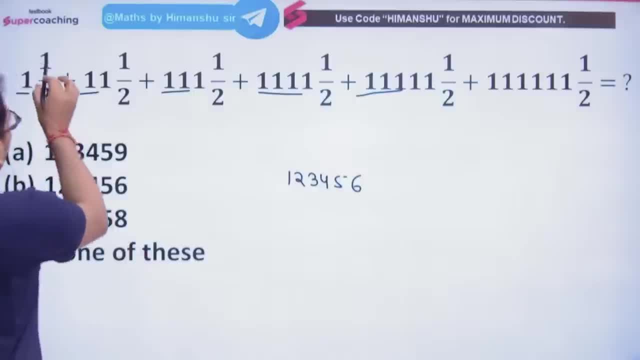 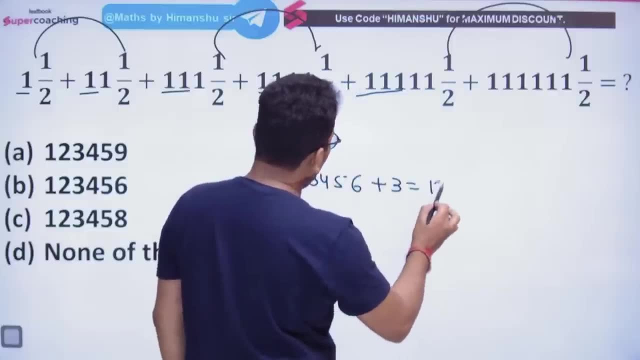 We will write like this: Now, the child will join half and half Half and half 1 Half and half 1 Half and half 1. So 1 and 1, 2 and 1. How much will it be? 3 will be. So what will be the answer? 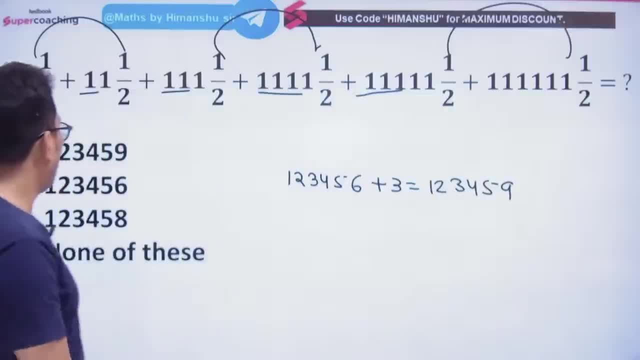 1,2,3,4,5,9. 1,2,3,4,5,9 Means our solution A is the correct answer. The answer of all the children who are doing 1 is correct. Next question. Next question is coming. 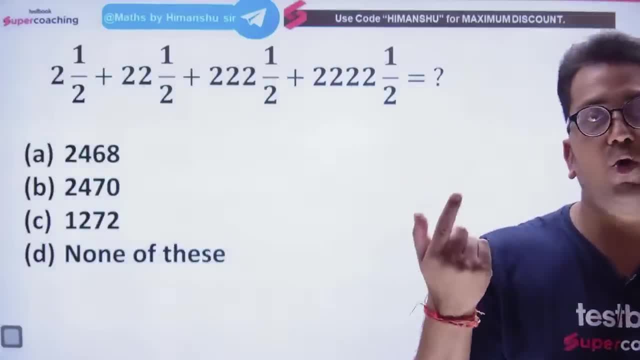 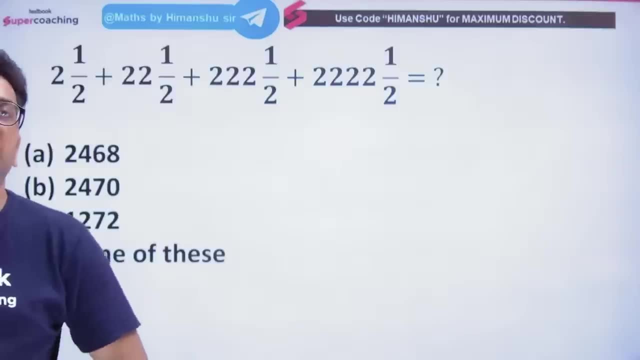 Read carefully Now. not 1 Here. 2 is given to you, Ok, Not 1. How much is given? 2 is given. Quickly tell me what will be the answer. Answer all, Come on, Listen carefully Now. say this question Now. the second answer is 2. 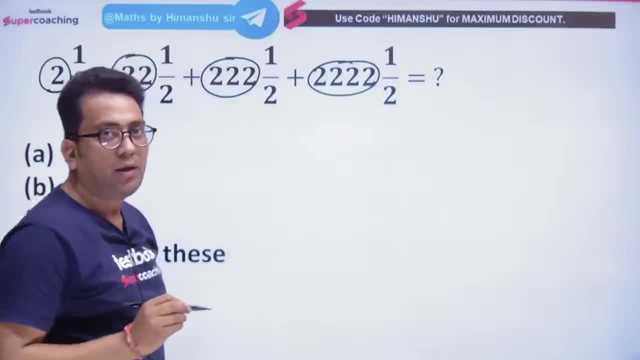 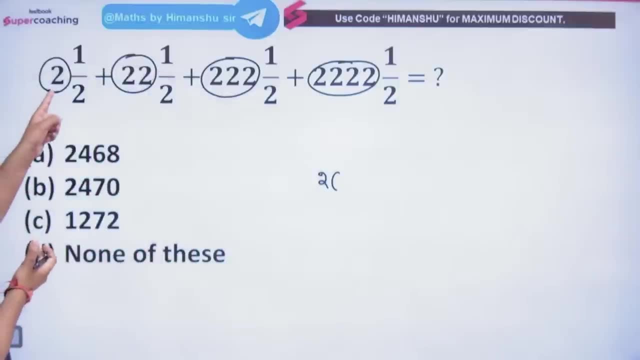 Now 2 is written, 2. Now what do we do? Take 2 comma from here. When 2 is taken as a comma, Do you know what you will see inside? 1, 2, 1, 3, 1, 4 times 1? 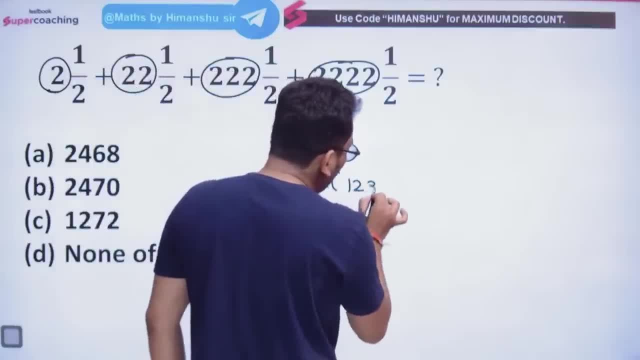 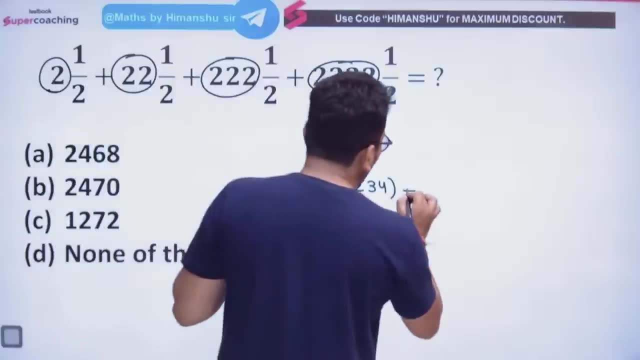 So when you add them, you get 1,, 2,, 3, 4. You know how to add 1 And you have taken 2 as common. Now what else do you add? Half half 1, half half 1. 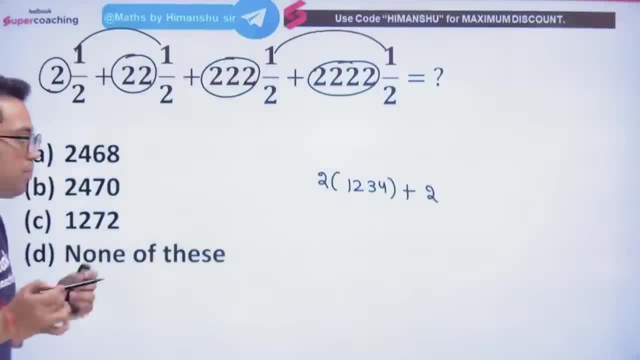 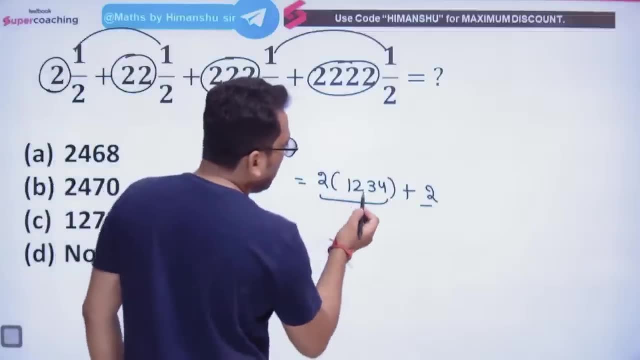 So 1 and 1 is equal to 2, So you can understand this much. Now do not do anything. Multiply by 2 and add 2. Do you understand what I am saying? Multiply by 2 and add 2. So look: 4 times 8, 2 times 6, 2 times 4, 2 times 2. 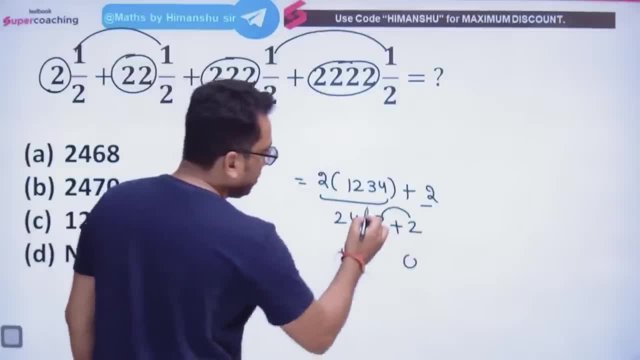 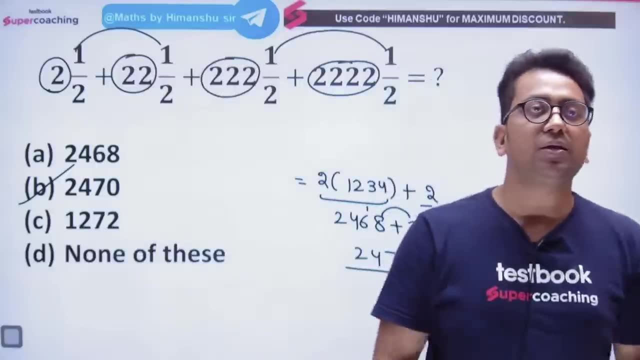 And add 2 to this. So what will be 8 and 2? 10? You got 1, 7, 4, 2, 2, 4, 7, 0, So our answer is absolutely correct. The children who are answering B: their answer is absolutely correct. 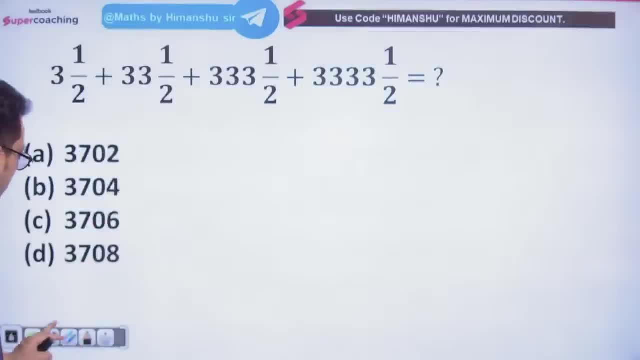 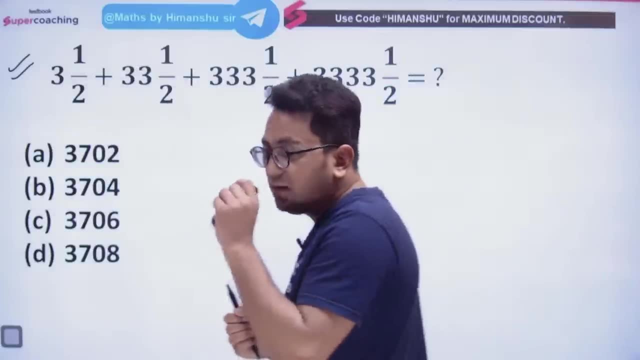 Let's move on to the next question. The next question is coming in front of you Now. what did he give? He gave 3. Tell me quickly what will be the answer? Shine every child answer. Then I will tell you a very good concept, Okay. 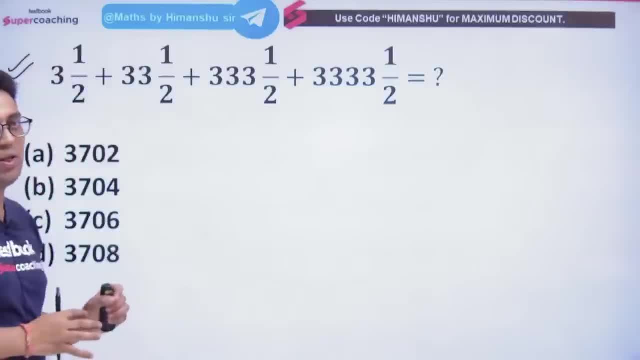 Now the question which we skipped. Now I am going to come to the same question. Okay, first answer this question to all of you. Tell me what will be the answer With speed. What will we do here, son? We will take 3 as comma this time. 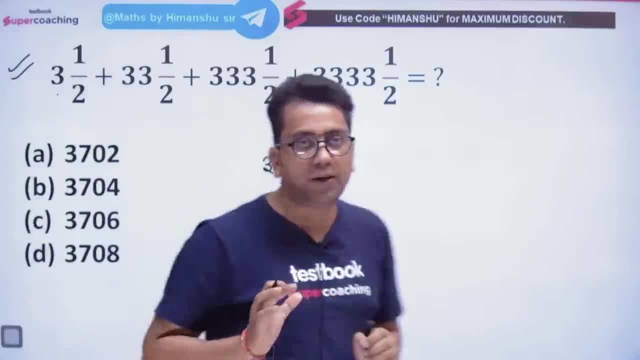 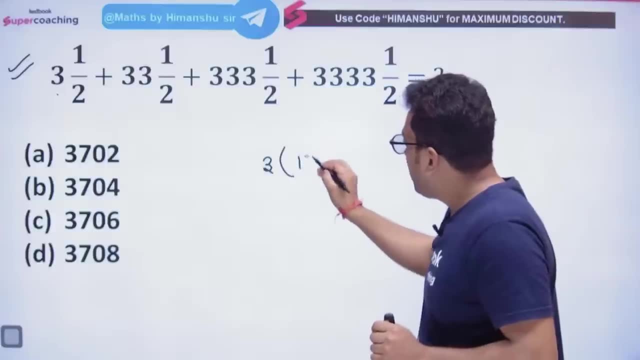 So when we took 3 as comma here, So what will be left inside you? 1,, 2,, 3, 4 Will be left like this: So you have to add them. So you have to add them: 1,, 2,, 3,, 4 will be left. 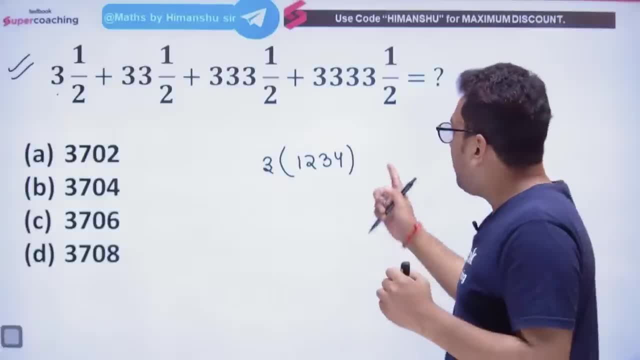 Because 4 times 1 came, So you have to add them: 1,, 2,, 3,, 4 came, Isn't it? Now 3 will be multiplied. And what will you add? Add them Half, half, 1. 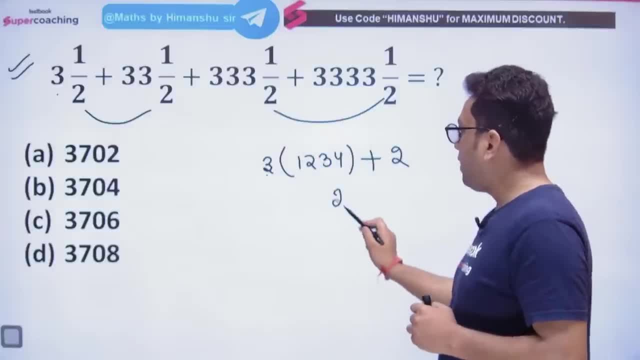 Half half: 1, 1 and 1, 2, So 3, 4, 12 Got 1, 3, 3, 9 and 1, 10 Got 1, 3, 2, 6 and 1, 7. 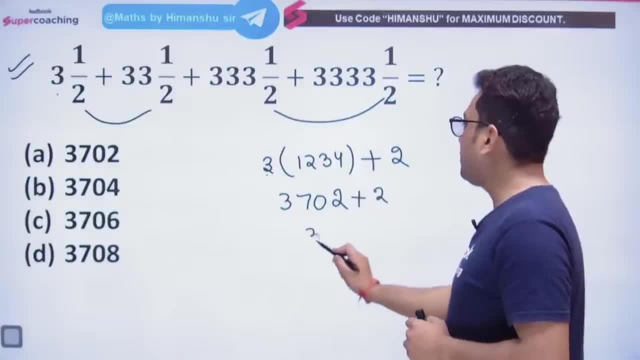 3, 1, 3. So add 2 in this. So the answer will be 3, 7, 0, 4. Is it clear? So, children, are you able to answer B? Everyone must be getting B answer. 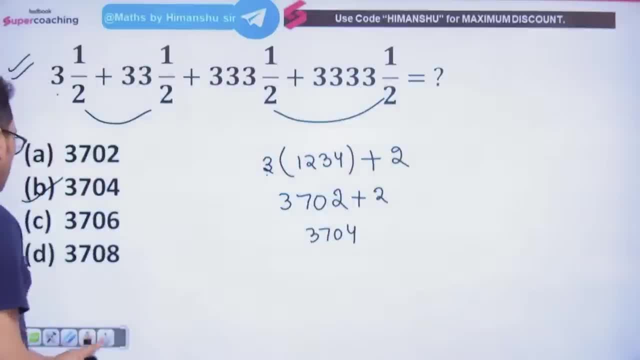 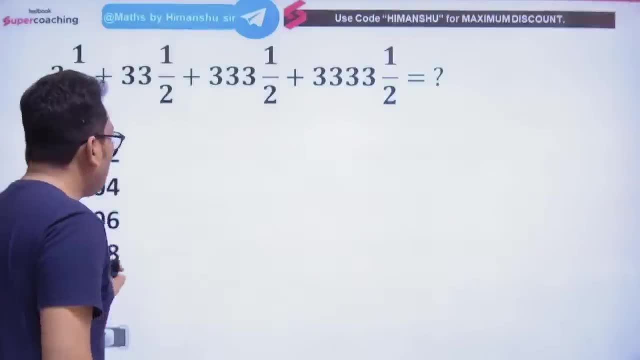 Very good, Very good, Let's move on to the next question. The next question is coming in front of you. The next question is not here. The next question is the torture. But before coming to the torture, Before coming to the torture, I would like to come to that question. 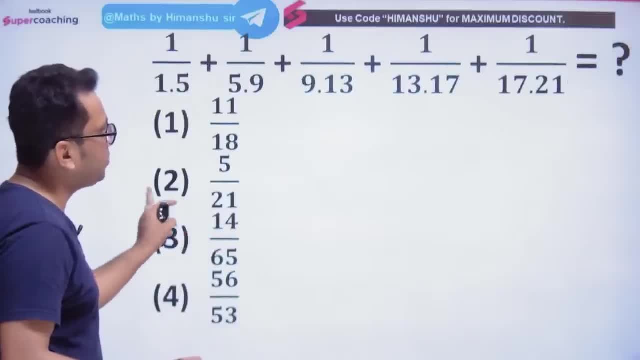 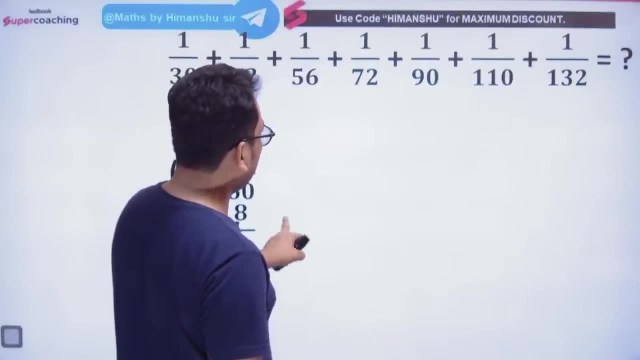 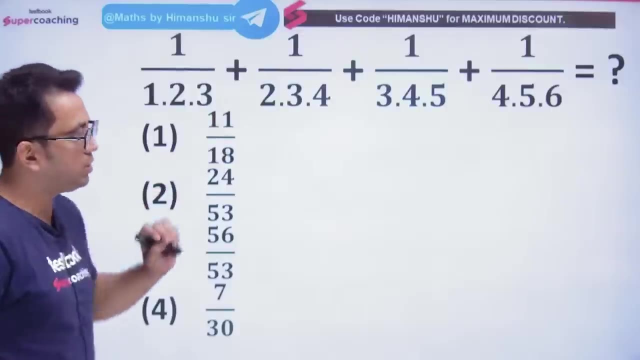 It will be punished. We will see its torture too. But before coming to that question, I would like to ask you this question, Because this question is also important for you. Where did it go? Here it is. Hold on This question. Understand this question carefully. Understand this question carefully. 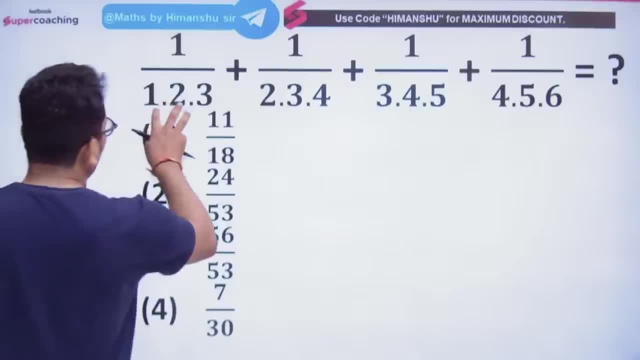 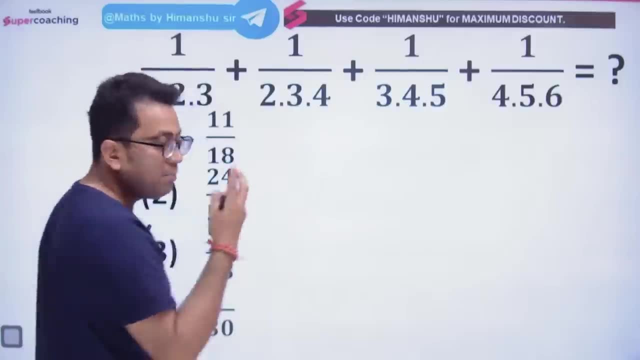 This is the question. You must have understood the dot. That is the question. This is the multiplier. Okay, Now see, I can't do this in that way, Because there are not two numbers here, But there are three numbers here. What is the number? There are three numbers. 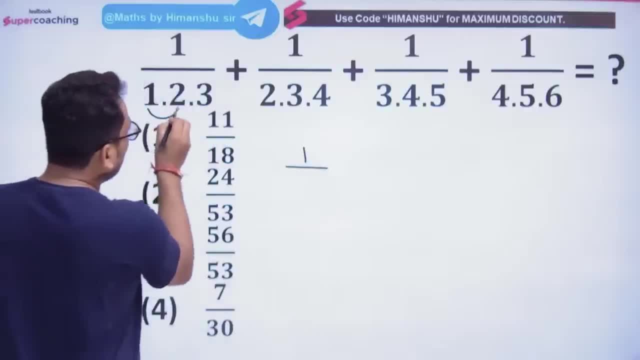 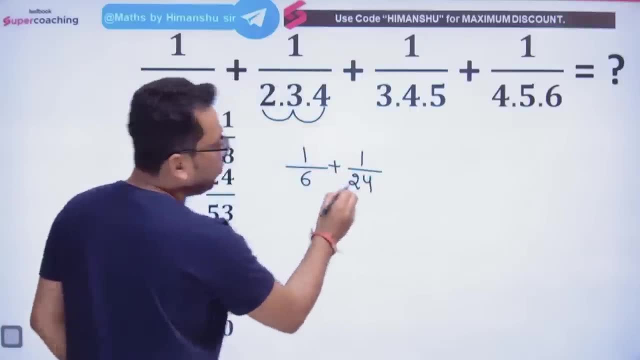 Now see how will you do this When I solve it child. So 1 times 2, 2 times 3 Means 6, Plus me Here, 2, 3, 6, 6, 4, 24. First I will tell you. 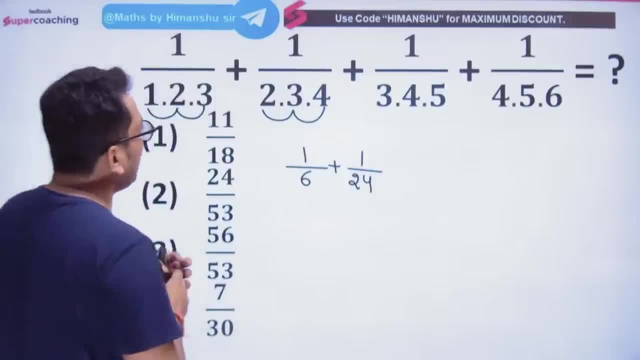 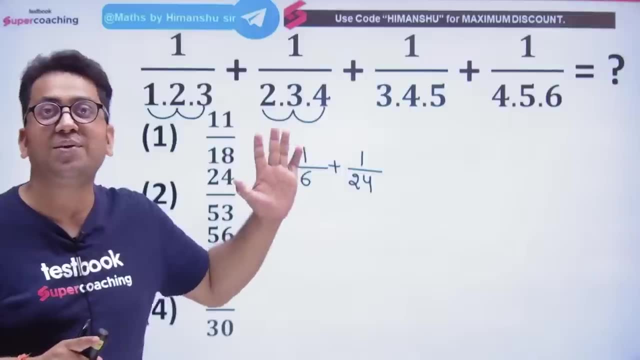 The traditional way, Conventional way. Then I will tell you How do you see this question, How to find the way to find it, And what I am telling you. The way to find it, You will find it only here And you will not find it anywhere else, Because I have solved it from the concept. 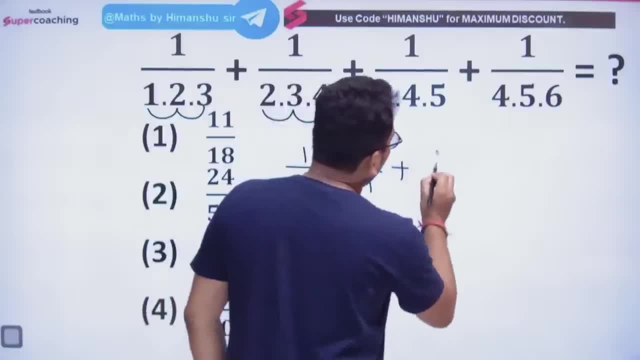 Now understand this child. So this 1 times 24 will come Here, see, this will come. You have 3 times 4, 12, 12 times 5,, 60 And here, if we do 4 times 5,, 20. 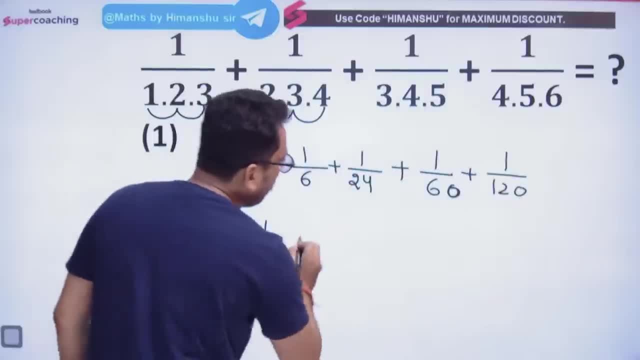 20 times 6, 120. Do you understand what I am saying When I take them LCM? So 6 times 24,, 60,, 120. LCM of 120 came. I will run from 6, It will go to 20. 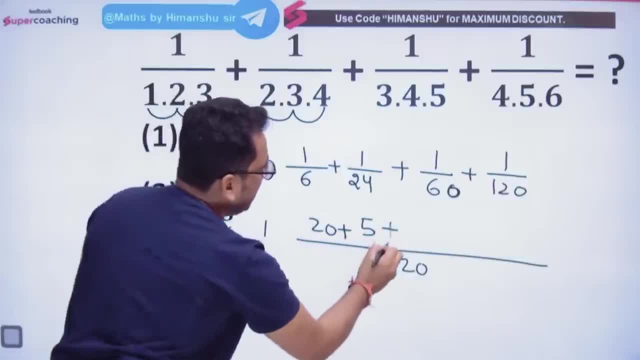 20 came up 24 times. 5 will go here on 5, 60 times. 2 will go here on 2. And there it came. 1. Are you able to understand this much? Now, if we add them up, then 25 and 20 will come. 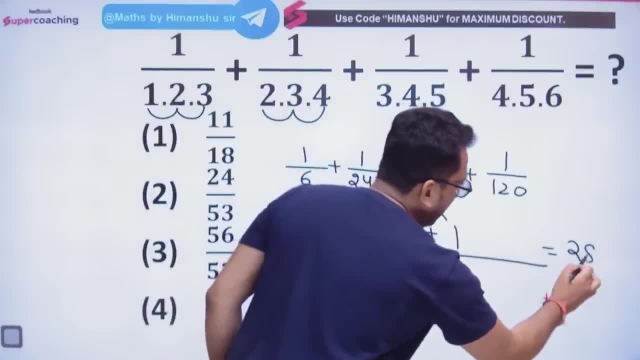 2,, 27,, 27 and 1. How much has come? 28? So 28 divided by 120 is coming. How much is coming 28 divided by 120? Let's cut from 4, sir, If we will cut from 4, 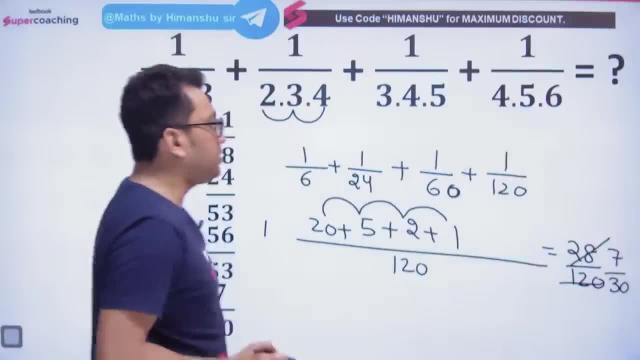 4 times 7 is 28 If we will cut from 4. So 4 times 3 is 12, Means 7 divided by 30. Means 7 by 30 is our answer, Which we are seeing as option number 4. Do you understand what I am saying? 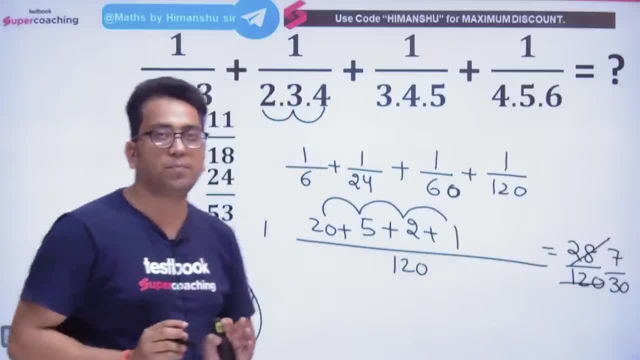 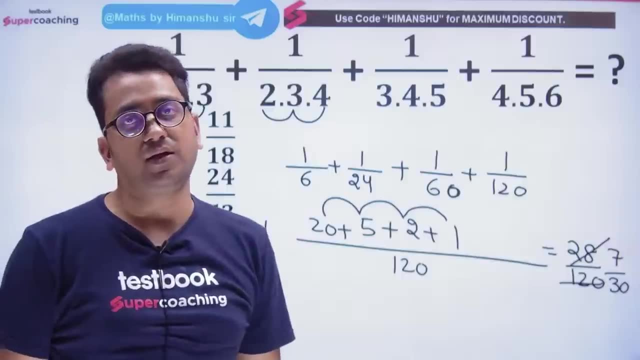 So what we have done is We have solved it all in this way. Ok, sir, If number was 4, then we have solved it. If we had given further, Then will we keep solving like this. No, sir, No Brother, it is the era of 5G. 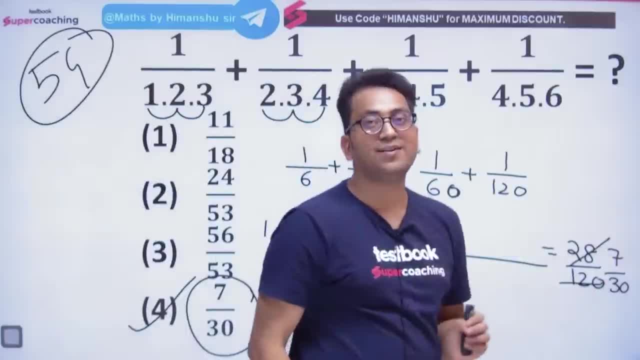 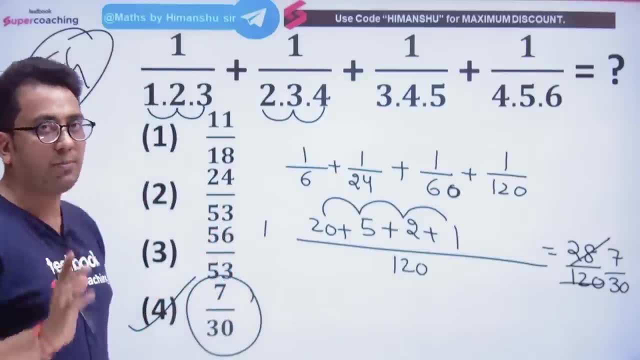 Yes And sir, we are on 1G, How We have to give speed to the solutions of the questions, So you should know the way to make it shine, How to make it shine Now, understand my words carefully, Which I am going to explain to you. 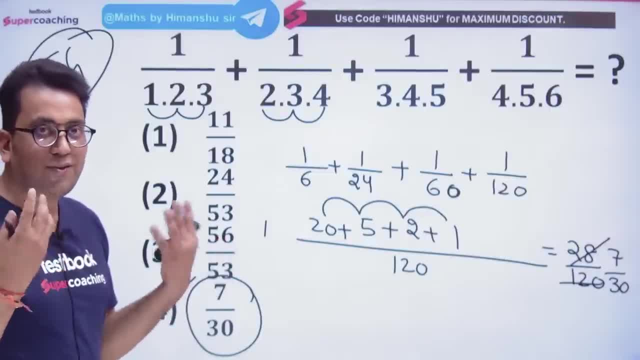 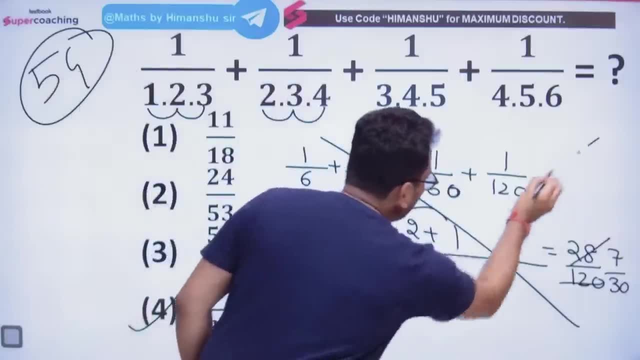 Ok, Are you all ready? How to make it shine? So come here. See what you have to do. I will remove this Means. you don't have to do anything. You just see the end. See the end, The last one, The last one that you see. 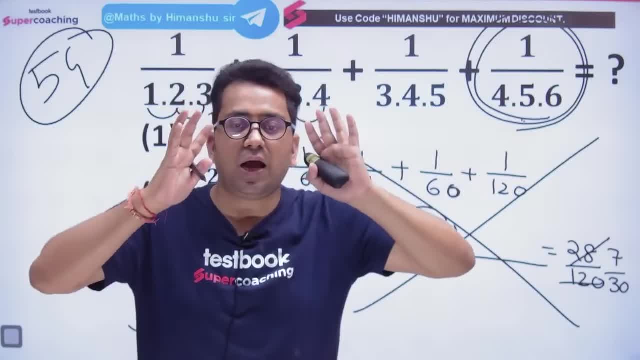 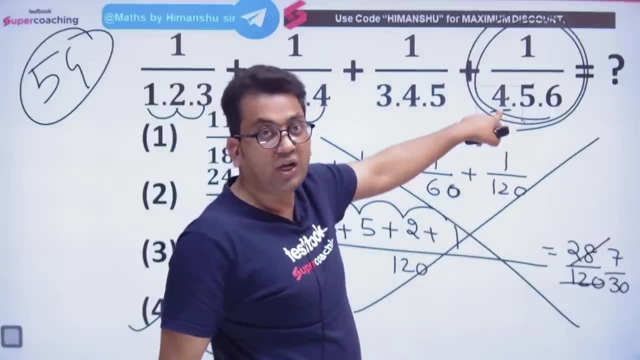 Come on this. What did I say? The last one that you see. Just come on this And listen to what I am going to tell you. You pick this. What has it given you? It has given 4. What has it given? It has given 4. 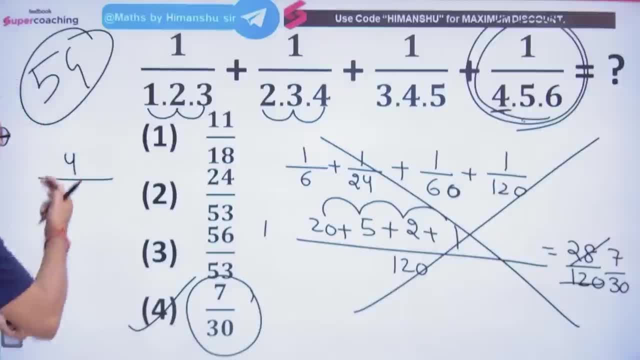 You pick this 4. Keep this 4 up. Ok, Now tell me What comes after 4?. What comes after 4? 5, 5, What comes after 5? 6 And what comes after 6? 7 Means it will go up. 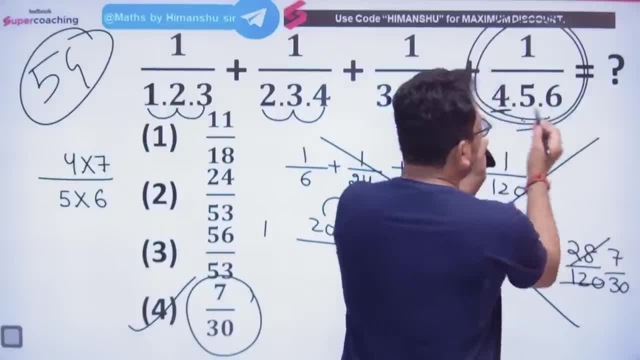 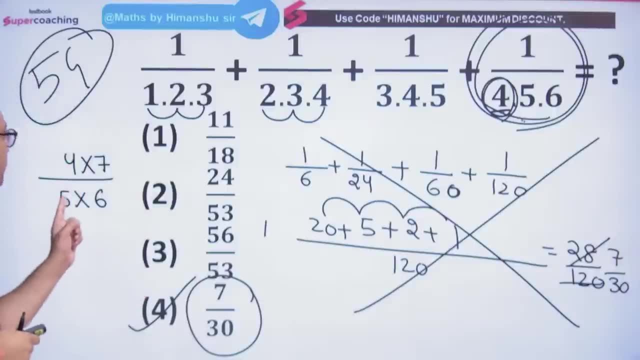 Let me explain again. You see, this last term, The last term that you are seeing. What is the first term here? 4, Pick up 4, Put 4 up. What comes after 4? 5, Then what comes after 5? 6, Then what comes after 6?. 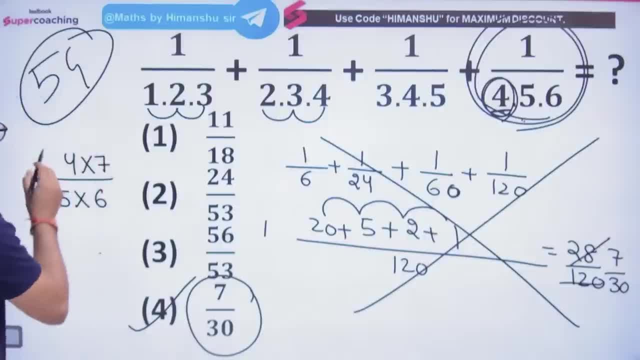 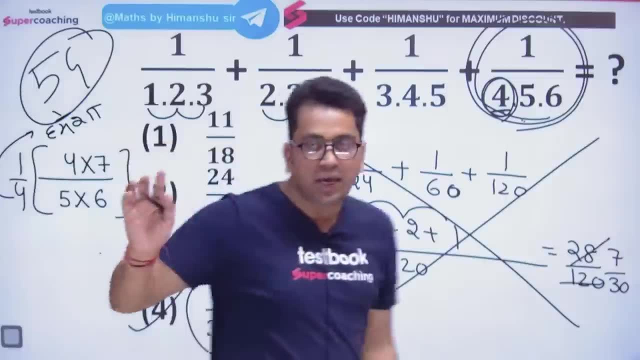 7 Means 5 times 6 down. The next term that will come, It will go up And always, Always, you have to divide it by 4. Always, With whom to divide With 4? You will have to do this And your question will be clear. 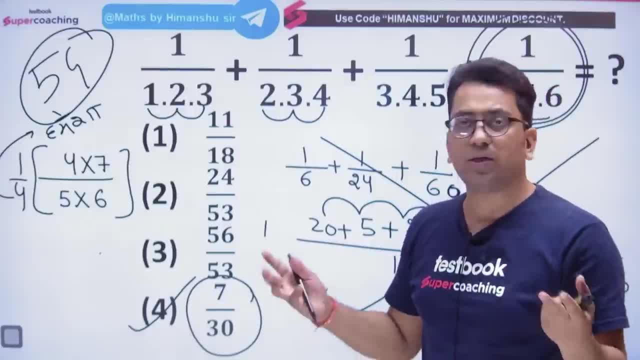 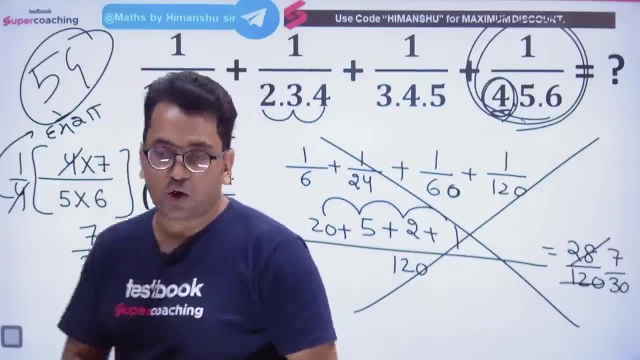 You will get your answer. You will say, Sir, how? You will say, Sir, how? See, 4 to 4, 7 up And 5 times 6 is 30 Here, Tell me, Is black magic happening? See, It is happening, Isn't it? 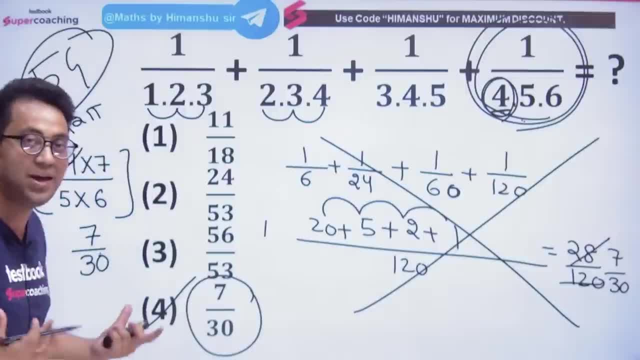 In the beginning of our session. Black magic happened When fashion was not going, So we will also do black magic. See: 7 divided by 30. See, The same answer is getting. Which was there? Is it getting or not? 7 divided by 30? Our answer. 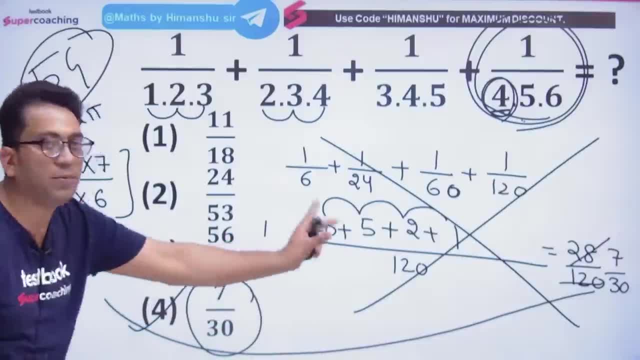 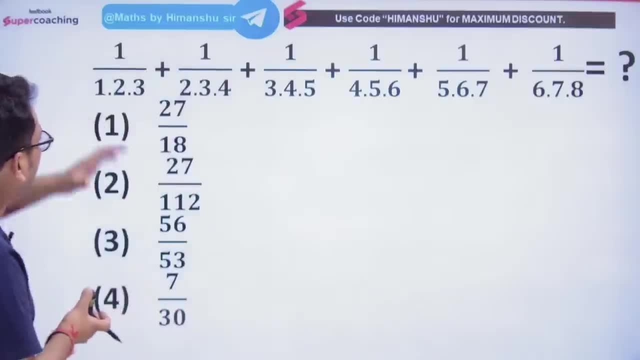 Is it clear? I can understand. So 7 by 30 Will be the right answer, Sir. This thing, We can apply this thing everywhere. Yes, my dear, You apply here. Your answer will be correct. Look at this question carefully. The thing I have told you, Apply those things. 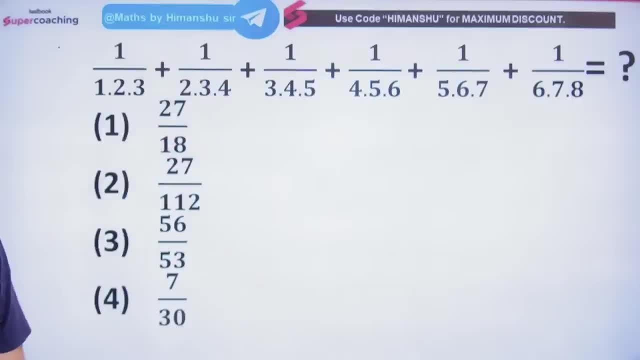 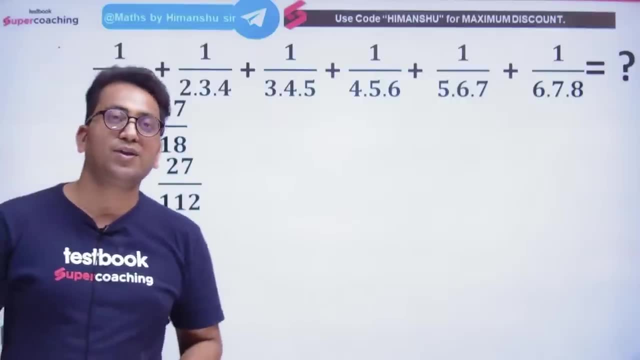 And find your answer. See what the answer is coming, or not, Quickly, Is it going live? Sir Royal Rahul Yaduvanshi is saying: Now, I took your name. Now, more than this, We can't give you a better proof That, yes, This live class is going on. 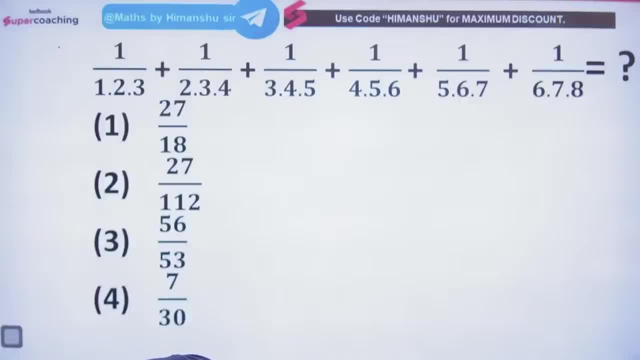 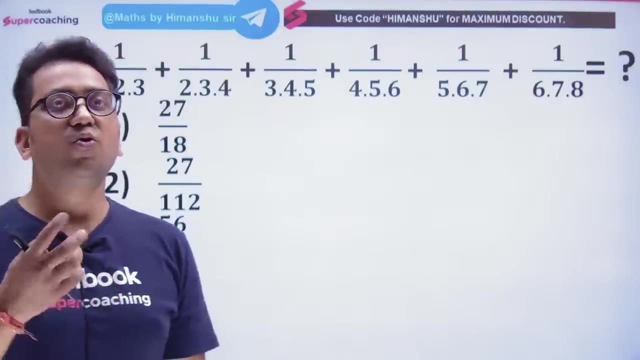 Okay, Okay, tell me quickly What will be the answer. All of you Answer with speed. Pooja Singh is saying: Sir, I am Aarti. I Okay, Okay, I am coming. Okay, I am coming. Okay. Yes, my dear, Come Come, No problem. Samadhan is saying: 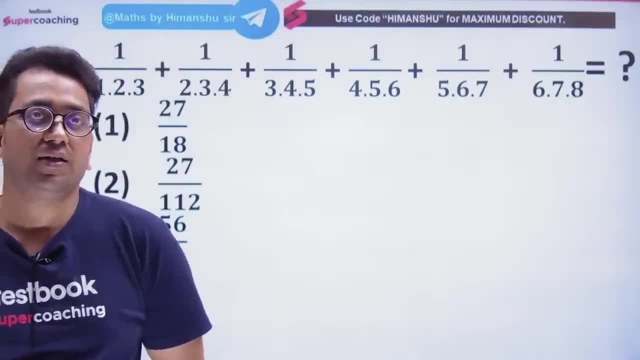 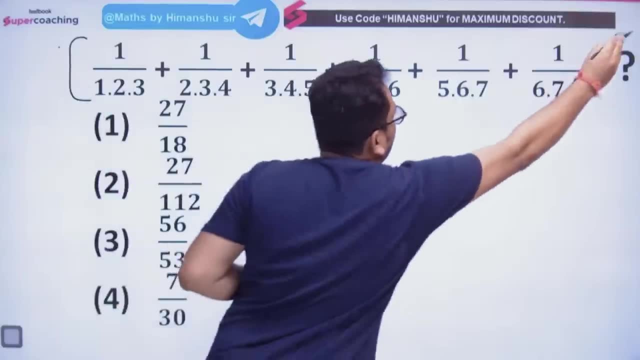 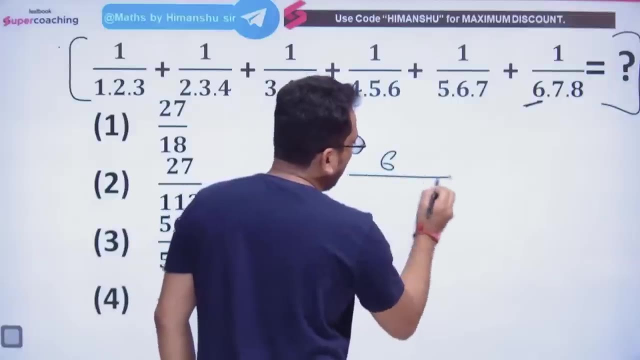 Ghost has done. It will be Sir Black magic. He knows. Come, Come, Come here, Come, Come, Come, Tell me what will happen, What will be the solution. You see the last here. What is six? So you write six. What will come after six? What will come after seven? What will come after eight? 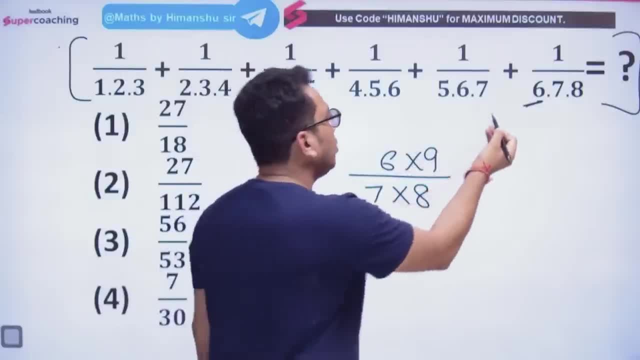 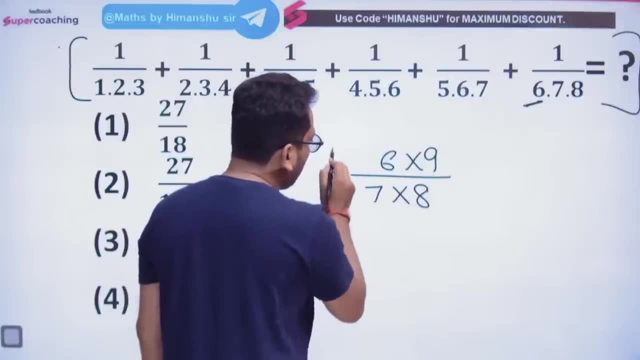 What will come after eight? What will come after nine? Rise nine, Understand my thing. Write six, Six after seven, Eight after eight, Nine after eight And always. Whom will we give a part? To four, Always From four To give a part. This is the day That you have to keep in mind. 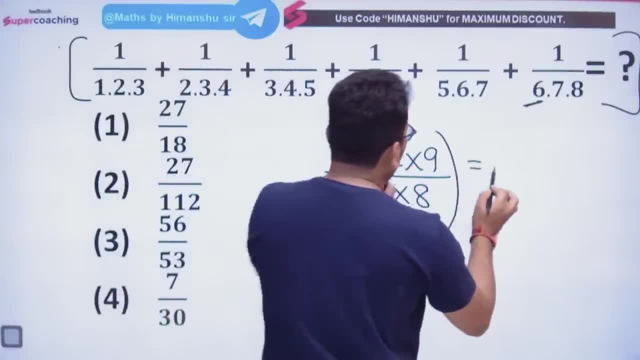 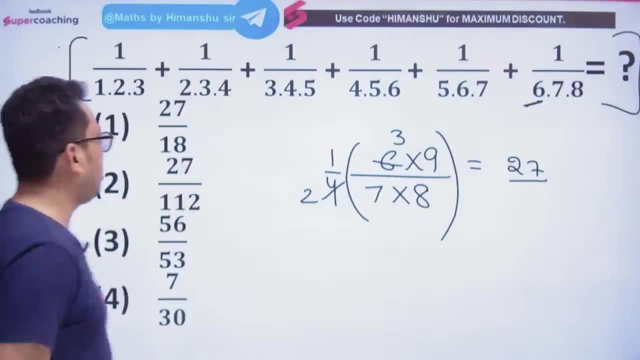 Okay, Now look, We will cut from two, then it will be 27 out of 3. and what will come down? if you multiply 7 by 8, then it will be 112. so 27 divided by 112 means we have 2 options. 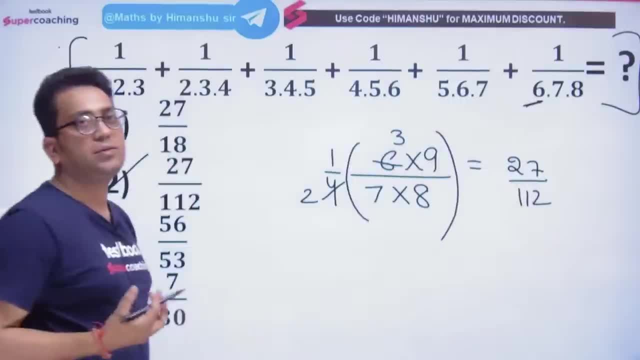 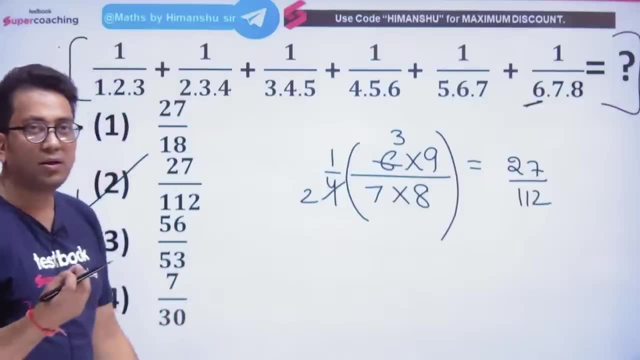 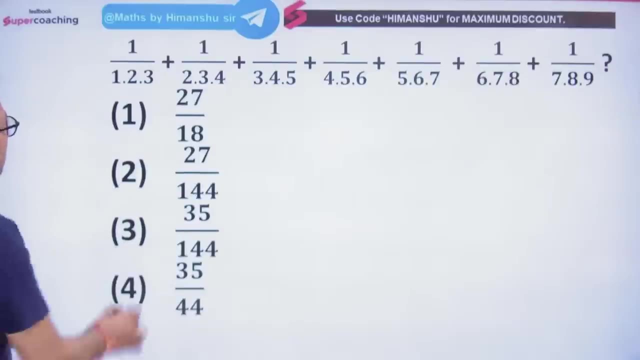 and if you solve this, then also you will get 27 divided by 112. are you enjoying it? are you understanding it? like this? next question? next question: let's see how many of our children are able to answer this question quickly. tell us what will be the answer. 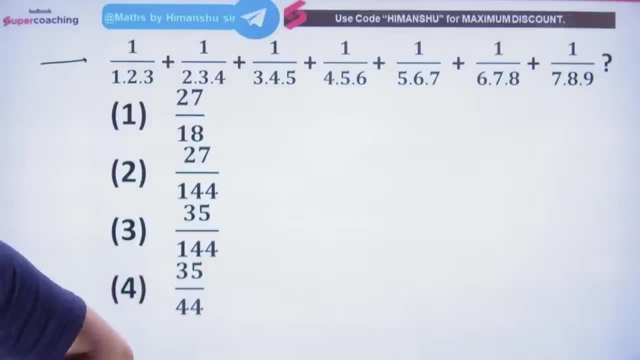 next question is in front of you. answer all of them. Rimpi, Nahid Faiz, Gopal, Jainak, Ankita, Khushboo Reena. how did this slow down in the comment section? catch the speed, let's answer all of them. 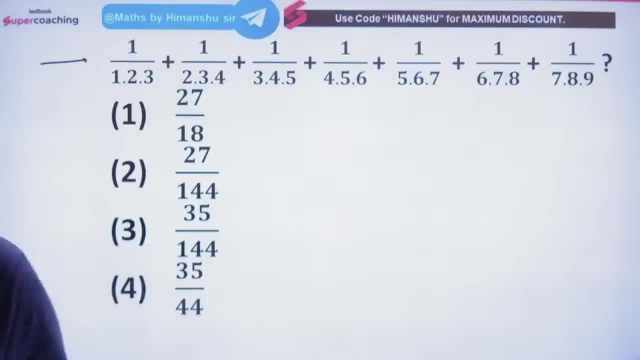 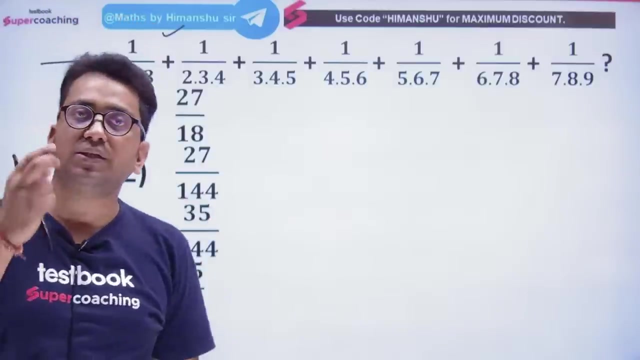 let's go. the child who is still not connected: Maths by Himanshu. sir, connect with this telegram channel. here you will get the link of all the sessions and today, with all of you at 2.15 pm, class will be on this channel with excellent questions. 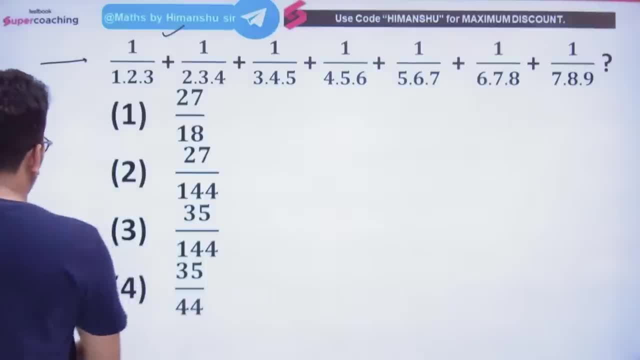 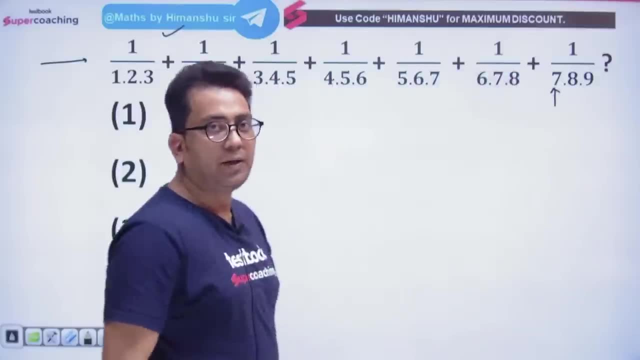 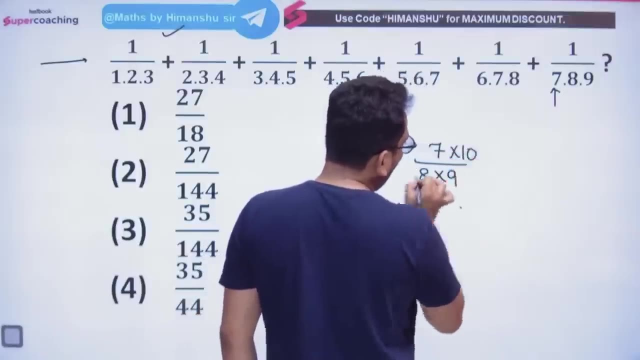 quickly answer this question. what will be the answer? see what you did. these things are going on in this way, so you will catch the last one. you caught 7. pick up 7, 8. what is after 8, 9? what is after 9, 10. 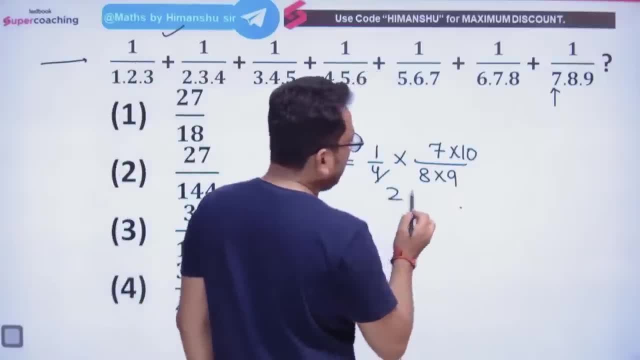 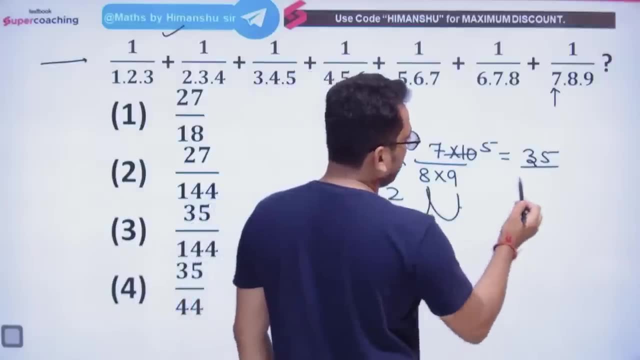 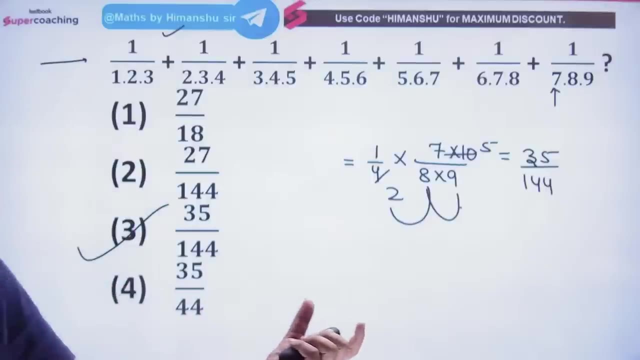 and always divide by 1 divided by 4. who will divide by 1 divided by 4? finished story. see how many are coming: 2 divided by 4. 2 divided by 5. 10, 7 divided by 5, 35 divided by 144. 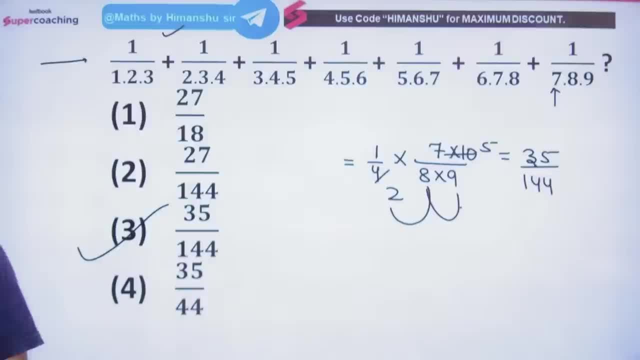 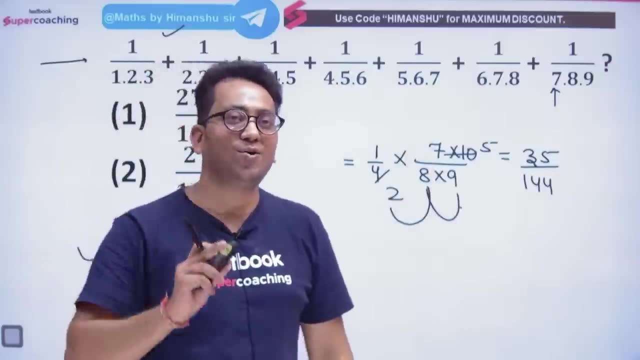 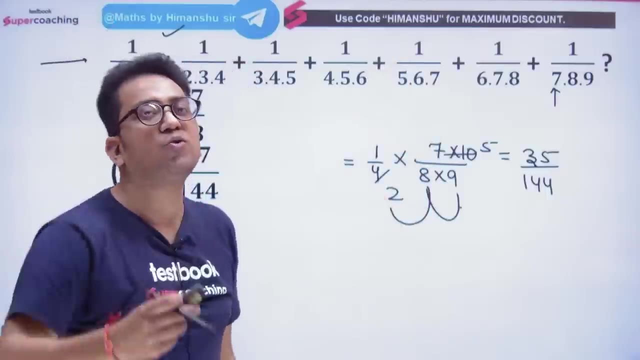 you should get the answer. ok, see, is the right answer. are you enjoying? are you understanding? means such a question the way of shining you have never seen before. are you enjoying, are you understanding? these are very good things, son. it is a mess, but you come and connect. 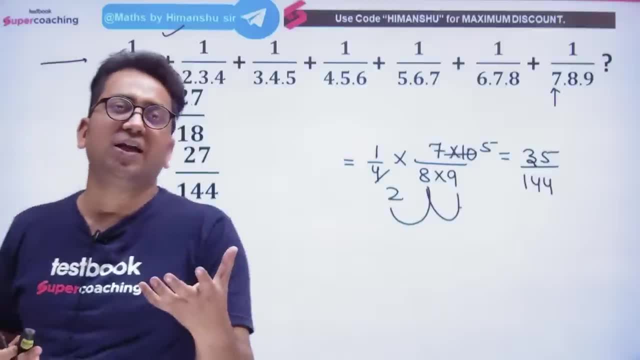 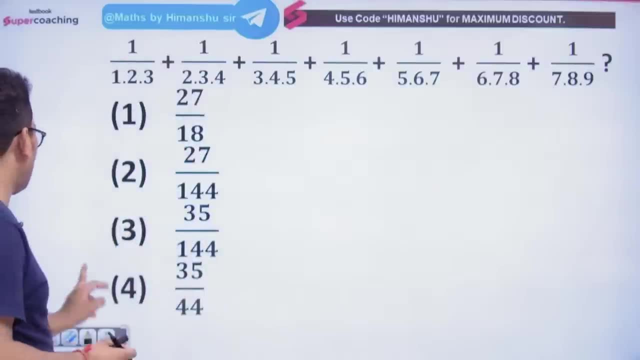 those things which I want to give you, which I want to deliver. let it reach you. ok, it will reach you only when you come and connect with everyone, right? ok, so we had done this question. we had done this question. now. see, brother, the cruel has come. see what the cruel is saying. 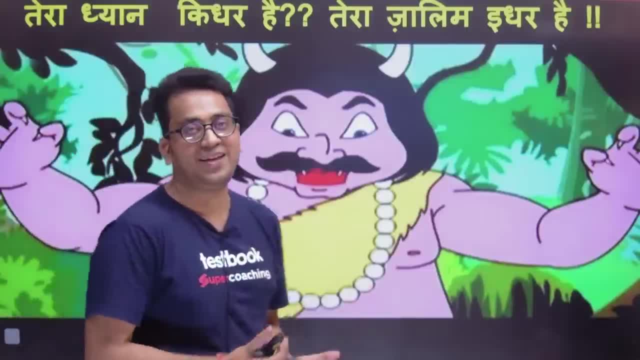 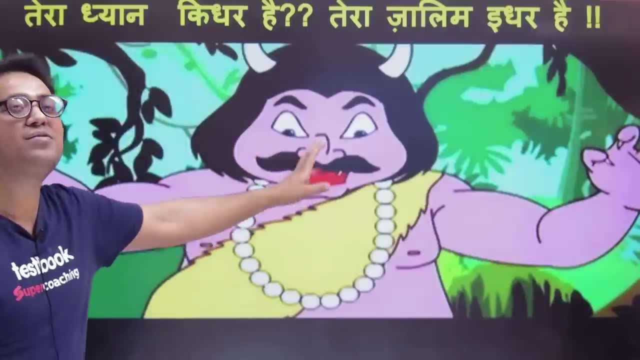 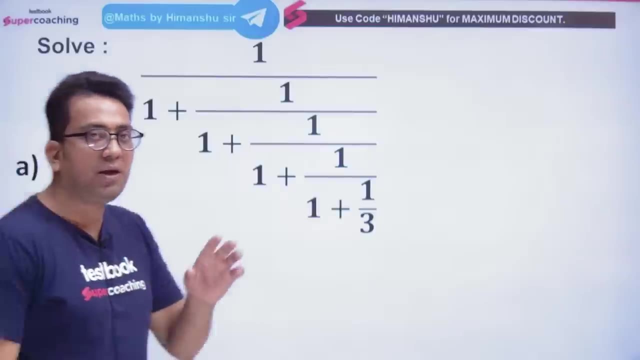 he is saying: where is your attention? your cruel is here. see the questions of the cruel. that simplification, simplification, that question. how does he give come this question: what is it son longra bhin? in fraction bhin, one comes longra bhin. this is the same. 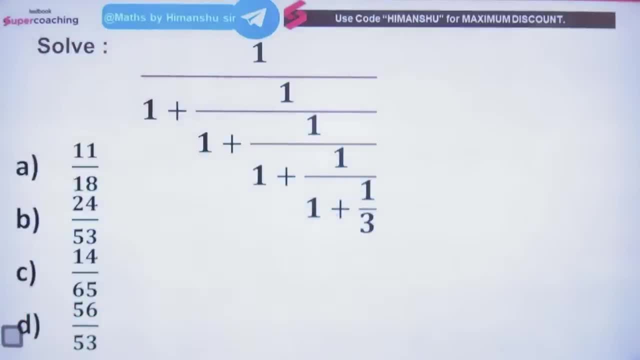 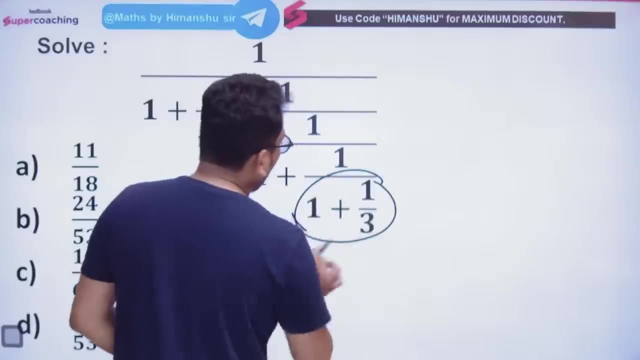 the questions based on this are made in your exam. ok, now see this question. now see this question. if I go to do it in conventional way, then first I will solve this, then whatever will come, I will solve this, then I will keep on increasing this way. I. 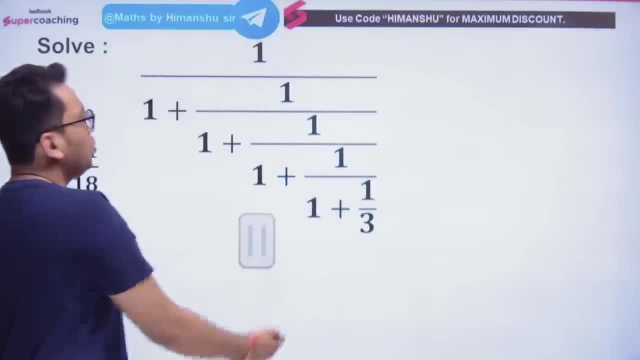 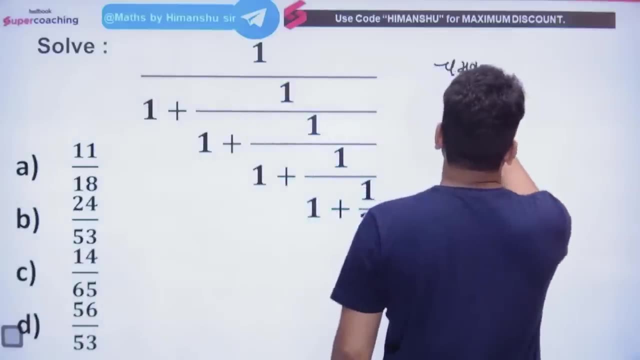 means I will keep on solving it, but if I do this, then it will take a lot of time again. we will shine. we will not solve like this. what will we do? we will shine. we will shine. see the way of shining. what is the way of shining? 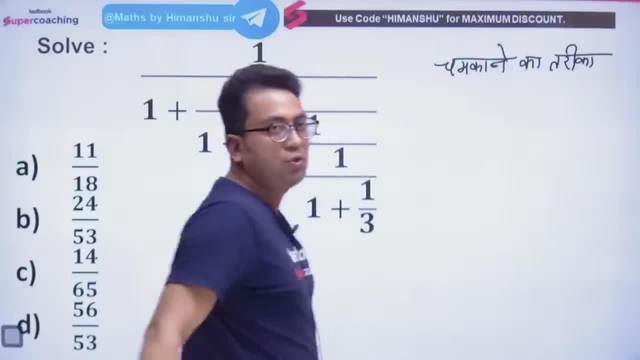 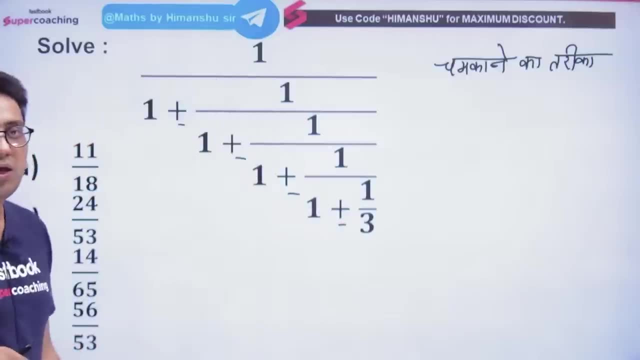 see very carefully what I am going to tell you how you have to shine this question. you just have to see that here, this plus how many times is coming what I said, how many times is coming. plus see how many times is coming this symbol: how many times is coming. 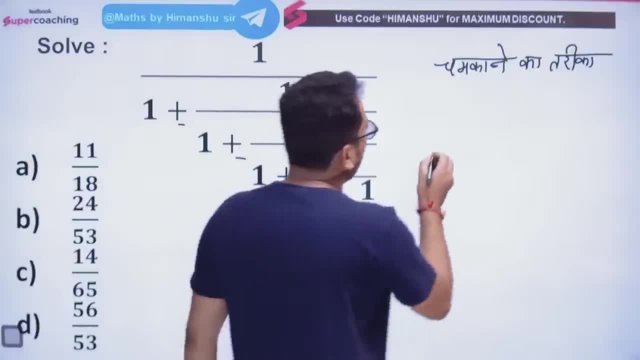 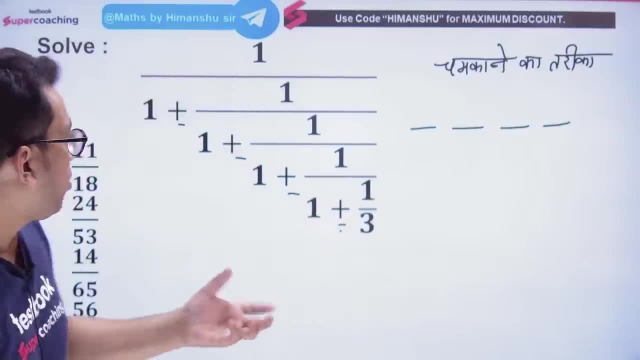 you have seen one, two, three, four, so put four lines. one, two, three, four. you know how to put lines, means you know how to draw lines, everyone knows. so what will you do? one, two, three, four, so put four lines. now understand the thing carefully what you are seeing. 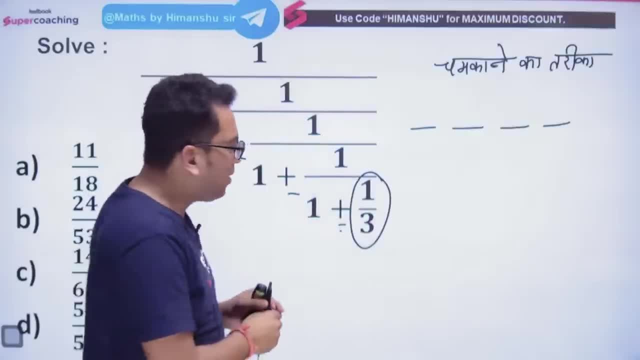 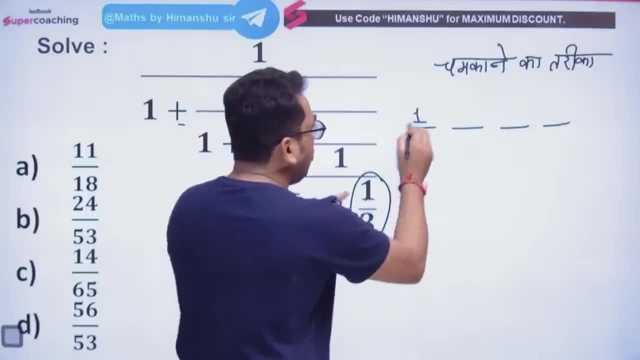 one divided by three. see, in the end you have to pick up from the end, pull the delay leg. see here: one divided by three. so first is one, so write it. one means the one above write it first, the three below write it later. in this way am I understanding the thing. 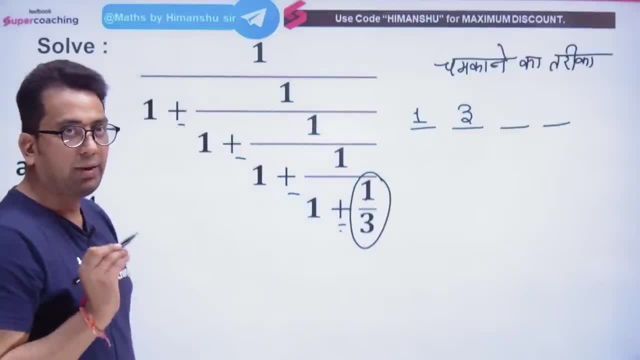 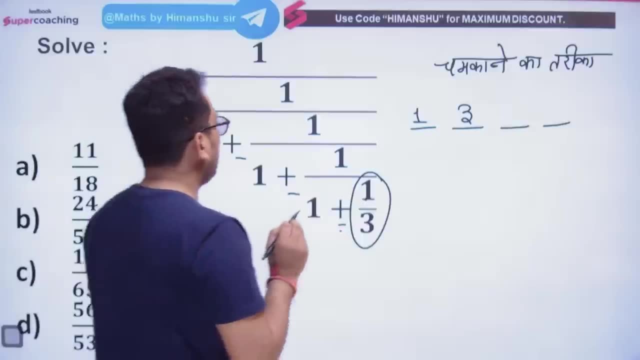 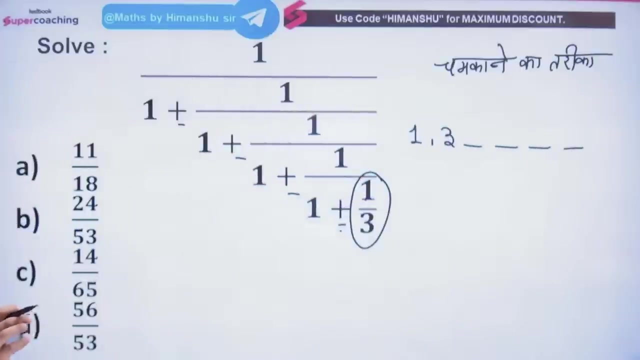 am I understanding the thing? ok, understand carefully. ok, one, three first, then we will put four lines here in this way. ok, because we have to put four lines in this way. ok, because we have to put four lines. ok, ok, because we have to put four lines in this way. 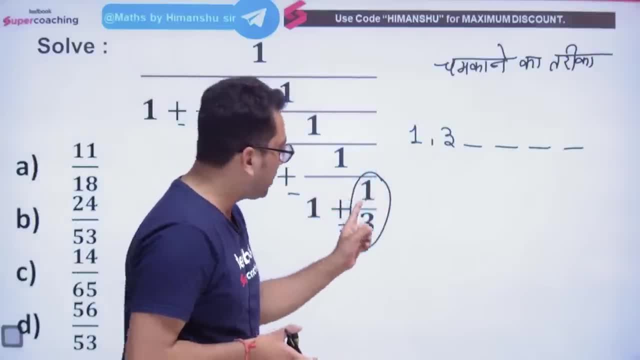 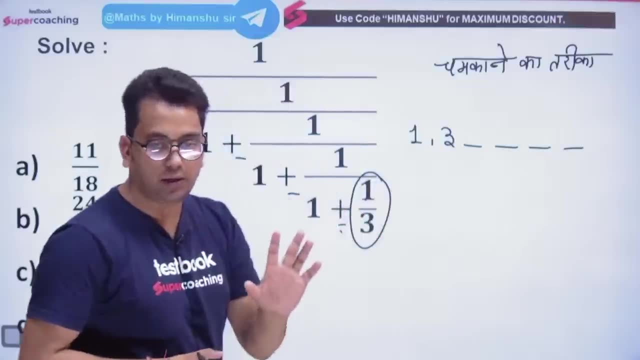 ok, understand carefully this one divided by three. how did you write one divided by three? one above first, wrote it. three below, wrote it later, and four plus signs. you have put four lines in this way. ok, now understand carefully what you have to do. you have to put the one in the back. 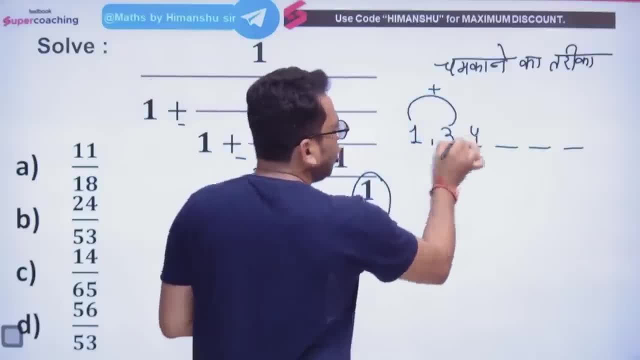 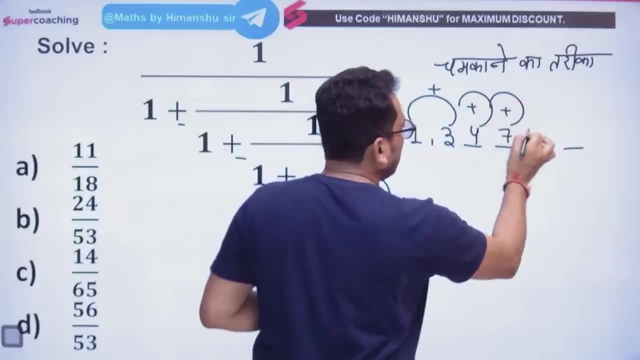 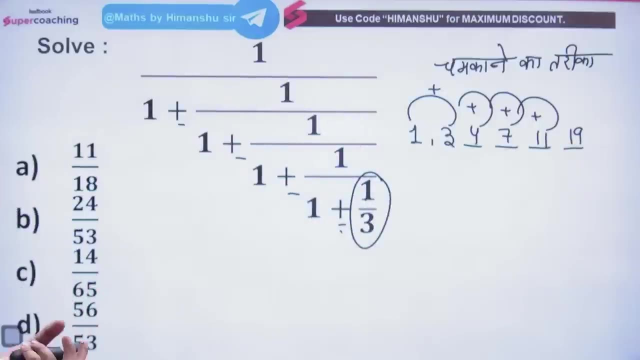 and write it in front of. it means three and one, four. why are you adding, sir? because it is plus, like this: four and three, seven, seven and four, eleven, eleven and seven, nineteen. how many things are you understanding? how many things are you understanding? let me tell you again. 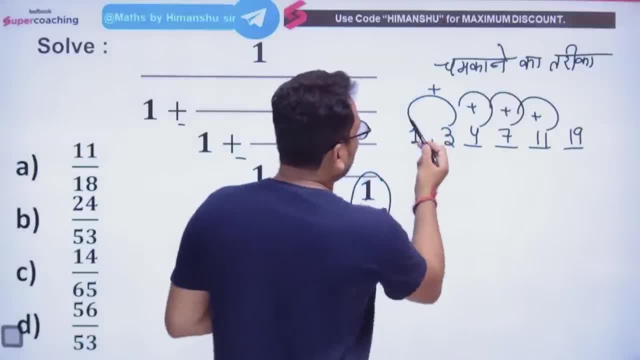 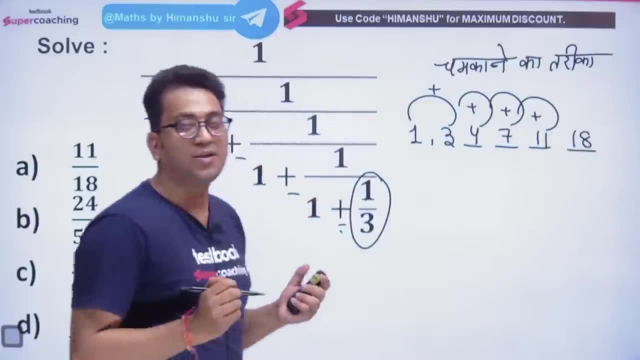 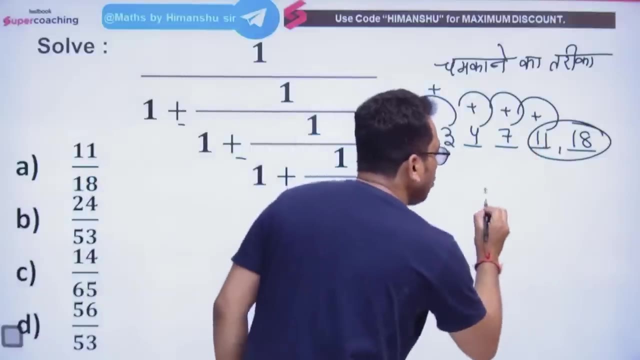 what happened. understand carefully what did you do: one in three, four in four, three in four, seven in seven, eleven, eleven, seven, eighteen, eleven, seven, eighteen. ok, we are doing nineteen, eleven, seven, eighteen. now what we have to do. the last two numbers will be our answer, the one that came first. 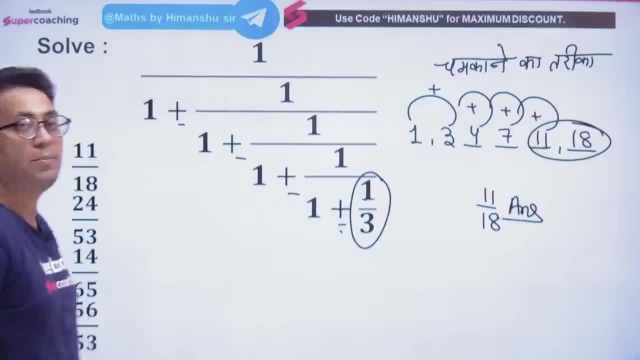 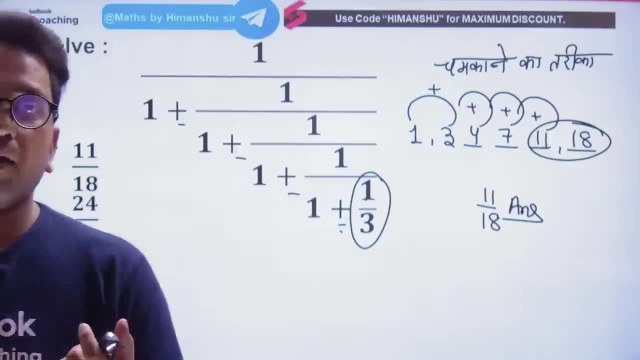 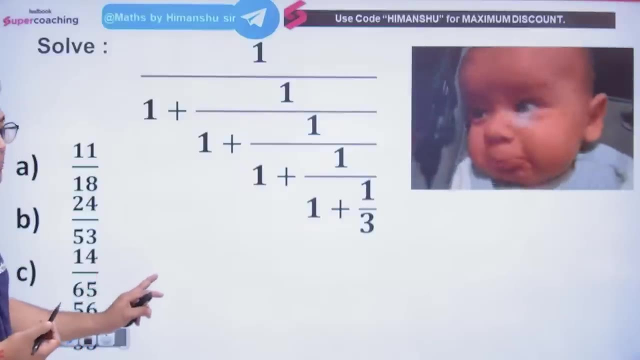 keep it up. the one that came later, keep it down. keep it down, because what we are going to say is that the answer will be not a question. that is our answer. the answer will be not a question but a, not a question but a. we will say: 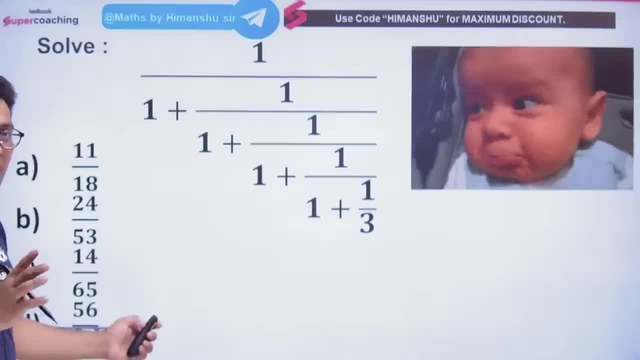 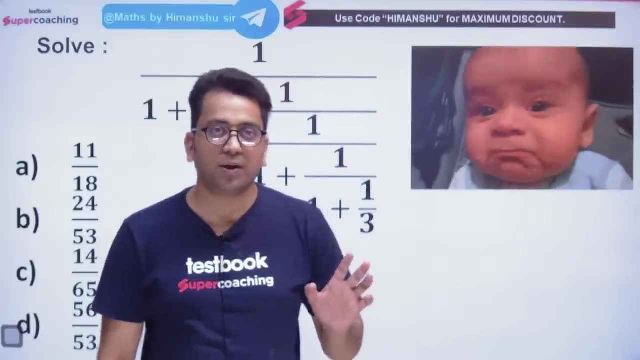 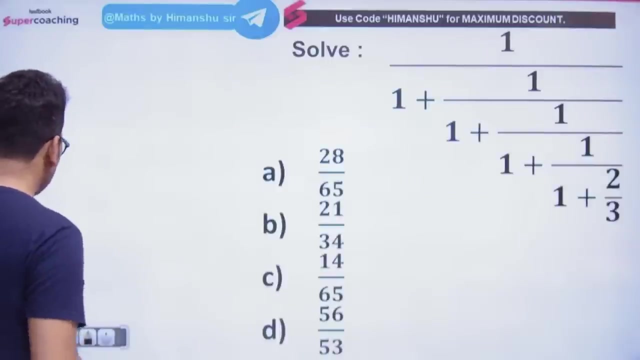 yes, you know, we will say yes, yes, yes, yes, yes, we will say yes, yes, yes, yes, yes. Next question: Tell me quickly what will be the answer. The next question is in front of you. Let's see how many children are able to answer. 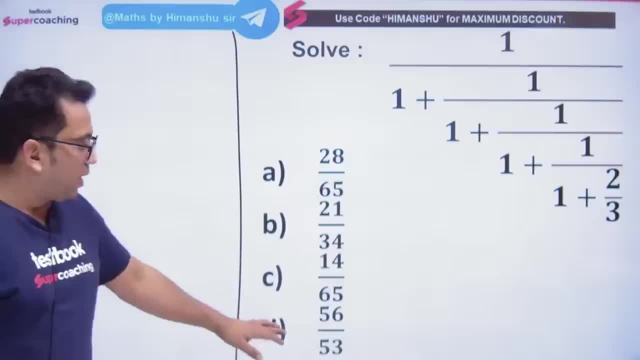 Answer: The question is in front of you, The idea is in front of you. Answer quickly. Let's see how many children are able to answer. Answer: Look, understand carefully. What will you do? Hold the bottom line 2 divided by 3.. 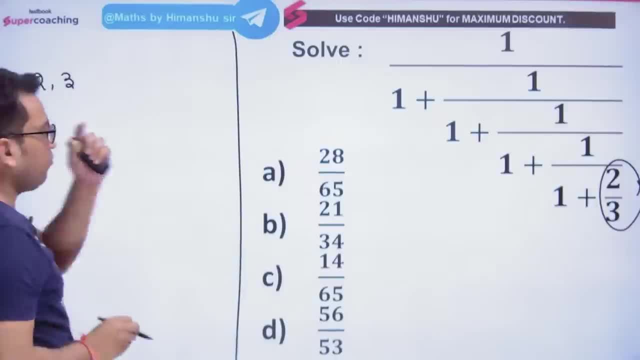 So first write 2. And then write 3. That is the one above is first, The one below is later. Now see how many plus signs are there: 1,, 2,, 3,, 4.. So 4 lines. 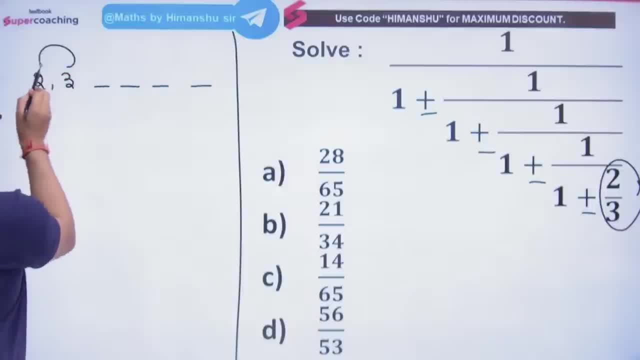 1,, 2,, 3, 4.. Now see, We will add the one in front to the one at the back. 3 and 2, 5.. Write here: 5 and 3, 8. Write here: 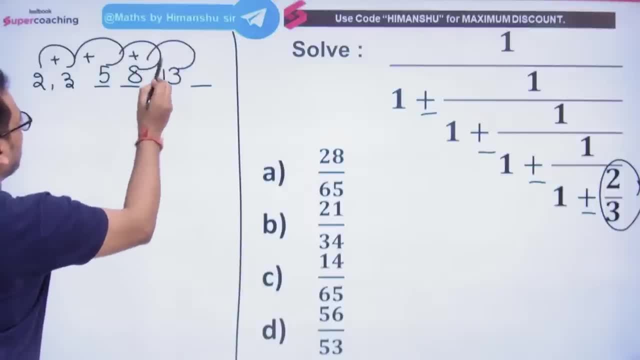 8 and 5, 13.. Write here. 13 and 18, 21.. Write here. So the last two numbers are our answer. 13 is coming first, It will come up. 21 is coming later, It will come down. 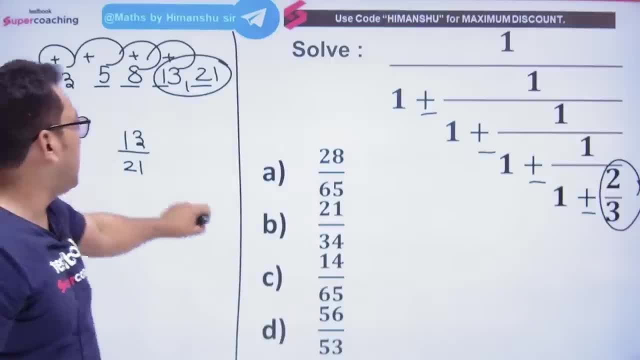 So 13 divided by 21 will get its answer, Which is not given here, Because 1,, 2,, 3,, 4.. Is 13 divided by 21 coming? Yes, So do one option. Do correction here. 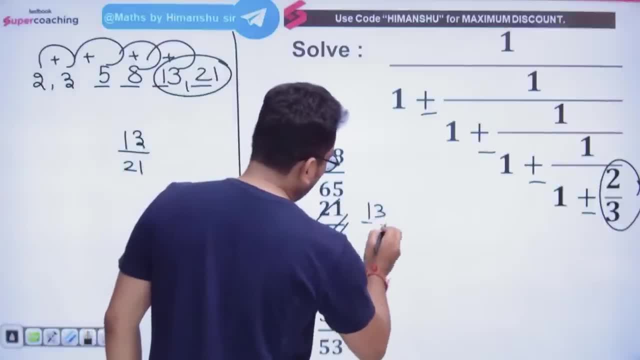 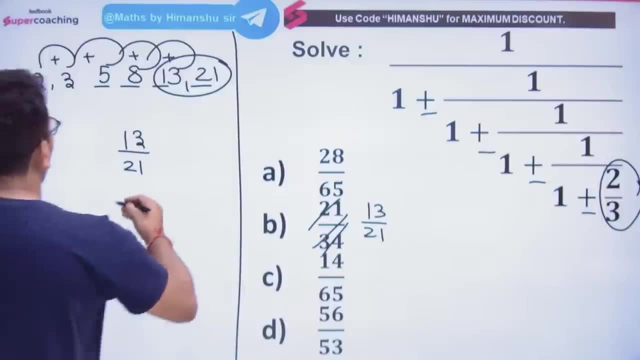 Do 13 divided by 21.. Do 13 divided by 21.. Option is mistake. Do 13 by 21.. Everyone's answer will be 13 by 21.. Is it clear? Yes, Very good. So all the children who gave this answer. 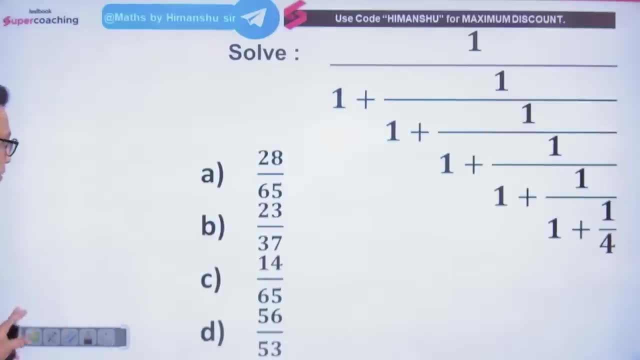 all of them have given the correct answer. Let's move on to the next question. Come on, Answer this question. Tell us what the answer will be. Next question: Give it son, Answer it. All of you, All of you. 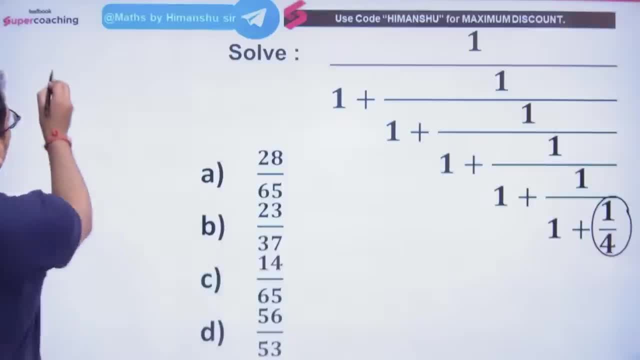 See What do you have? 1 divided by 4. So first 1 is up, So first 1 will come. 1 is below 4. So later it will come 4.. Right, How many letters are there? 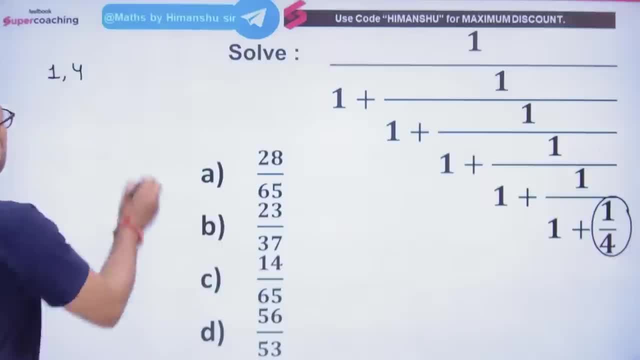 1,, 2,, 3,, 4,, 5.. This time there are 5.. So you have to hit 5 lines, That is, 1,, 2,, 3,, 4, 5.. Right, son. 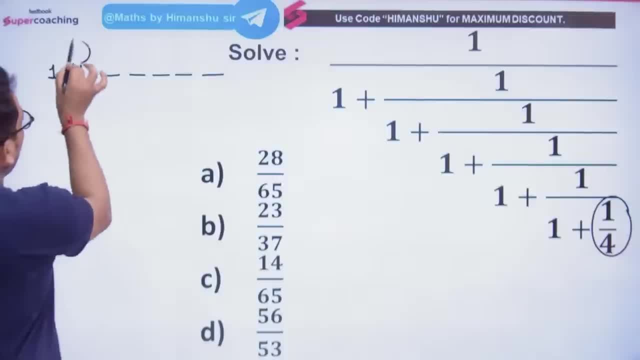 Now, what will you do? You will add 1 in 4.. 5. 5 and 4,, 9. 9 and 5,, 14.. 14 and 9,, 23. 23 and 14.. 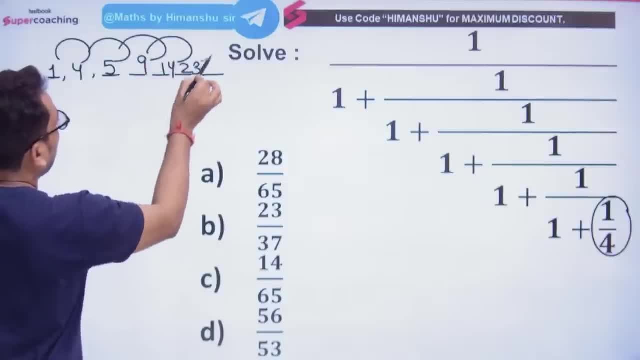 You will get 37. So first it is coming 23.. Later it is coming 37. So what will be the answer? 23 divided by 37. That means our option is also the correct answer. 23 by 37 will be our answer. 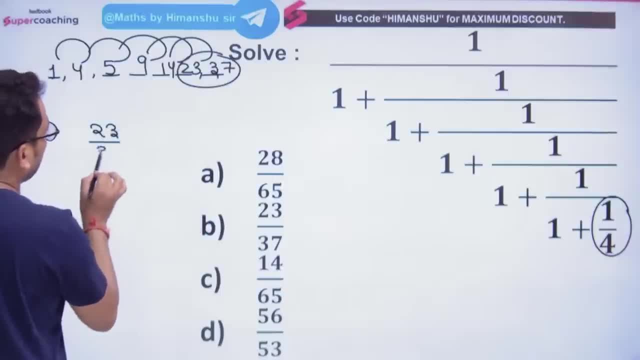 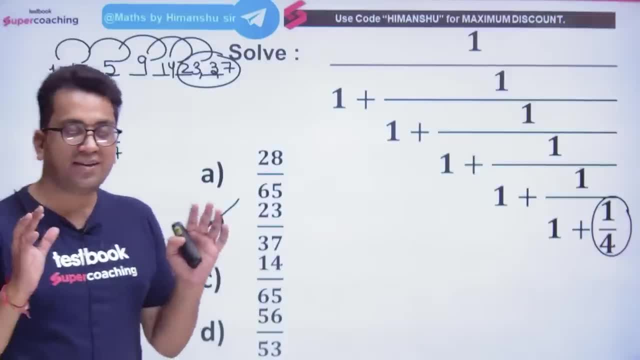 Is it clear, Is it understandable? Is it fun? Press like son All the sessions Once all the children click on the like button once. If you like the session, if you are having fun, then Okay, let's move on to the next question. 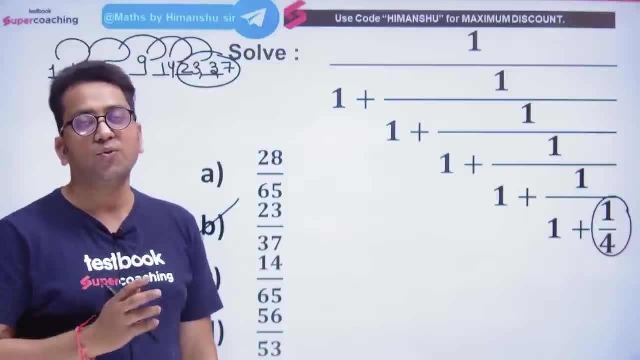 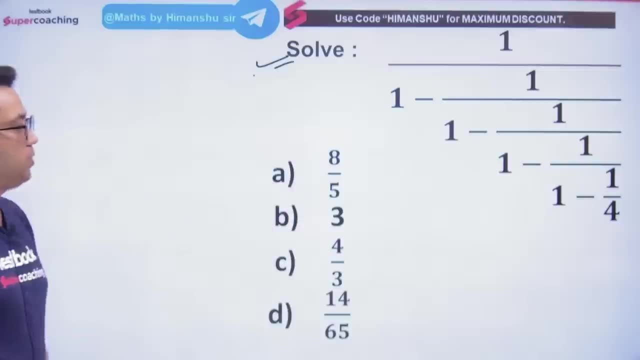 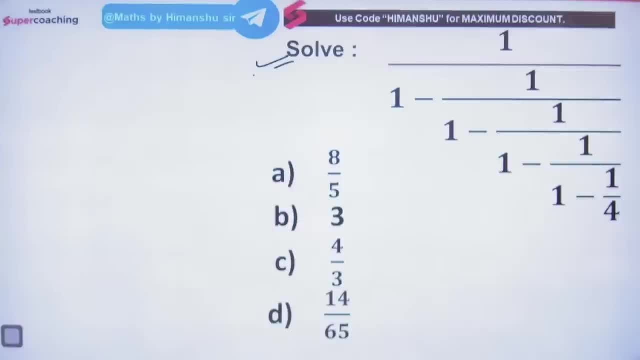 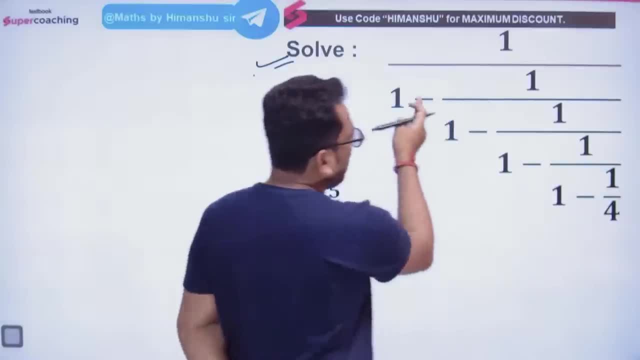 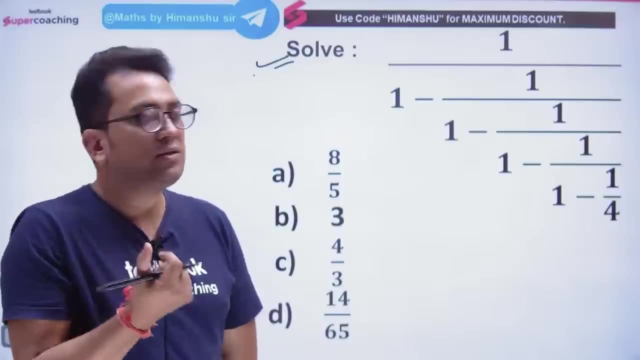 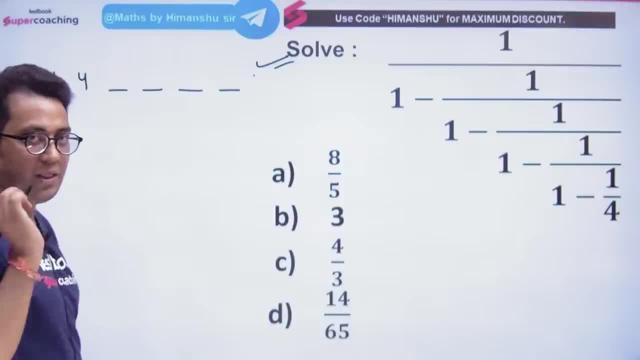 So 1,, 2,, 3,, 4 symbols were there, 4 times minus was there. So we put 4 in this way. Now, what will we do? We will subtract, So understand. Keep in mind the symbol. 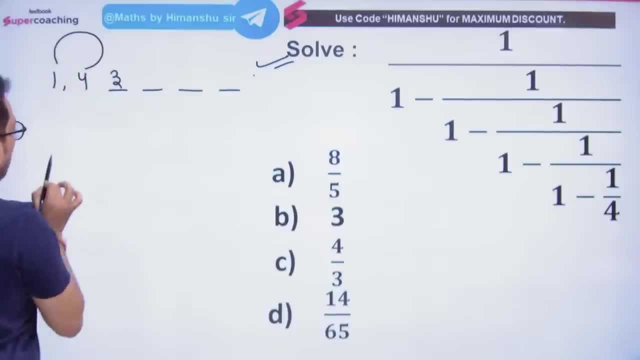 If you subtract 1 from 4, then how much will it be? 3 will be. Are you understanding? If you subtract 1 from 4, then 3 will be. Now, if you subtract 4 from 3, then minus 1 will be. 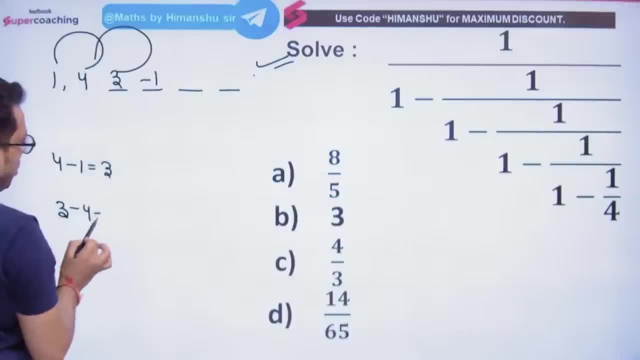 How Look, if I subtract 4 from 3, then minus 1 will be, Because sin is a big number. See now Minus 1.. Minus 1 from minus 3, then minus 4 will be. 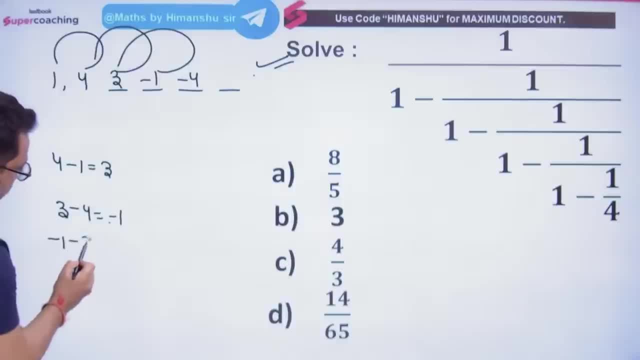 How, sir, Minus 1 from minus 3, then minus minus plus 4 will be, But sin will be minus, then minus 4 will be. How Minus 4 from minus of minus 1, then minus 3 will be. 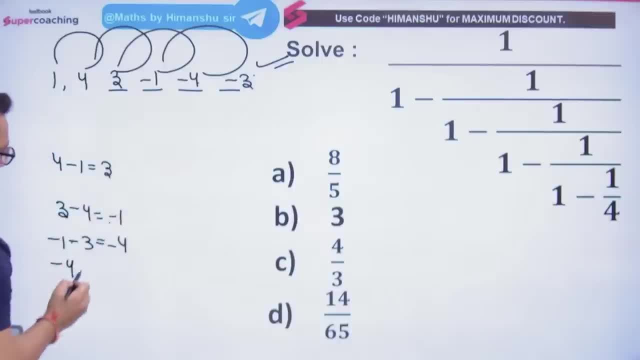 How, sir? Look minus 4 from minus, then minus 1.. So look what will happen. This minus minus will be plus. That means minus 4. plus 1.. Do you understand what I am saying? Now what will happen? It will be minus because minus plus. 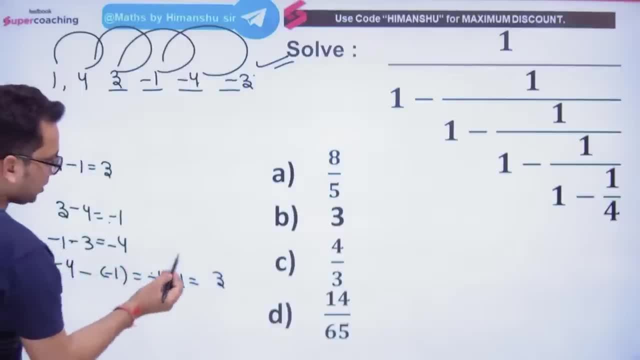 minus is there. So 1 out of 4 is 3.. But the sign will be of a large number, That is, minus 3.. So write minus 3.. I have also written all the things. Now tell me. the last two lines are the same answer, So put the first one. 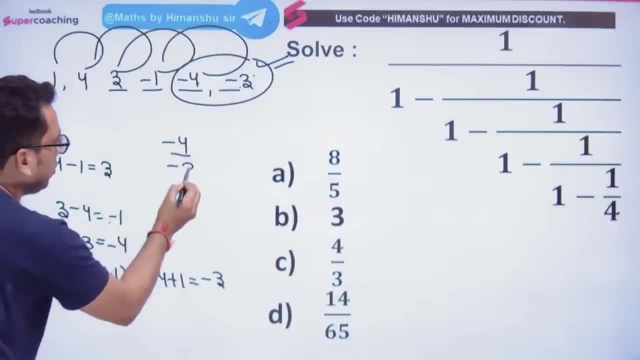 above it and put the one that is coming later below it. That is, minus went from minus 4 divided by 3 is our answer. On the other hand, C will be our correct answer. Do you understand what I am saying? So the answer is: 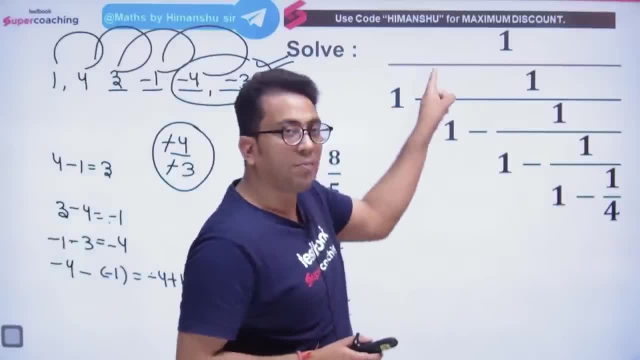 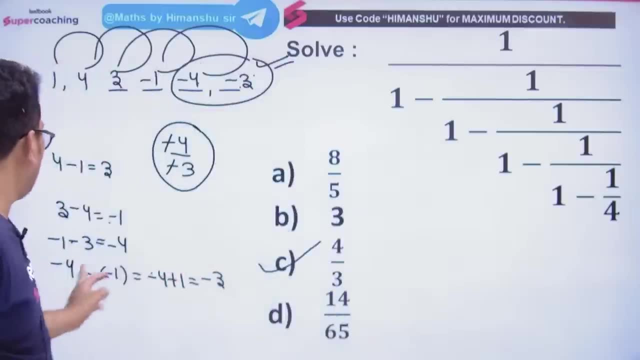 going to be the same. If it is plus, then do plus, If it is minus, then do minus, But you have to be very careful about the sign, ie the symbol. Are you able to understand the matter? Is the matter clear? Let's move ahead, son Next question: Come on, shine quickly and tell me what. 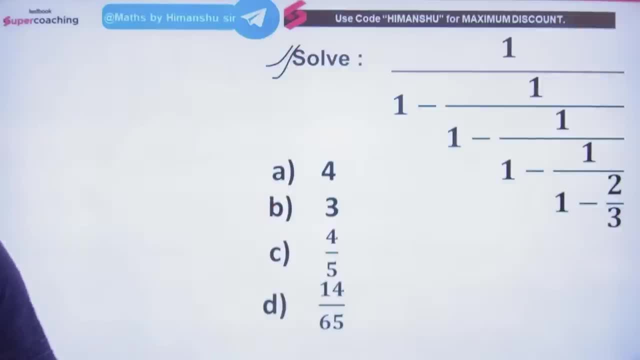 the answer will be: The next question is in front of you. Answer with speed. You have to do minus. Keep in mind the symbol. Keep in mind the sign, Isn't it? Come on, tell me what will be the answer. All of you. 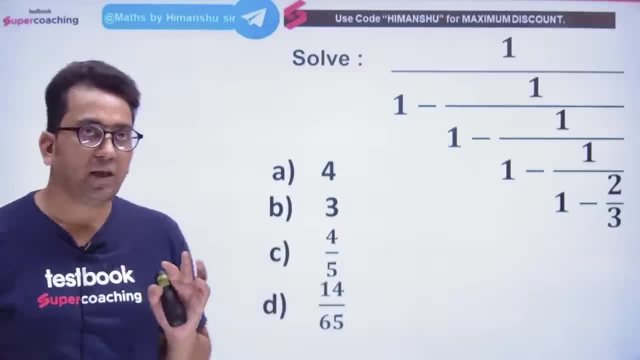 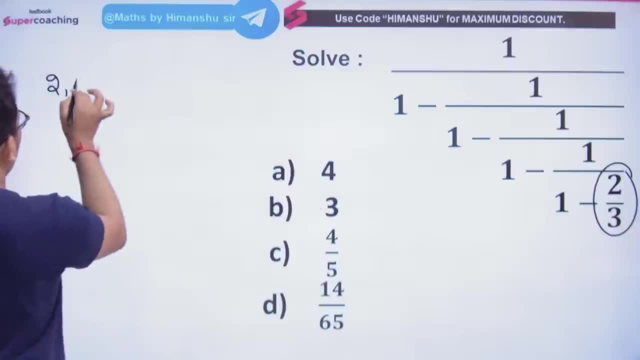 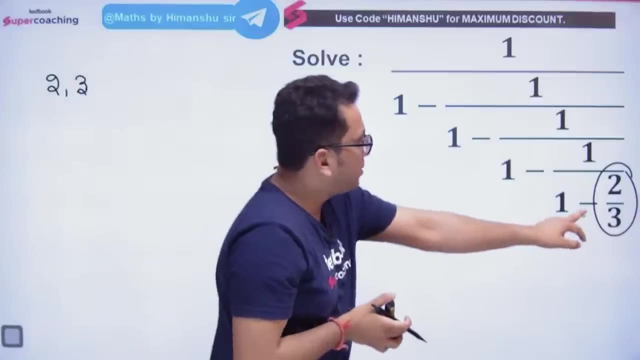 All of you keep answering. You will see two divided by three. What will come first, son? Two will come first. What down? there is three, So three will come later. So two has come, three has come. That is what you are able to understand. two and three came Now. you see how much is minus here. 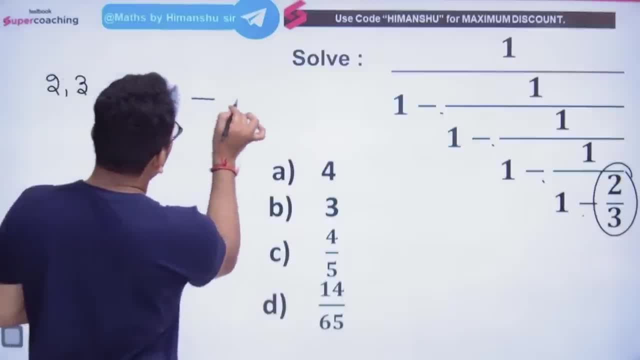 One, two, three, four, Four is here, So there are 4 lines: 1,, 2,, 3,, 4.. Okay, son, Now look, We will do minus. We will subtract 2 from 3.. 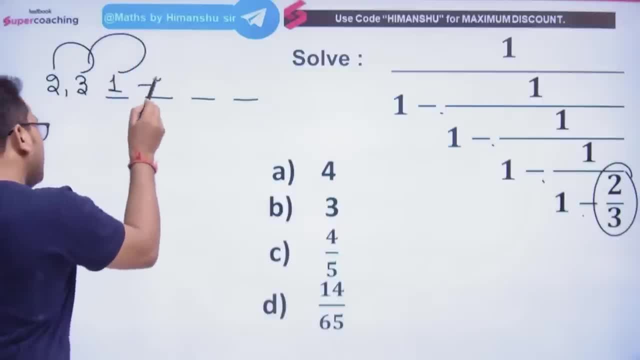 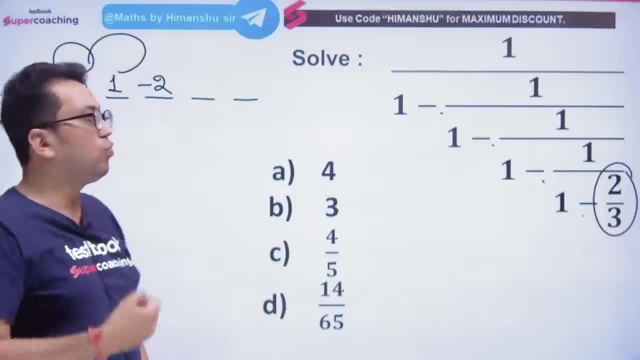 1 came. If we subtract 3 from 1, then minus 2 will come. If we subtract 3 from 1,, 1 minus 3, then sin minus will come and minus will happen Minus 2 of minus 1.. 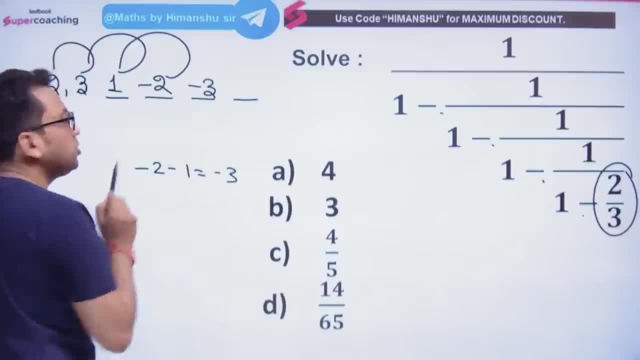 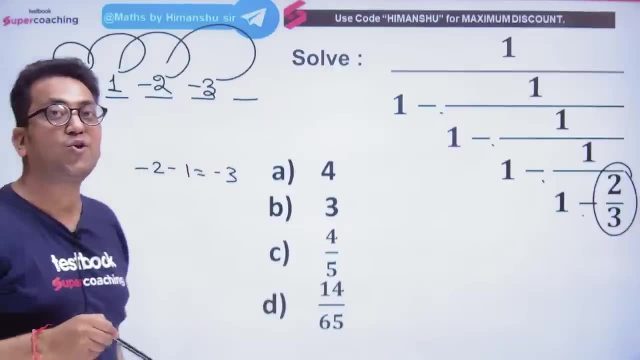 Minus 2 minus 1.. Minus 3 will come. Are you able to understand now? Minus minus plus- Sign of minus will come. Now, if you subtract minus from minus 3, then minus 2 will come and minus 1 will come. 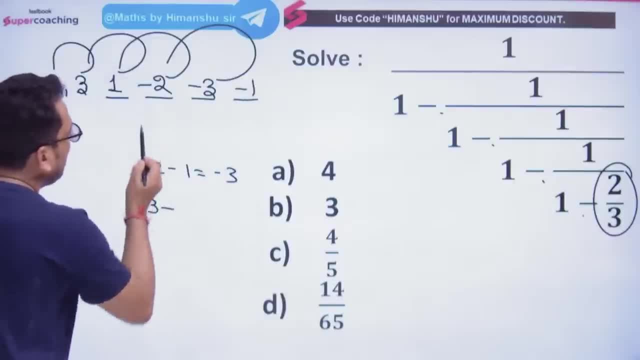 How did the answer come? Look, We will subtract minus 2 from minus 3.. So minus minus is plus. So minus 3 plus 2. So plus minus is minus. That means 2 from 3 will go to 1 and sin minus will come. 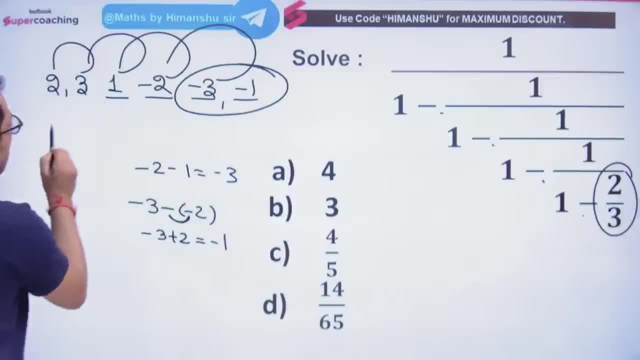 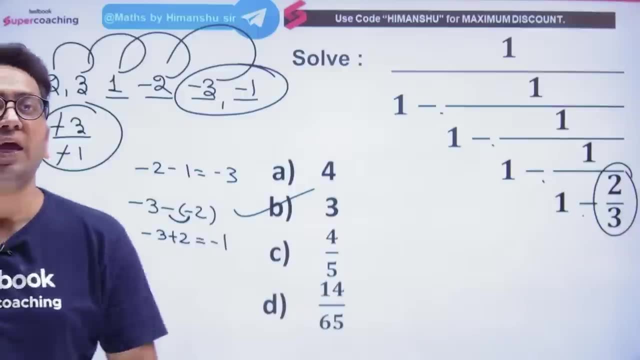 Now the last two numbers are their answer. That means minus 3 up and minus 1 down. Minus 3 minus 1.. That means 3 is our answer. It is absolutely correct. All the children who are doing B answer. their answer is correct. 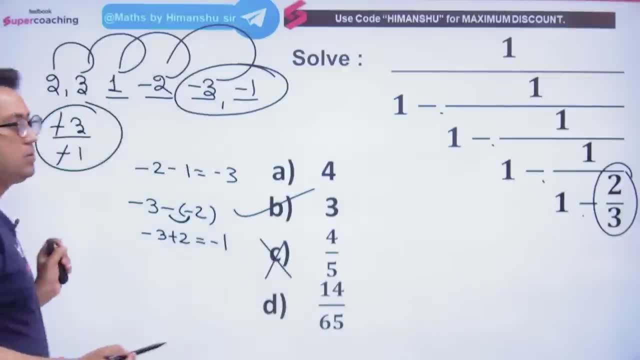 I can see that some of them are going towards C, son. C will not be the answer, B will be the answer, 3 will be our answer. Is it clear? It is fun. Things are coming to understand. Let's move ahead. 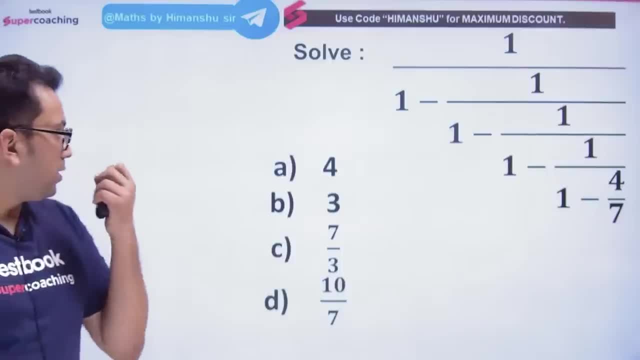 Next question. Here it is in front of you. Tell me what will be the answer. Is it done? Let's check. Yes, it is not done. Come on, tell me quickly what will be the answer. Answer: All of you. 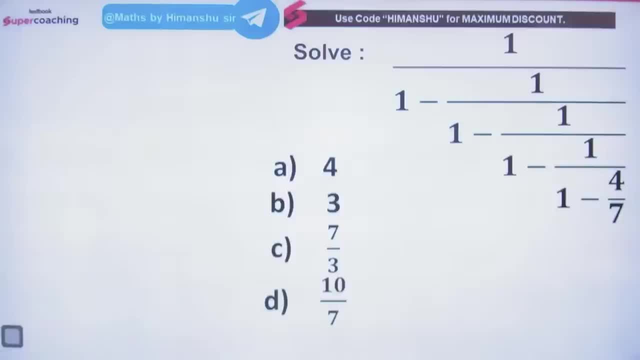 All of you. That's it. Answer: Yes, I fixed this. Yes, I fixed it. You, Guririot…. What will be the answer? Yes, What will be the answer? The last is: you have 4 divided by 7.. 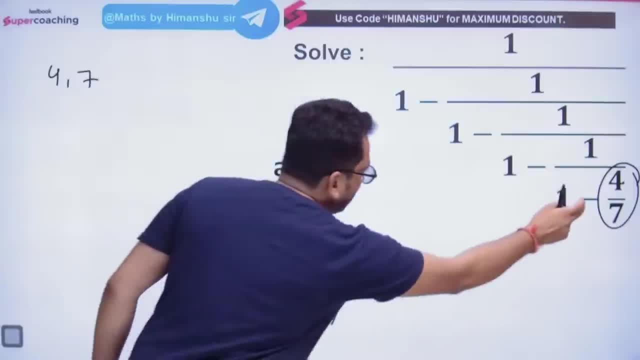 So you have written 4 first and then 7.. How many times is minus 1,2,3,4.. So give four lines: 1,, 2,3,4.. Now we will start reducing it. 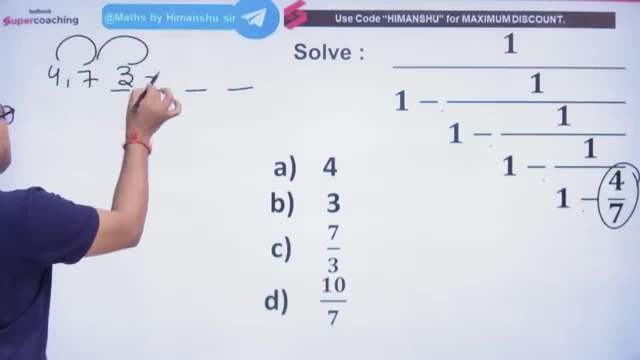 We have reduced 4 from 7 and 3 came. We have reduced 7 from 3 and 4 over minus comes Because it will be of minus Minus 4, minus 3, minus 7 will be there. Minus 7 of minus of minus 4 will be minus 3.. 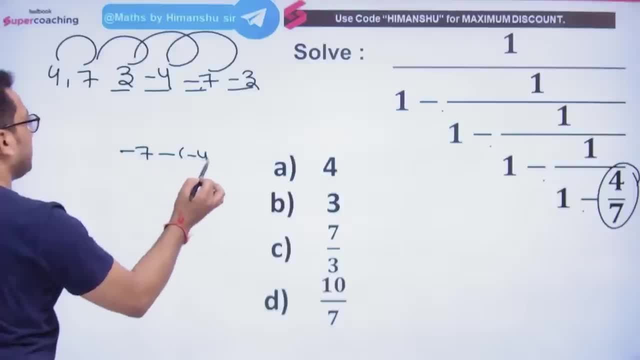 Why See? minus 7 will be reduced from minus of minus 4.. So minus minus is plus. So minus 7 plus 4 will be minus 3.. And the last two numbers are our answer: Minus 7 up, minus 3 down. 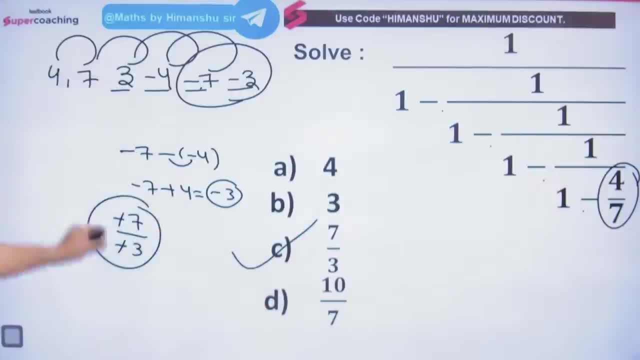 So 7 divided by 3 will be our answer. Tell me how much time is it taking? How much time is it taking to make it shine, Is it or not? Very good, So 7 by 3.. All the children who are answering: their answer is absolutely correct. 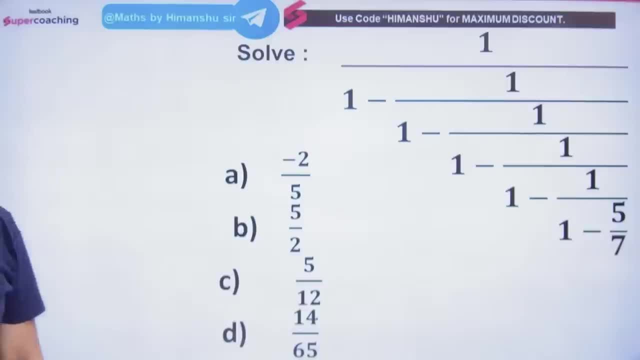 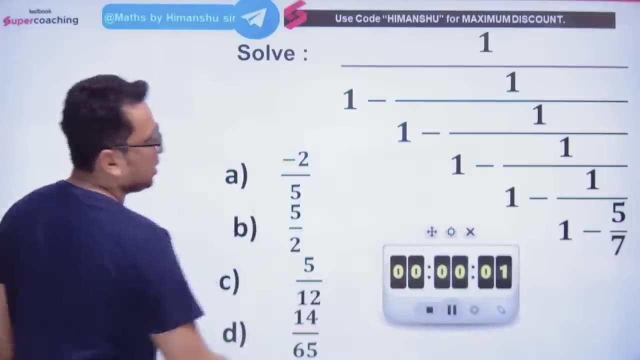 Next question: Come on, shine quickly, Tell me what will be the answer. I want all of you. I am setting you a timer of 20 seconds. In this 20 seconds, every child has to answer. Okay, Come on, fly, son. 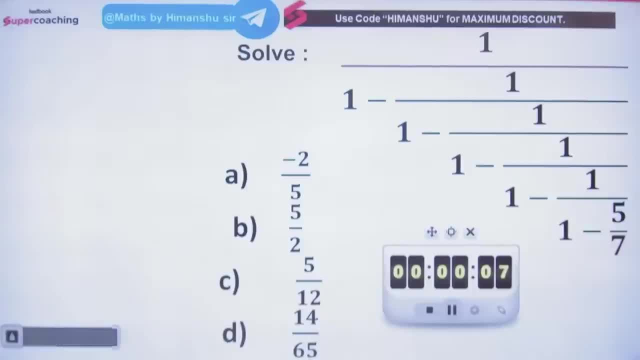 Tell me what will be the answer. I want all of you. I am setting you a timer of 20 seconds. In this 20 seconds, every child has to answer. Okay, very good, Here the children are answering. Come on, son. 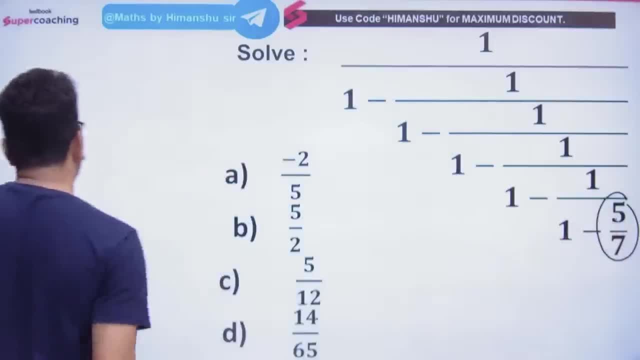 What you have to do is: 5 by 7 is visible. So first write 5 as 5.. Later write 7 as 7.. How many lines are there? 1,, 2,, 3,, 4,, 5.. 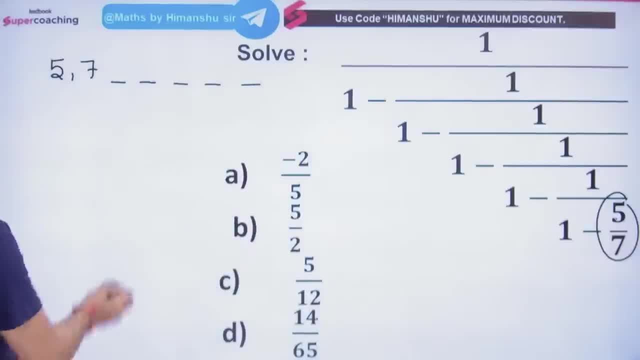 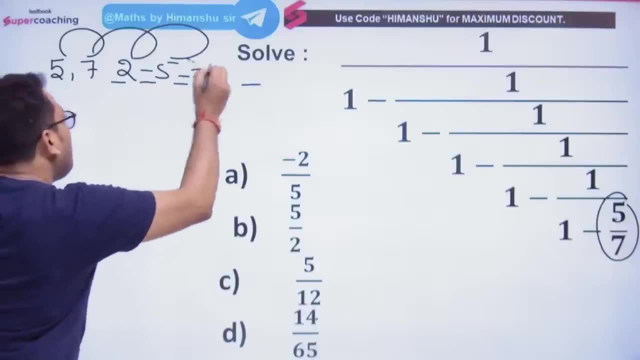 So 1,, 2,, 3, 4, 5.. 5 lines are there. Now what is next? We will start subtracting. 7 out of 5 is 2,. 2 out of 7 is minus 5, minus 5 out of minus 2 is minus 7, minus 7 out of minus of minus 5 will be minus 2, are you able to understand what I am saying? 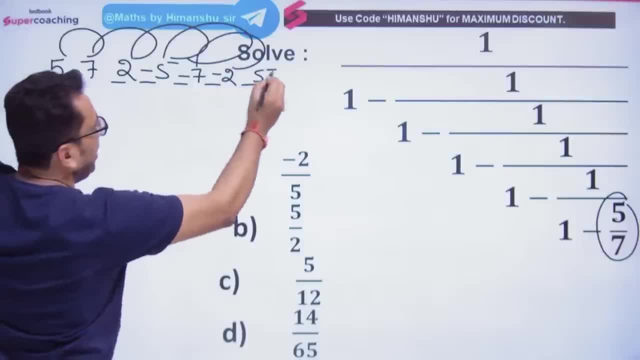 And then minus 2. out of minus of minus 7 will be plus 5,. now, sir, first is minus 2, last is 5, so minus 2 divided by 5 will come. tell me, is the answer coming? 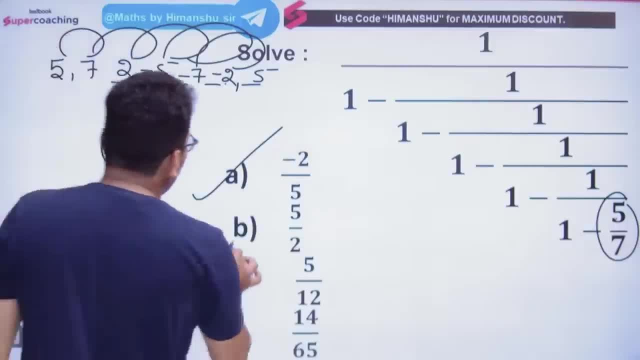 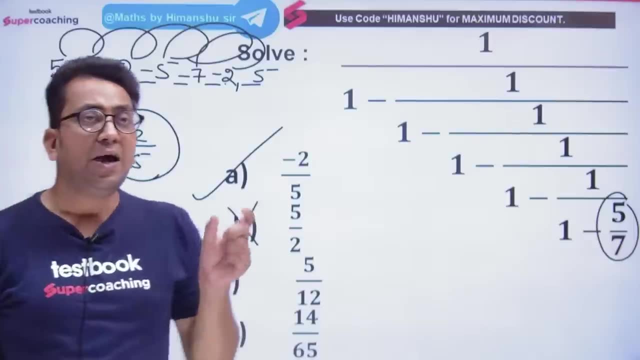 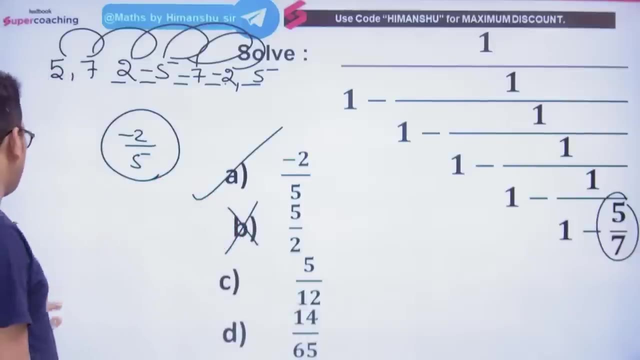 Yes, A answer will come. son, B will not come. you are doing wrong. you are doing wrong. see, somewhere you will get stuck. do it carefully, do it easily. you will get minus 2 divided by 5. answer: it is a plus minus game, son. it is just a plus minus game, simple. plus minus should come, everyone's answer will come right. A is our answer now. the child will think: sir, you are doing plus minus. if both come, then what will we do? 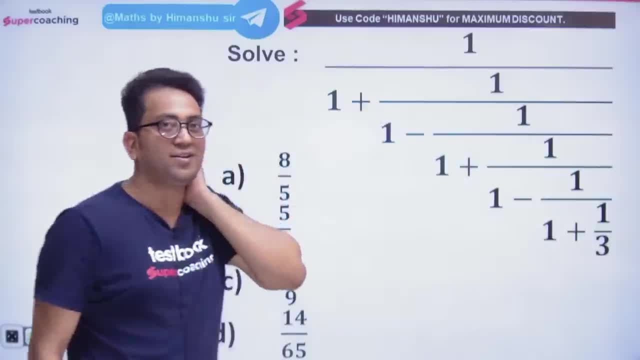 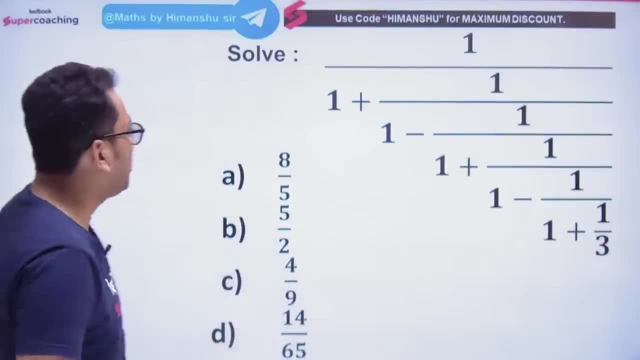 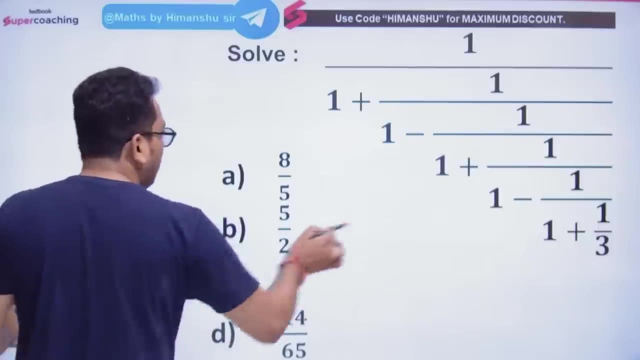 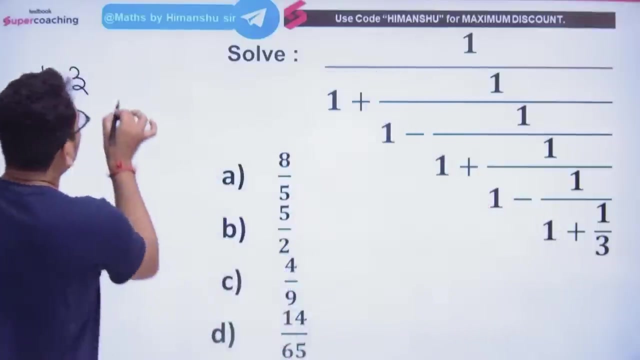 Brother, look in this question, plus also came, minus also came. it was amazing. plus also came, minus also came. now what to do? Hey, whatever he says, he will do. look 1 divided by 3, what is 1 divided by 3, look carefully here: what is 1 divided by 3, then what will our child do? 1 divided by 3 will write 1 first, 3 later. see how many numbers: 1,, 2,, 3,, 4, 5, put 5 numbers 1,, 2,, 3,, 4,, 5, now understand my thing very carefully. 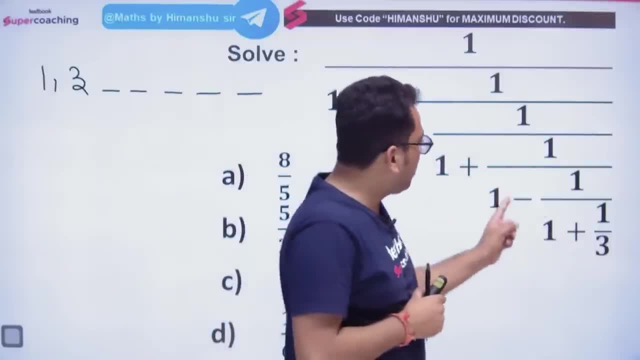 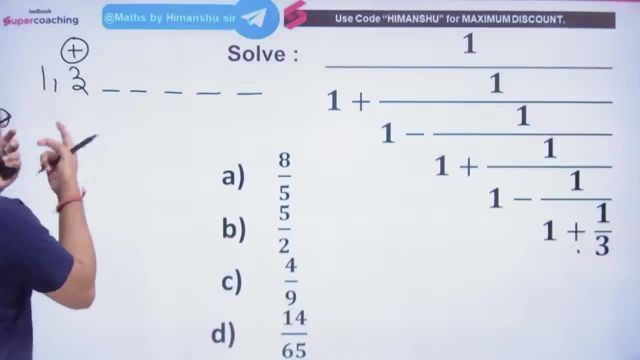 before, plus, plus used to happen or minus, minus used to happen. now, plus, minus, plus minus is going like this. so first see what is first. If the first is plus, then put plus on it. It will tell me whether I have to do the next plus or minus in it. 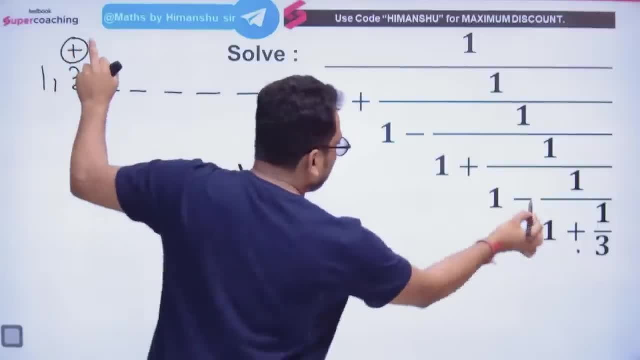 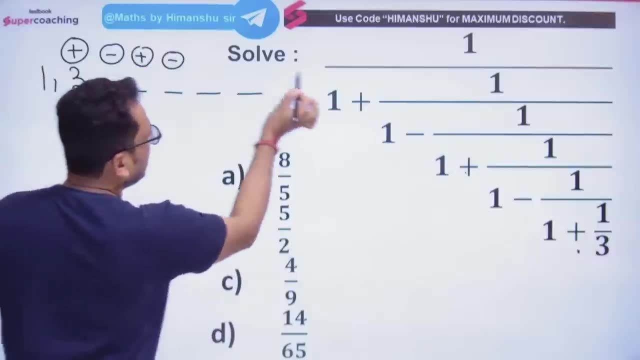 Do you understand? So you put plus After plus what is minus, So here is minus. Then what is plus, So here is plus. Then what is minus, So here is minus, Then what is plus, So here is plus. 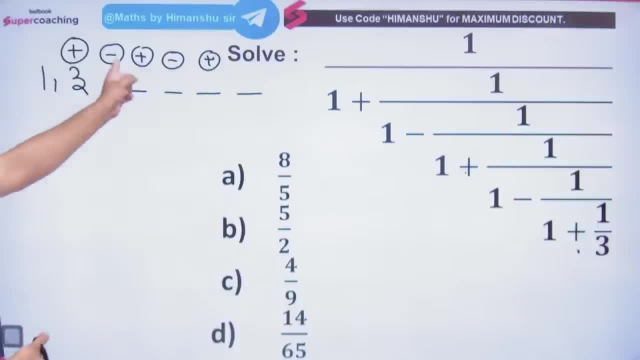 After saying it I am able to understand. So plus minus, plus, minus plus. Now see how it will work. I have to add the next one in 3.. So 3 and 1 is 4.. I have to subtract 3 from 4.. 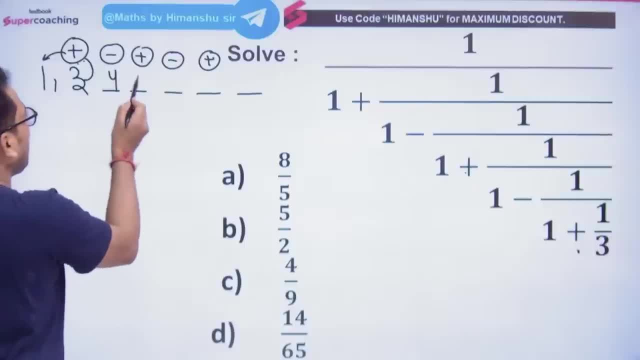 This minus will tell that I have to subtract, So we will subtract 1 from 4.. Plus will tell that we have to add, So we will add 4 to 1, 5. Minus will tell that we have to subtract. 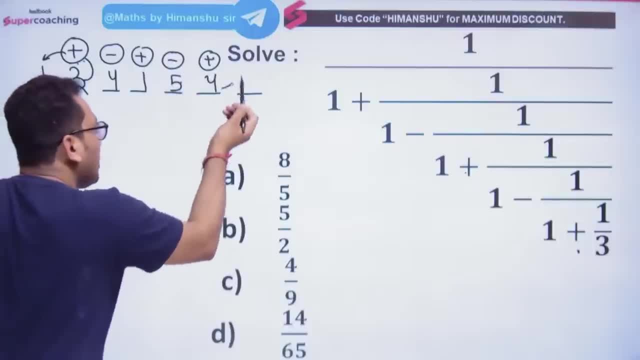 We will subtract 1 from 5, 4.. Plus will tell that we have to add. We will add 5 to 4, 9.. So, brother, the last two words that we get, that is our answer, That is, 4 will come up and 9 will come down. 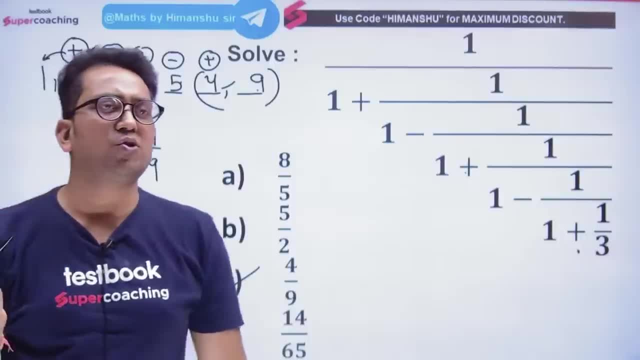 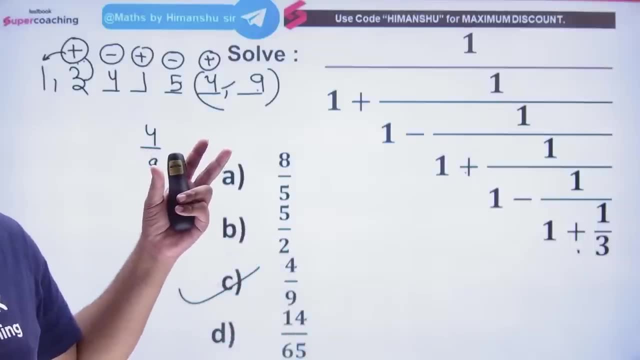 See how easy it is. You will enjoy solving the question. Tell me who is such a child? Who is such a child? I am not enjoying this question. Okay, Sir, you don't take regular classes. Okay, I don't take regular classes. 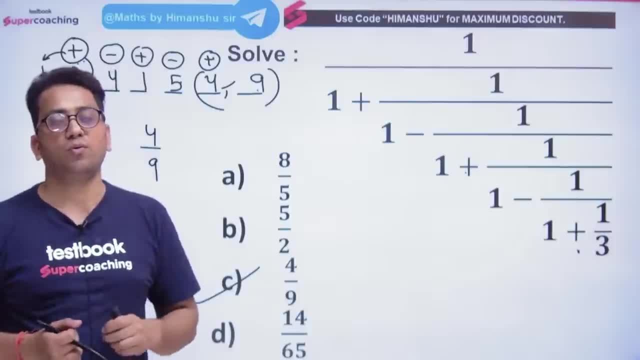 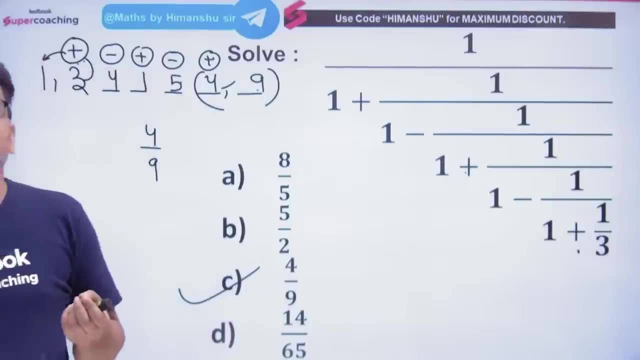 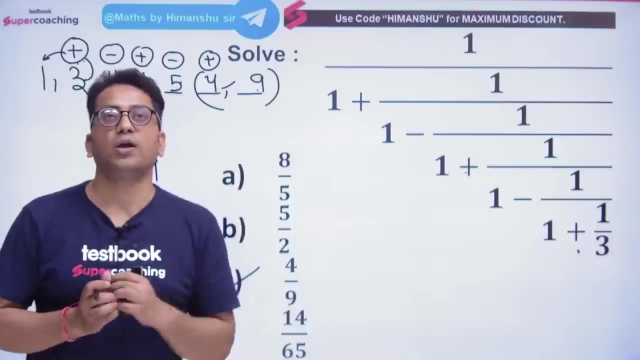 You don't take regular classes, I take regular classes. I take regular classes Only this Sunday. your class was not possible. That is only because I was conducting the interview of KVS TGT, PGT, whose cut-off was cleared. 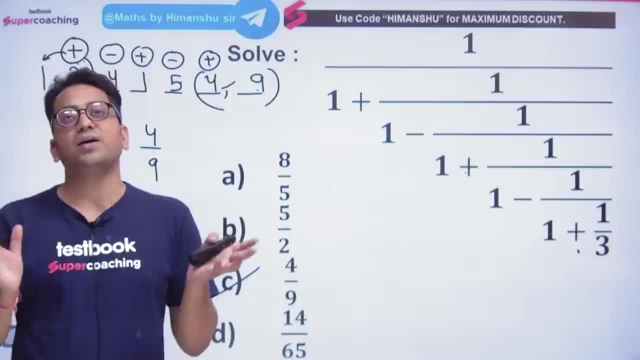 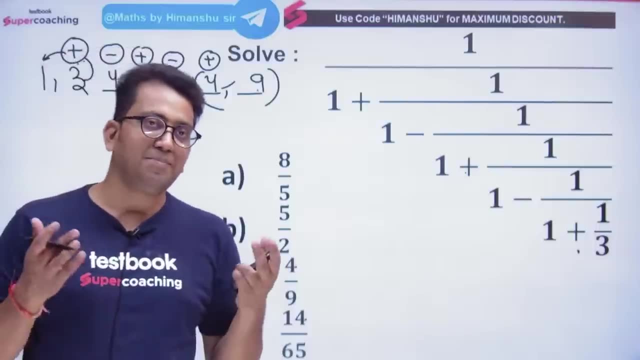 Otherwise, I take classes on Sundays too. I take daily classes. Only on Saturday my class is not possible Because your mock test is at 12 o'clock. So if you take the class, come and join at 12 o'clock. 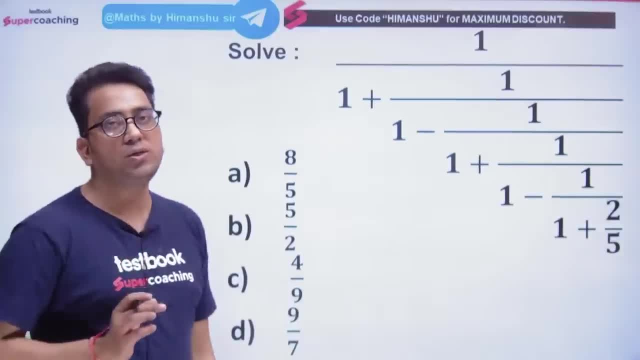 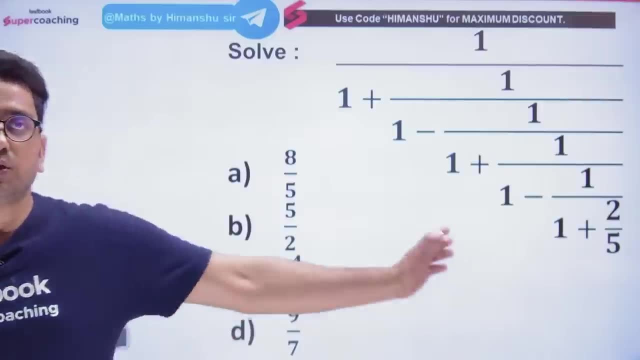 Okay, And today my class will also be at 2.25 o'clock on this channel. At 2 o'clock and 15 minutes Right, children have to come and join. Shine this question. If you understand the thing, then shine this question. 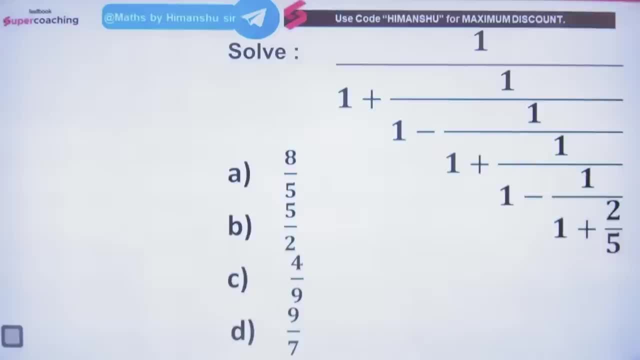 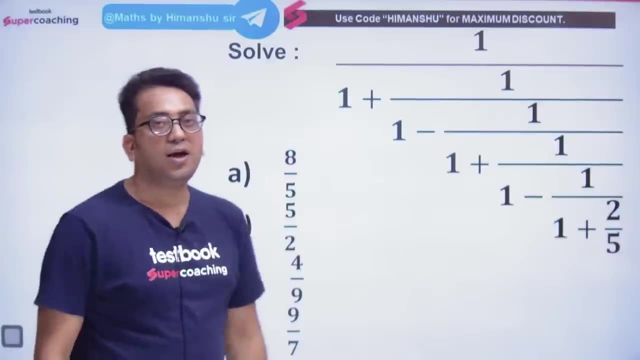 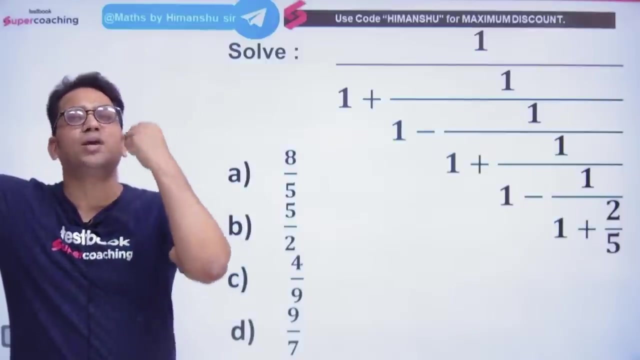 Tell me what will be the answer. Come on, Okay. So the same thing happened. We did not wake up. So we are saying that it did not happen in the morning. Huh, We did not wake up So we thought that the night is happening. 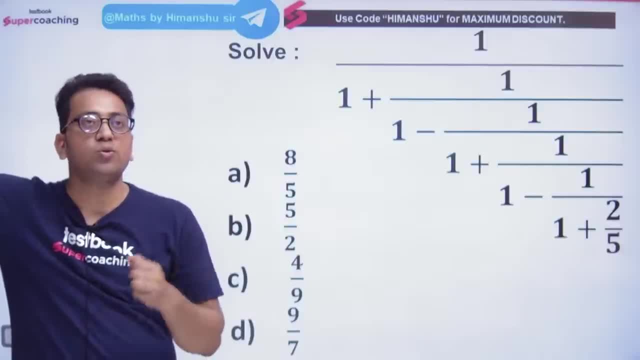 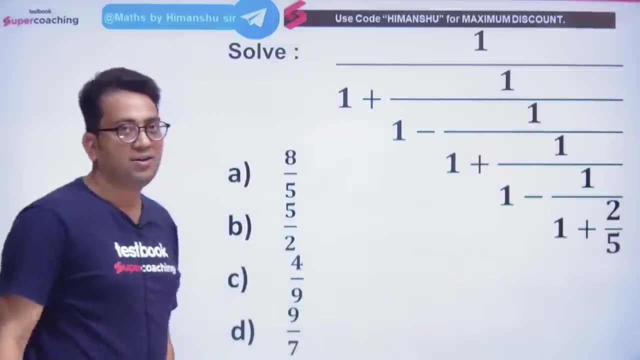 It did not happen in the morning. That is why we did not wake up. Son, come and join, Understand it. Come and join at 12 o'clock You will find the way of shining the questions here. Okay, You will find the way of shining the questions. 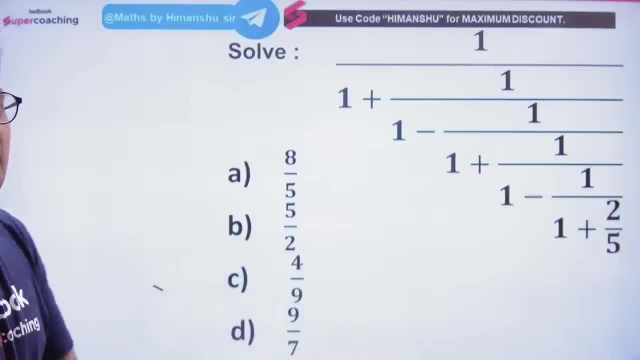 Right at 12 o'clock. Okay, Come and join. The result of KVSPLT did not come, Son. I am not talking about PLT, I am talking about TGT, PGT. Okay, TGT PGT, which is of KVSPLT. 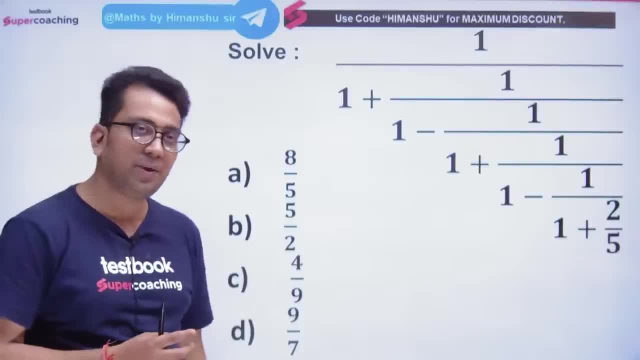 the interview content. Yes, PLT did not come either, Son. let's talk about this question. Understand it carefully Here: 2 divided by 5 is there. So what is 2 first, What is 5 later? 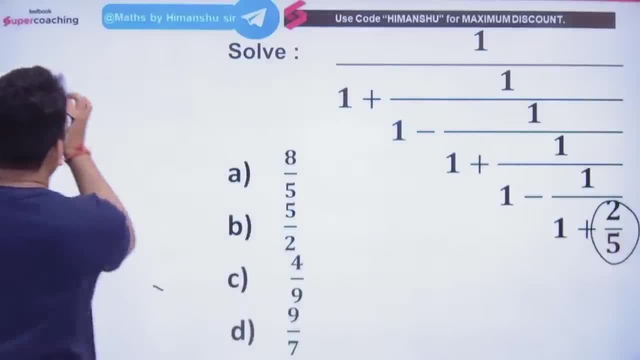 Okay, After that you saw how many symbols are there, Son. so 1,, 2,, 3,, 4, 5.. So 1,, 2,, 3,, 4,, 5 are there. 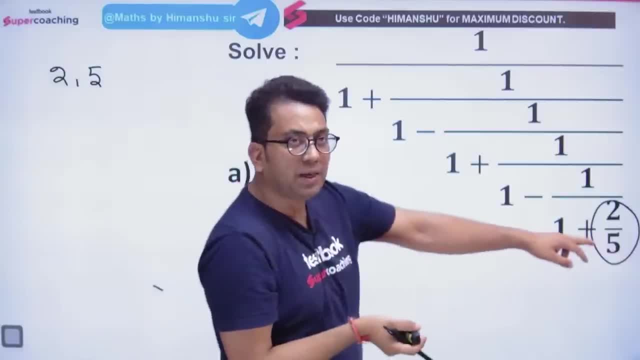 Clear Now: see Plus, minus, plus, minus, plus is there, So see a little Plus, minus, plus, minus, plus. Put it like this Now: see Plus, minus, plus, minus plus. 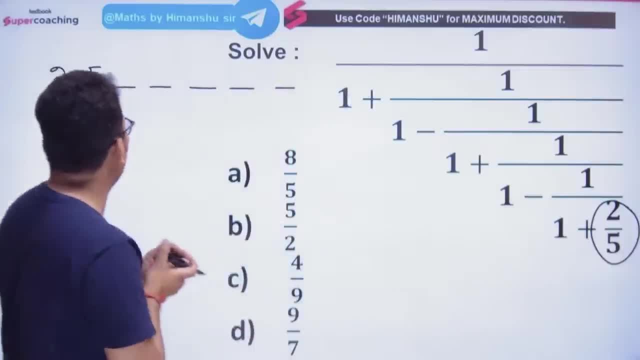 Put it like this: Now see Plus, minus, plus, minus, plus is there. So see a little Plus, minus, plus, minus, plus. Put it like this: Now: this will tell me: plus, join right. 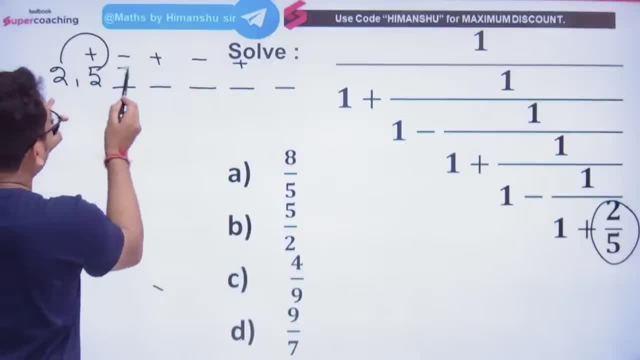 That is, 2 out of 5 will join 7.. 2 out of 5 will subtract 2.. 7 out of 2 will join 9.. 7 out of 9 will subtract 7.. 9 out of 7 will join 16.. 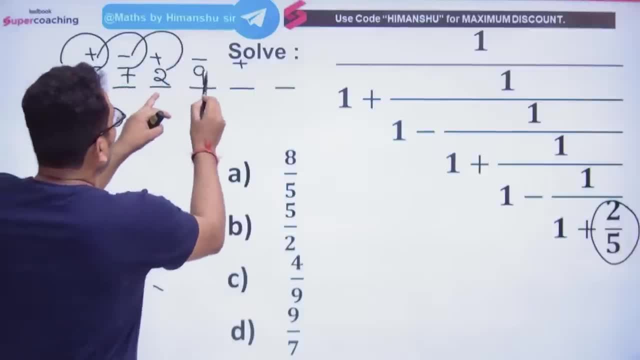 So, brother, the last two words are our answer, That is, 7 divided by 16.. Our answer had to be 7 divided by 16.. Which is not here, Is 7 by 16 coming. Everyone's 7 by 16 answer will come. 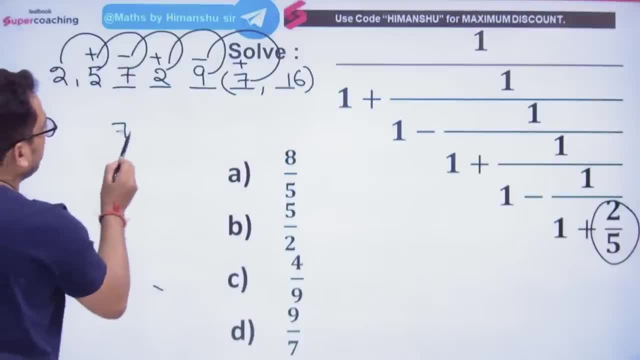 7 divided by 16. answer will come. Now see: Now see: 7 divided by 16.. Now see, Now see: We have taken 7 by 16 from here, So 7 divided by 16 mark. 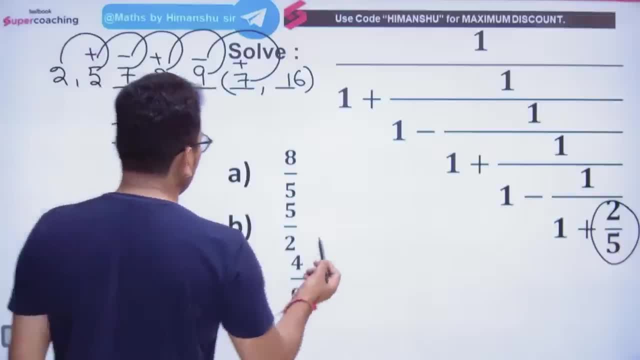 This is a mistake somewhere. This is a mistake somewhere in the options. So 7 by 16, do it. D will not happen. Some children are answering d. The answer will be son 7 divided by 16.. D from where it came. 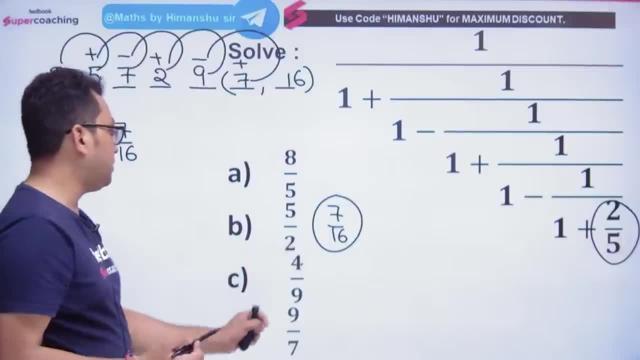 Oh brother, See, It is to be added or subtracted. It is to be added or subtracted. It is to be added or subtracted, So add or subtract. Add or subtract. There was 2 divided by 5.. 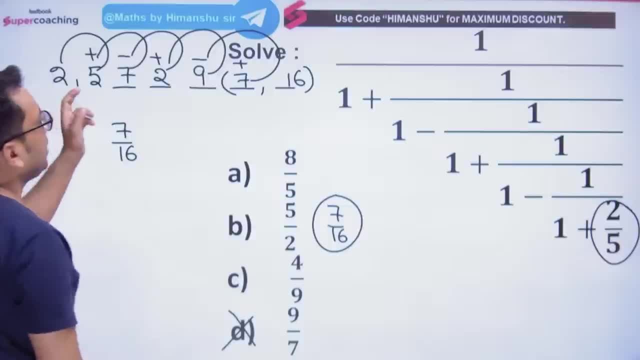 2 divided by 5 was 7.. 5 divided by 7 was 7.. Or 2 divided by 7 was 7.. If 7 divided by 7 is 6.. I said, 7 divided by 6 is 16.. 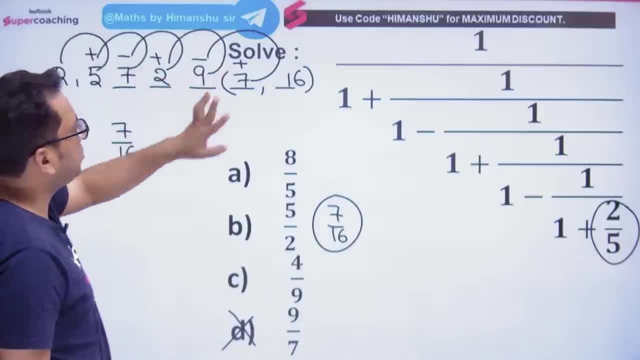 So here we have 11,. 11 is 16.. 2 divided by 5 is 7,. 7 divided by 5 is 7,. 2 divided by 2 is 7,. 9 divided by 9 is 7,. 7 divided by 9 is 16, the answer is 7 divided by 16, you don't have to think about it. 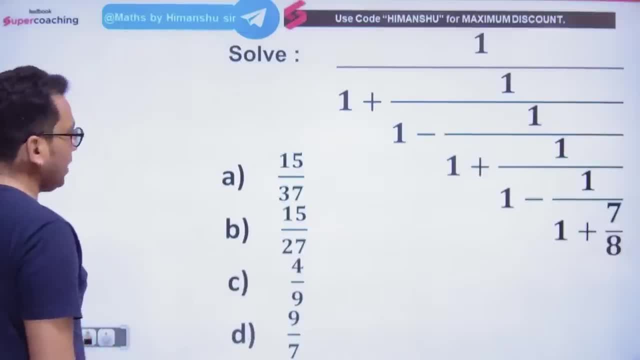 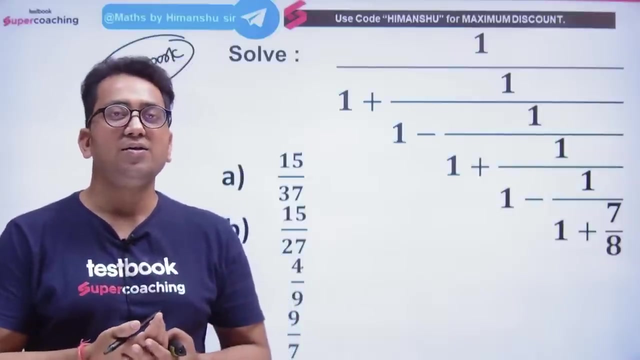 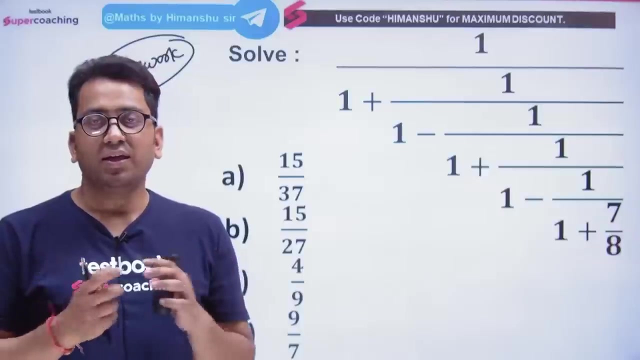 Now, one of today's session will be your homework question. Okay, now you know, yesterday I gave you a homework question. Only 21 children have answered. Do you understand how much my heart aches? Only 21 children have answered. 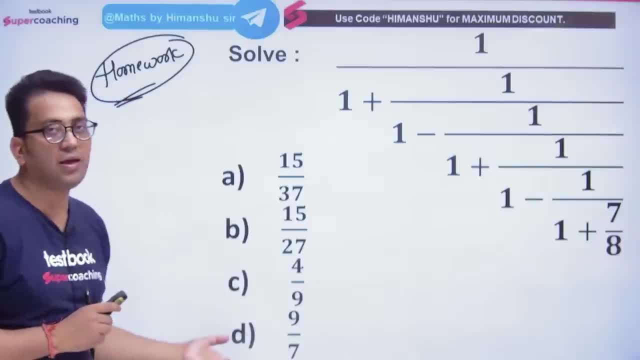 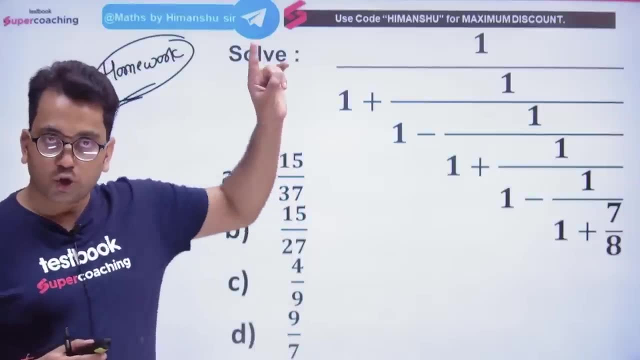 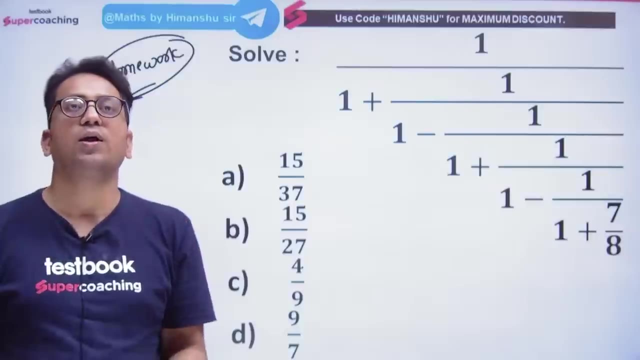 If you are able to understand things, then you answer. You tell me what the answer is, Then I will know. Yes, the child understood the session. He answered the homework question that I gave him. Please do answer in the comment section of all of you. 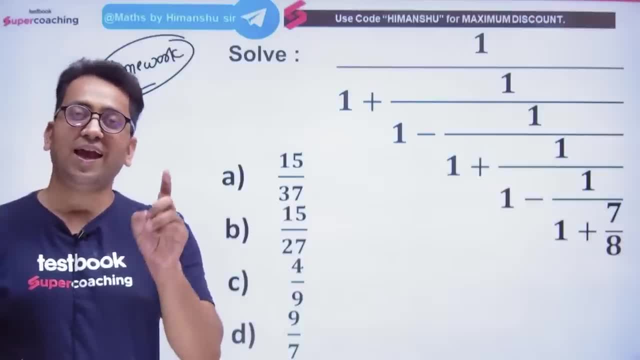 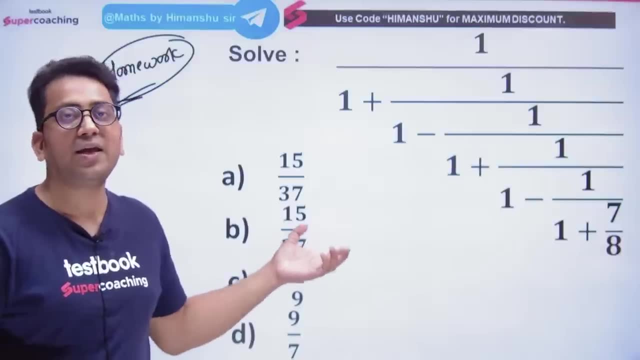 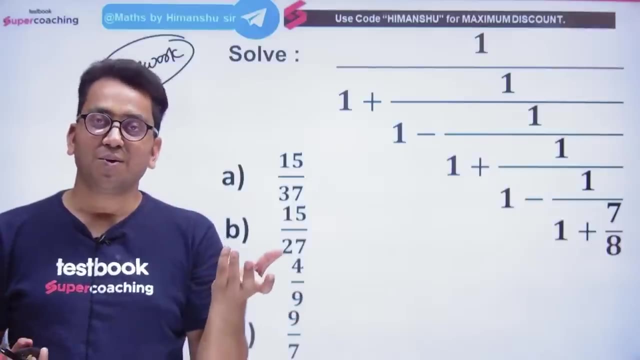 Okay, And write in the comment section that I love my Bihar. Okay, And if you love your Himanshu sir, you like the method of teaching math, then you can give me love with that lovely smiley heart. Okay, That's all you want from him and nothing else. 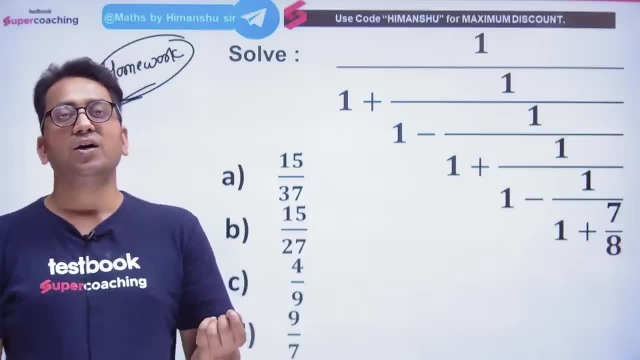 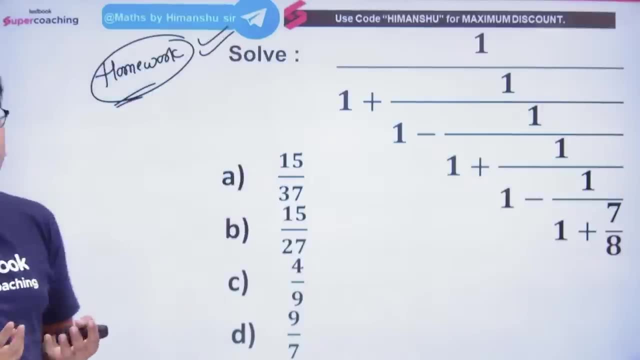 So the children who are here, please subscribe to this channel So that you get the notification of upcoming videos And Maths by Himanshu. sir, this is a telegram channel. Connect with all of you through this telegram channel. Along with that, all the children who are preparing for Bihar, Shikshak Bharti, here. 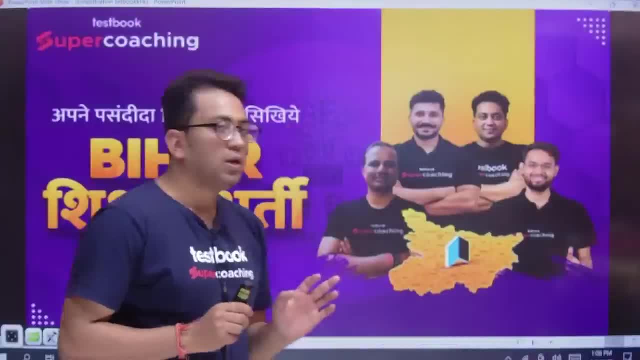 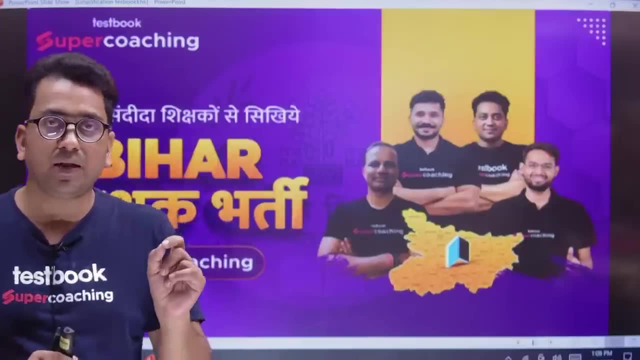 then on Super Coaching Bihar, Shikshak Bharti, 7th Phase batch is available for you here. You can go and join here Till the date of the exam. you will have this batch. Okay, I will also tell you how to enroll the batch. 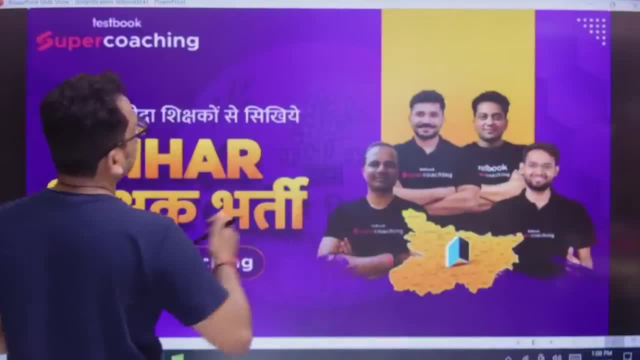 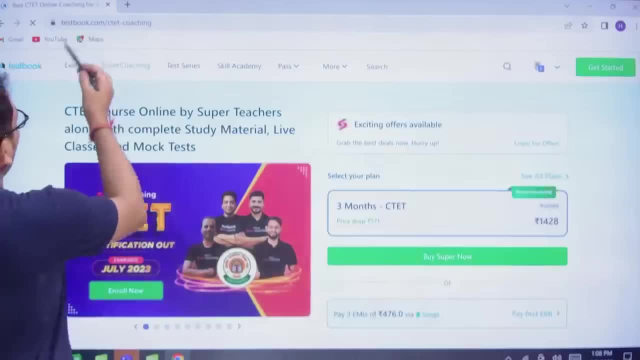 Okay, What you have to do here, please see here. Okay, So you have to go here on Testbookcom And after going to Testbookcom you will go to Super Coaching. On Super Coaching, you will click on Teaching Exam here. 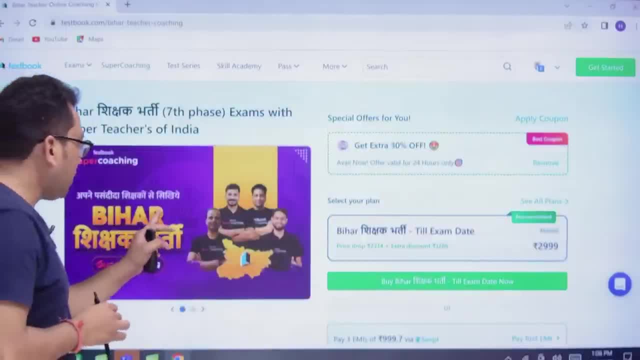 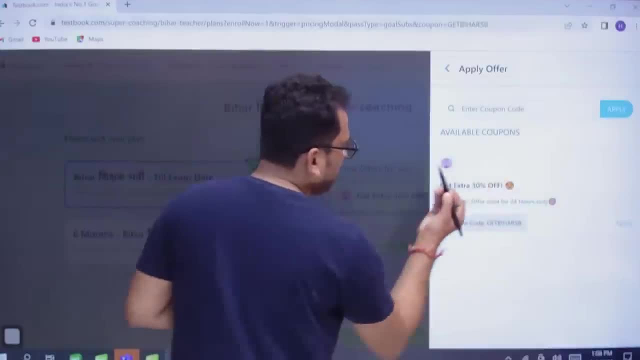 Second, you will see Bihar Shikshak Bharti. As soon as you look at this banner, you will see Till Exam Date, Right. You have to click on this banner. And after clicking on the banner, you have to go to the Apply Coupon section.